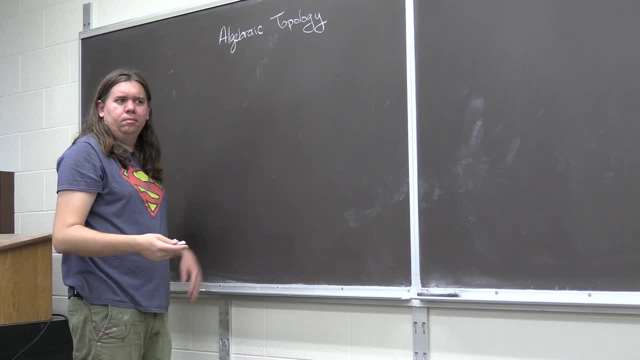 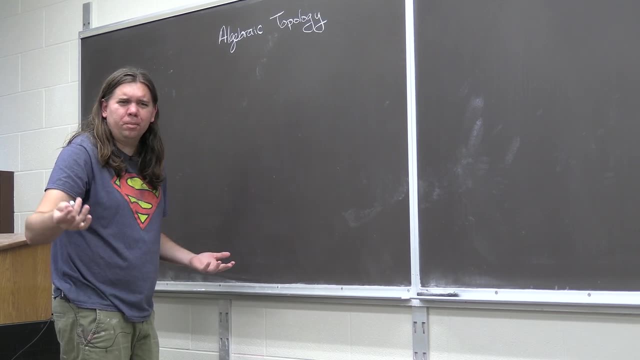 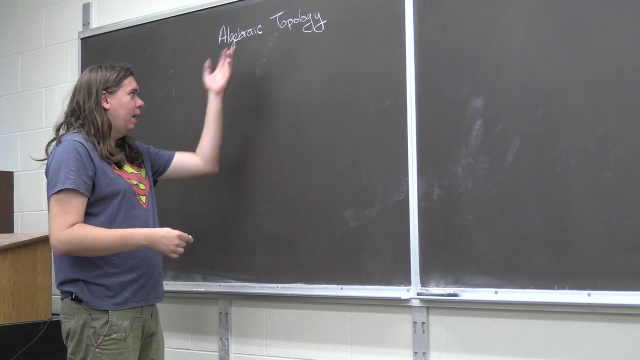 Arabic named after the inventor of algebra, under variable or something. The word for variable, the word for unknown, the way. anyway, this isn't a linguistics class, algebraic topology. So what is algebraic topology? Uh, the way we can think about it is within mathematics. 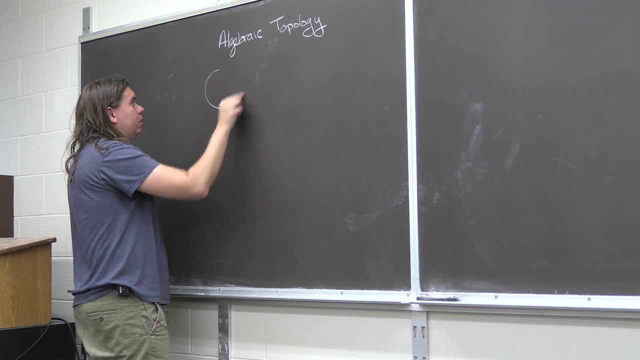 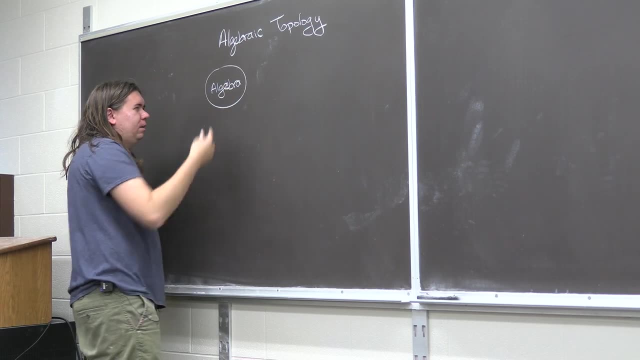 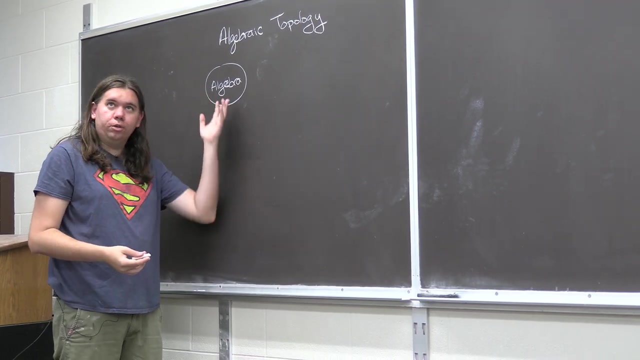 You have different islands of knowledge And over here we have the algebra algebra island of knowledge, where here you have things like group theory And some of you have taken some abstract algebra before you would have learned tools about groups, rings, all of this You learn about that in algebra land. 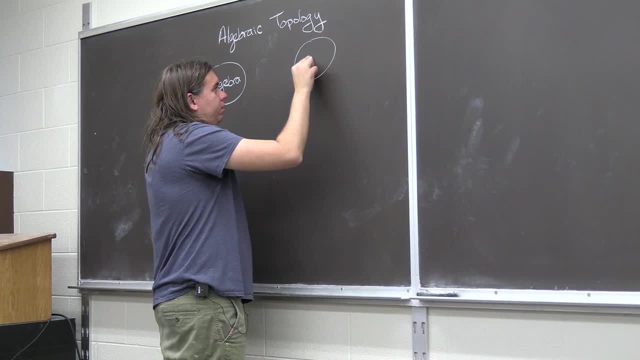 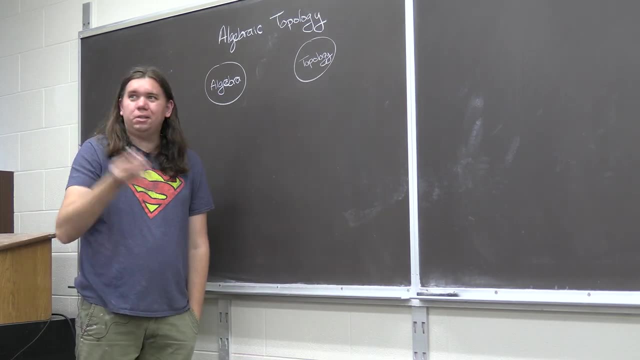 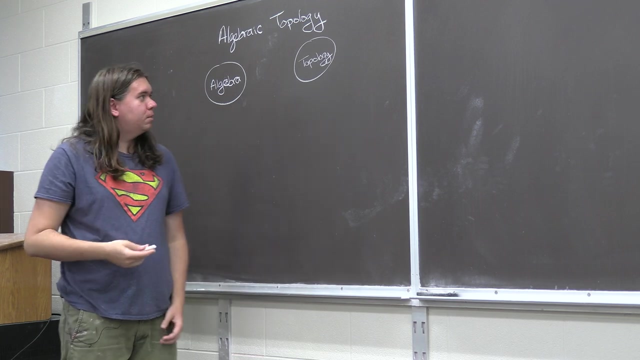 Over here we have the island of topology, And topology is interested in the study of shapes and surfaces. loosely It's like geometry, but a little bit under the influence, And so you're a little bit loose in how we handle things. What algebraic topology is is it's a bridge between these two lands. 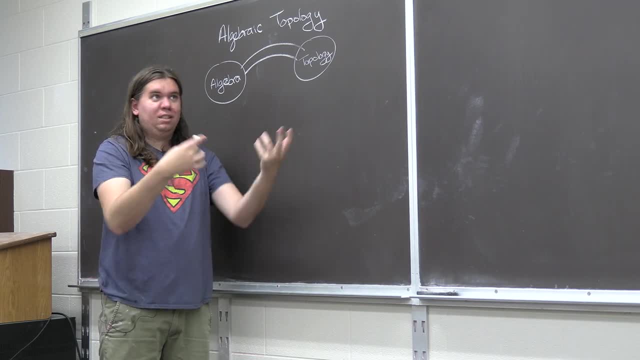 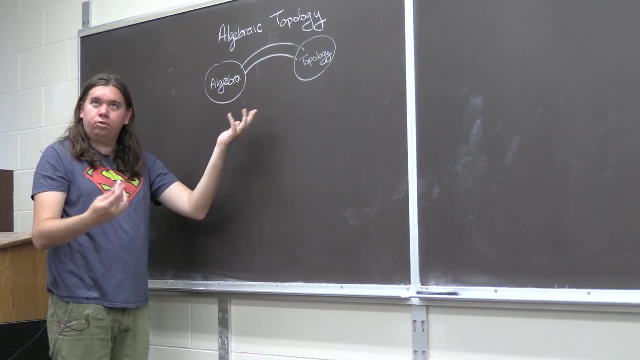 It takes some shape or surface, something that's kind of hard to grasp, something that's kind of loose, and transports it to the land of algebra. It assigns it some algebraic structure. Now, in the land of algebra, we can work with the structure. 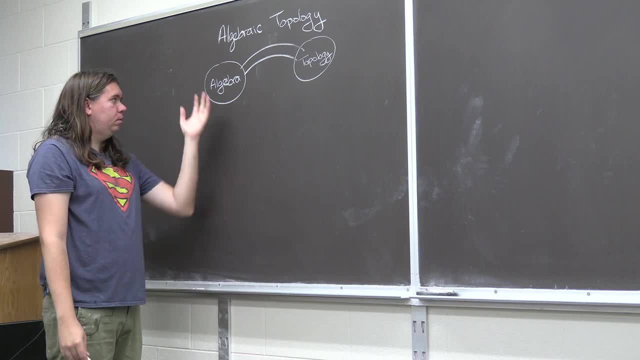 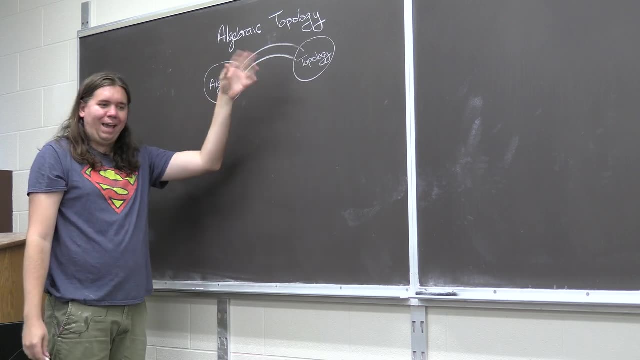 We can do nice clean mathematics and the base, whatever we discover in the land of algebra is giving us some insight to this topological structure. So you can think algebra is the way we're going to handle on the topology. So that's the big idea of algebraic topology. 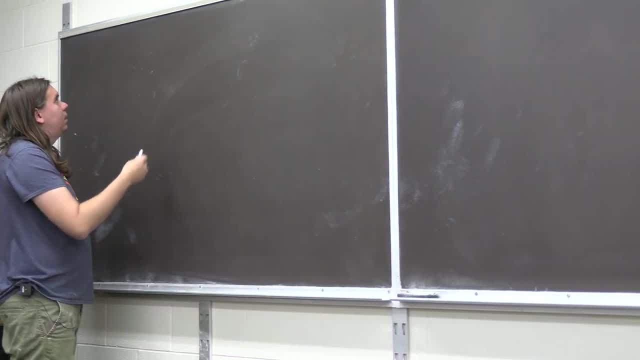 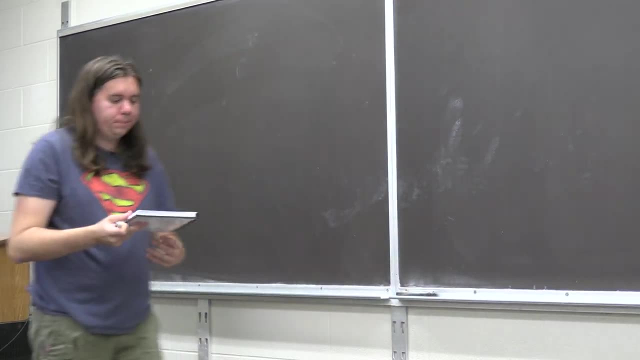 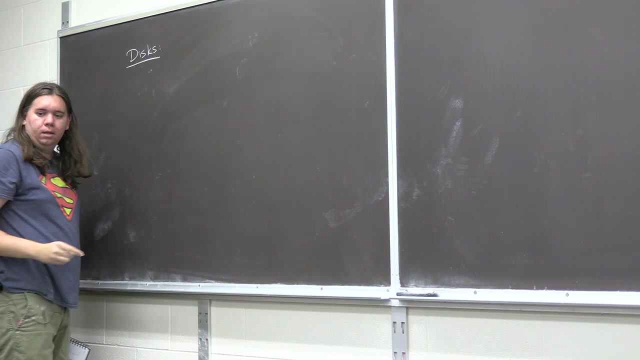 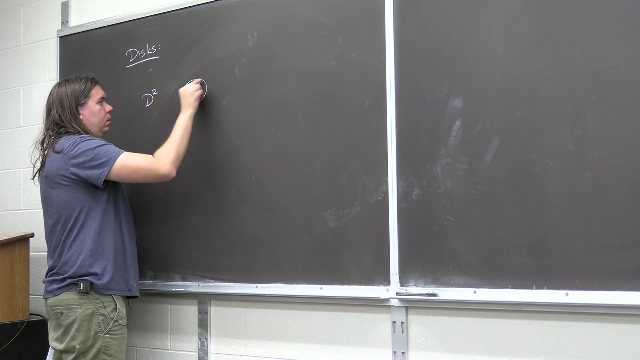 So today I would like to begin by introducing us to just some basic algebraic shapes, some basic notation we'll be using throughout the course, And the first object I'll introduce us to are a disc. So here's my notation: When I write D2, I just mean the two dimensional disc. 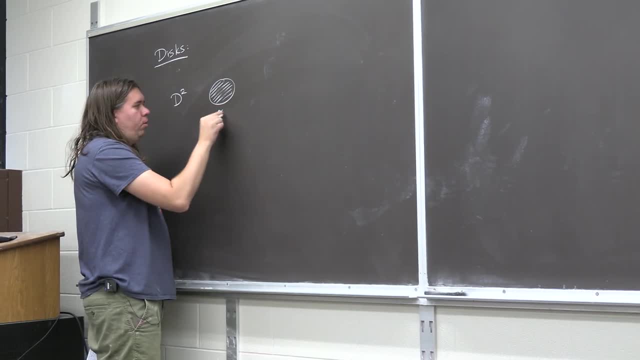 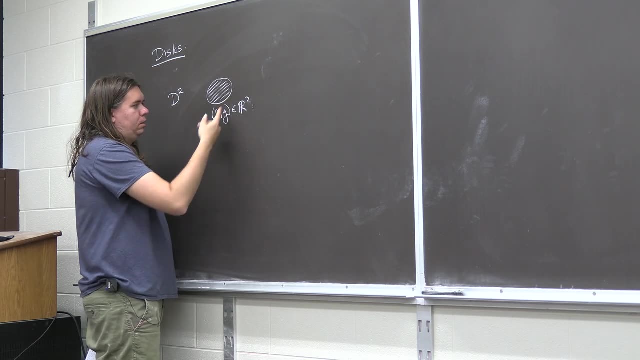 And so you might think of this as something like the set of all points: X, Y and R, Y and Z. So I'm going to write R2, such that the distance from the origin is less than or equal to one. 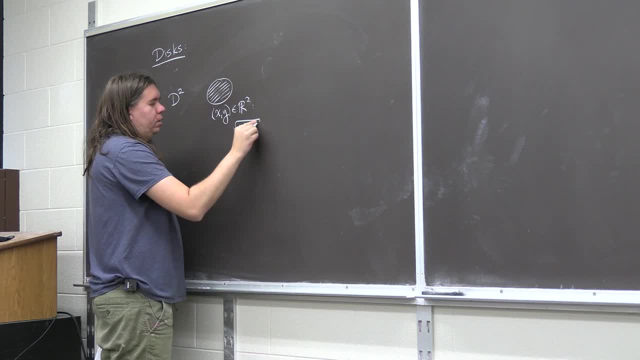 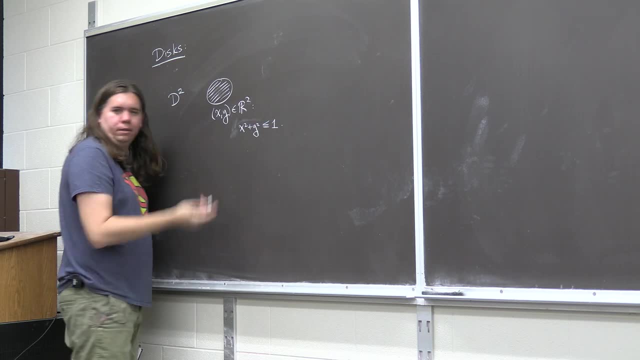 say such that the square root of X squared plus Y squared is less than or equal to one. Well, we don't need the square root, because the square root of one is just one. So X squared plus Y squared should be less than or equal to one. 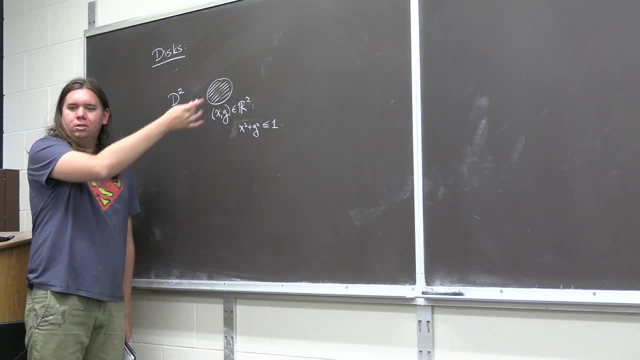 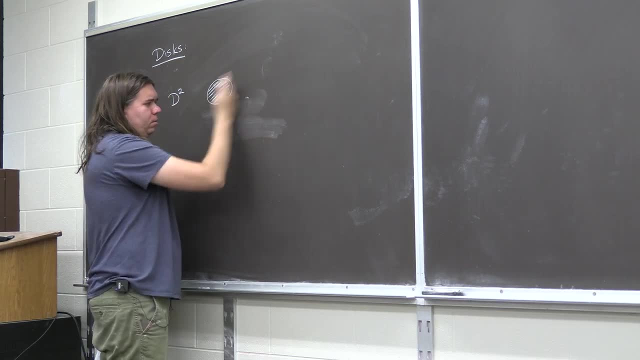 This is how you can think about a disc. But this definition is not so important because for us we're not going to really have this strict. you know, in the zoom we know metric that we're dealing with here, So we don't need a definition like this. 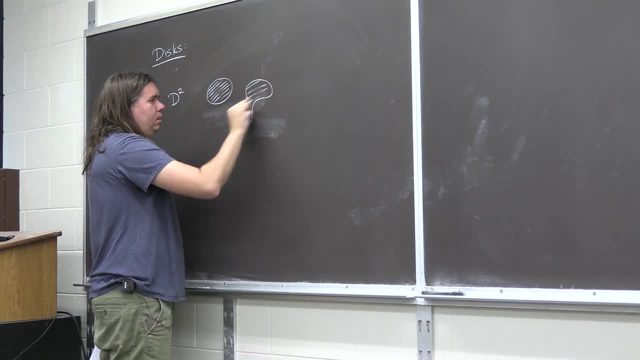 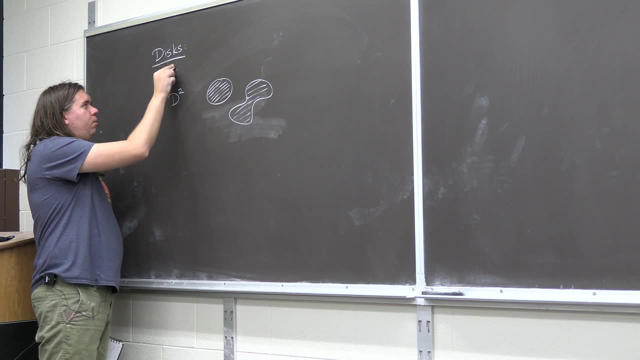 This is a disc. Sometimes I'll draw my disc like this instead. These are all discs, right? Okay? Idea is: D2 is just two dimensional. How about D1?? Can you give me any guesses of what D1 should be? 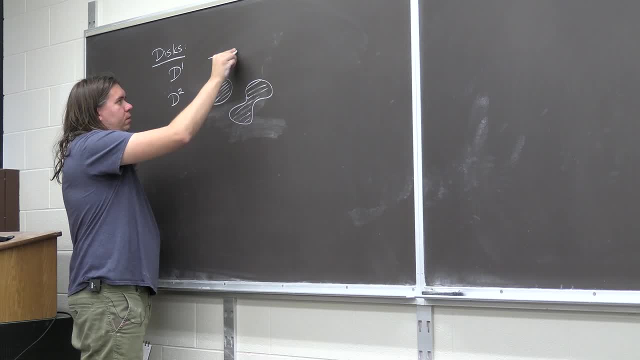 Just a line, So you might think it's the points of length up to one in the R1. But just think of it as a line segment. right, And sometimes I'll stretch and bend my line segments, I don't care. 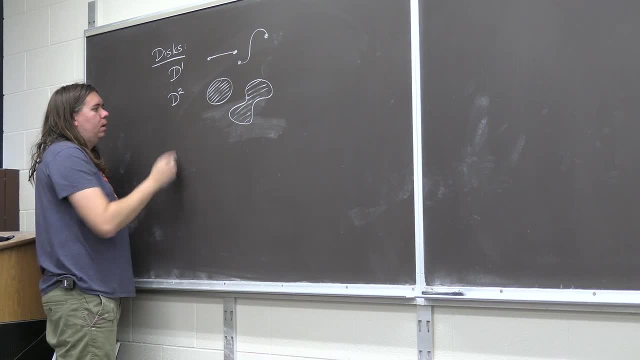 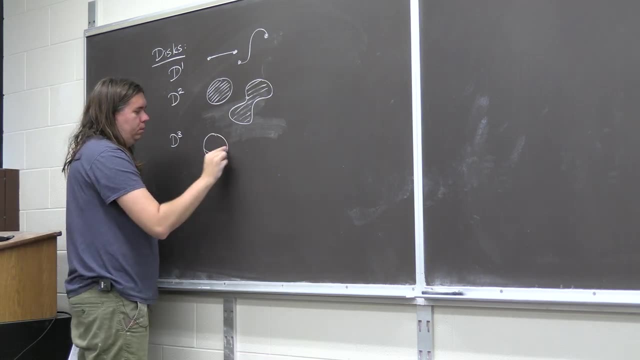 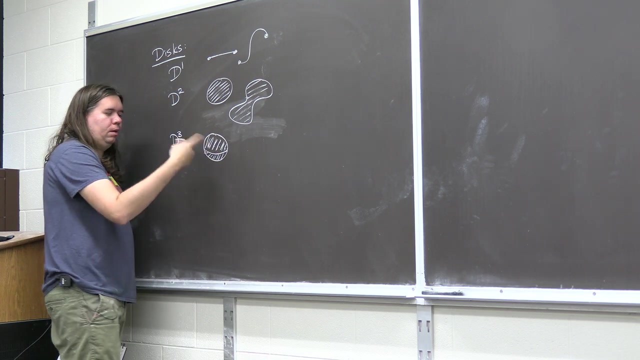 This is D1.. These are all D1.. How about D3?? Yeah, a ball, a solid ball, Right, And you might deform it to be a slightly different shape, but anything equivalent to this. I'll make more sense of what we mean by equivalent in the next lecture, and so forth, for 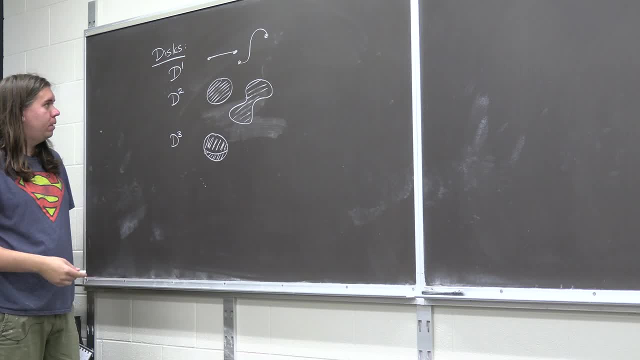 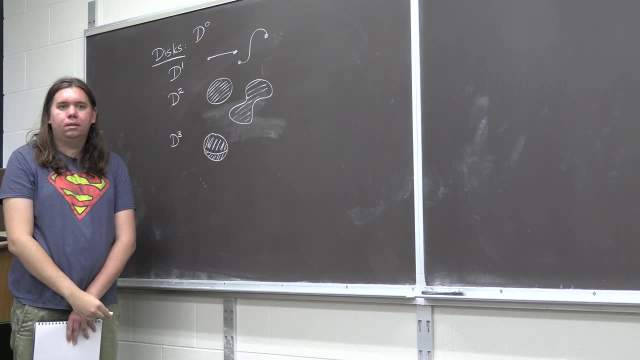 higher dimensions. right, You can go all the way up to DN. Well, N is whatever dimension you like. We can also go lower D0.. Help me out. What should D0 be? Just a point, Just a point. 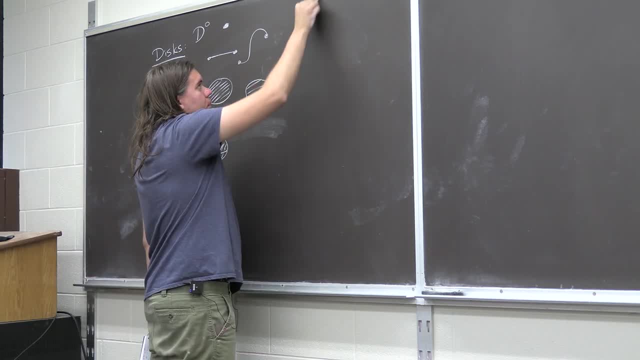 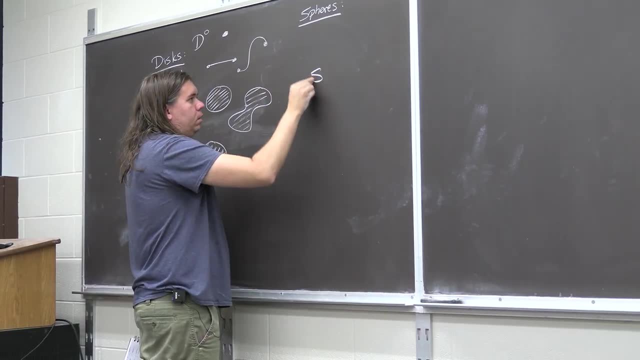 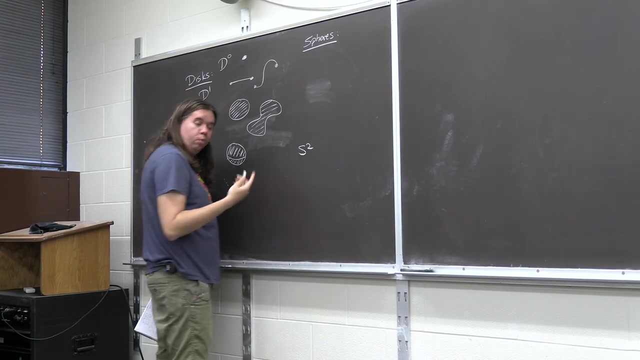 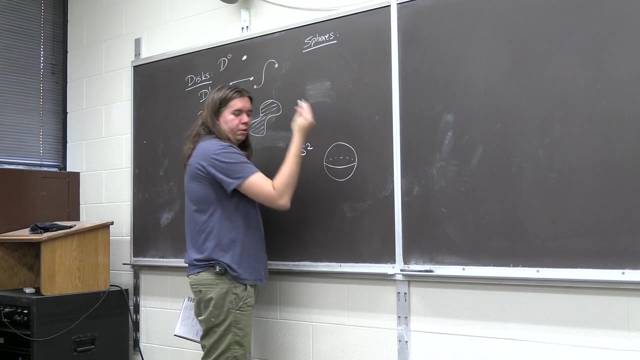 Those are discs. We also have spheres. S2 is I should draw down here. S2 is the two dimensional sphere, but the two dimensional sphere you think of as living typically in three dimensional space. You can live in higher spaces too, but you typically think of it as three dimensional. 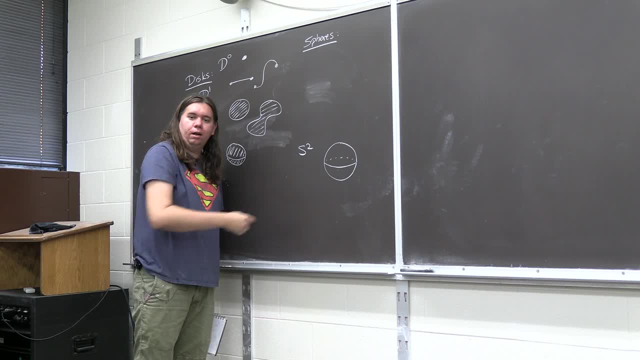 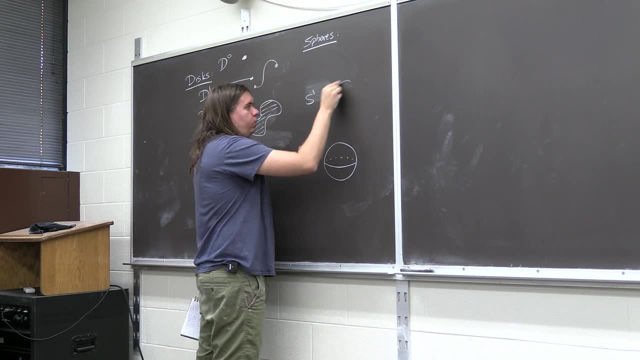 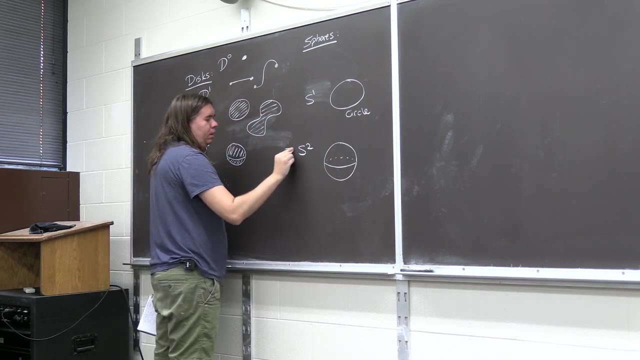 space. So this is just the boundary of the ball. Likewise, S1 is the one dimensional sphere which we often refer to as the circle Right. So S2 is the boundary, The boundary of D3, this is my notation for boundary. 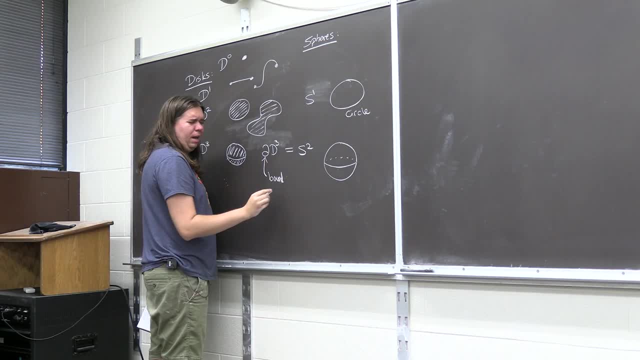 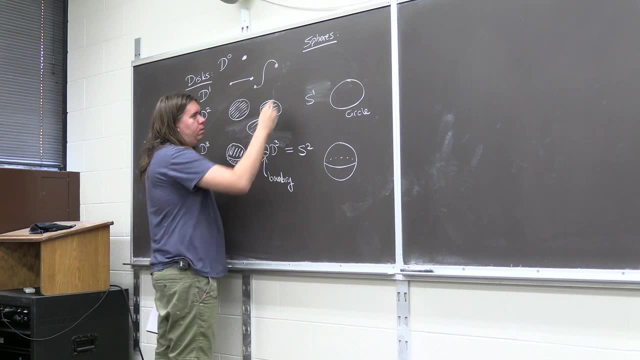 Is there an A in boundary? There's like half the alphabet in that word. The boundary of D3 is S2.. The boundary of B2 is S1.. So you help me out now. What should S0 be? Well, if we think of S0 as being the boundary of D1.. 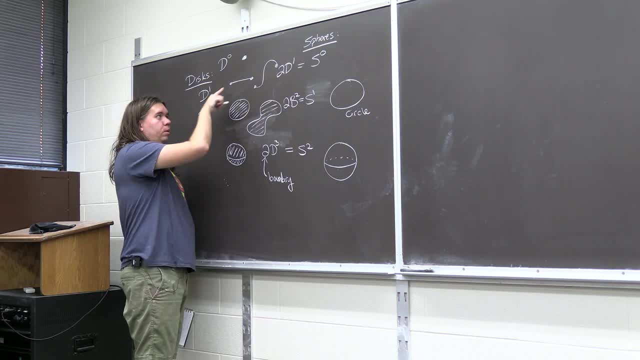 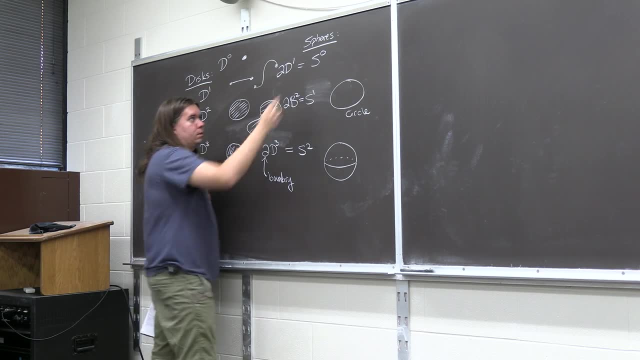 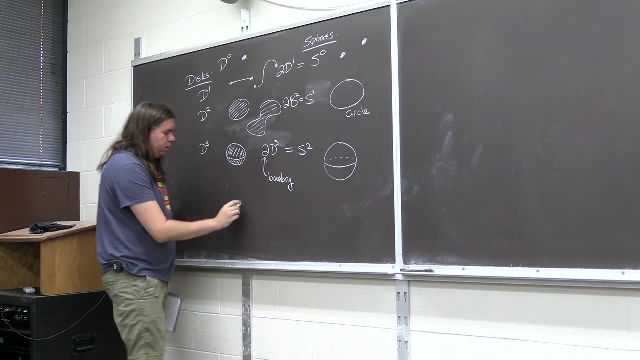 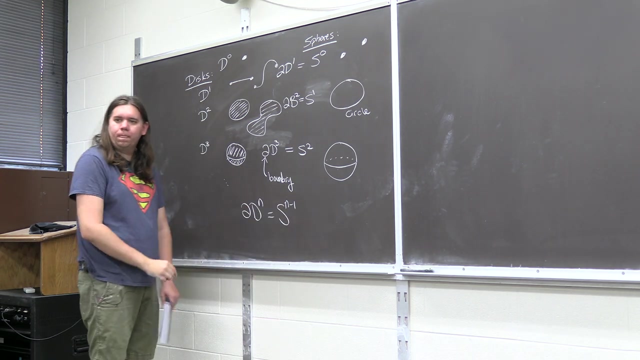 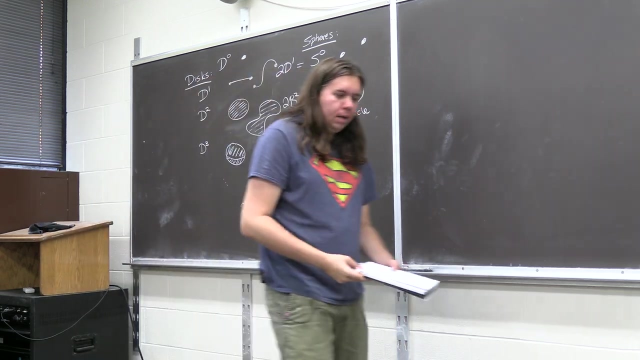 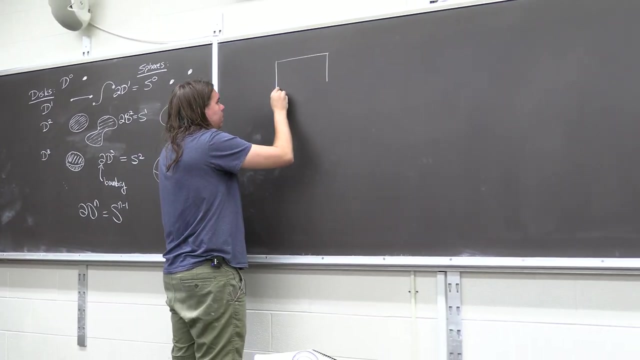 boundary of the one-dimensional disk, which is just the unit interval or just an interval. what would S zero be? Two points. S zero is two points And in general, the boundary of the n-dimensional disk is the n minus one dimensional sphere. Happy, Okay, There are other surfaces. Here's a classic one. 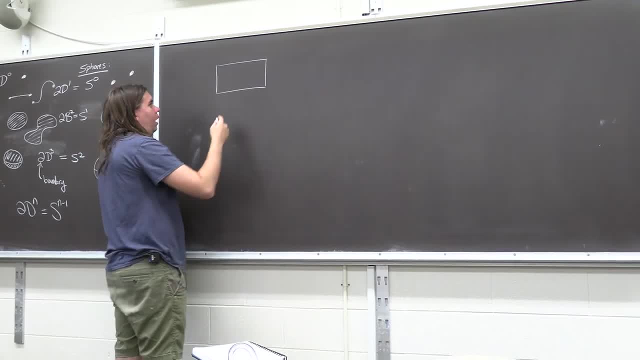 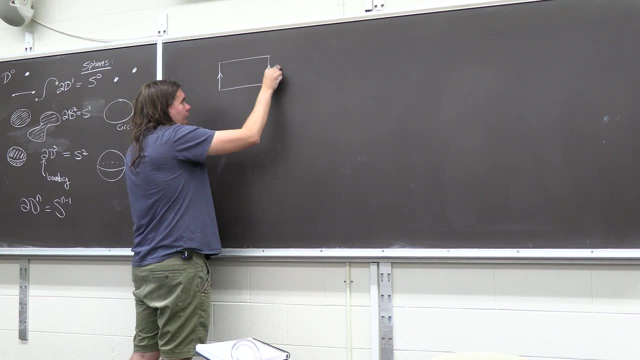 You might take a square and glue together the right side with the left side. I'm going to label this A and A just to indicate I'm gluing this side to the right, And I'm going to label this A and A just to indicate I'm gluing this side to the. 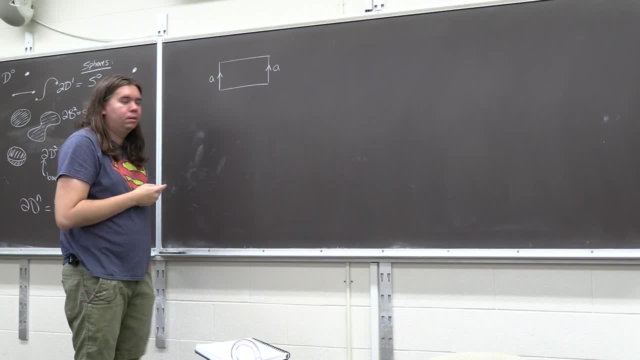 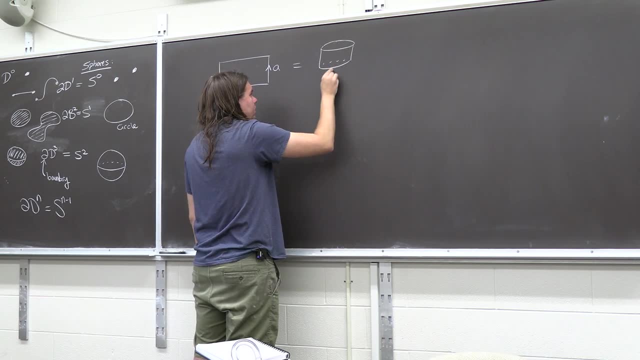 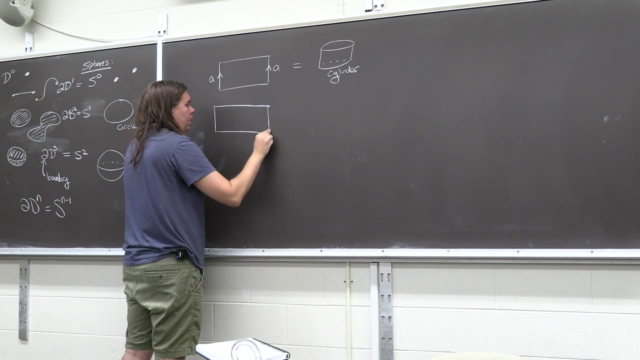 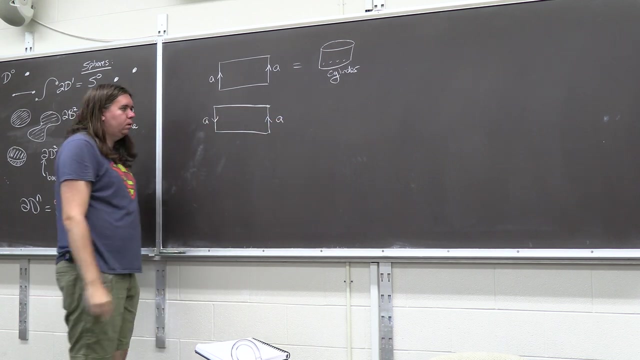 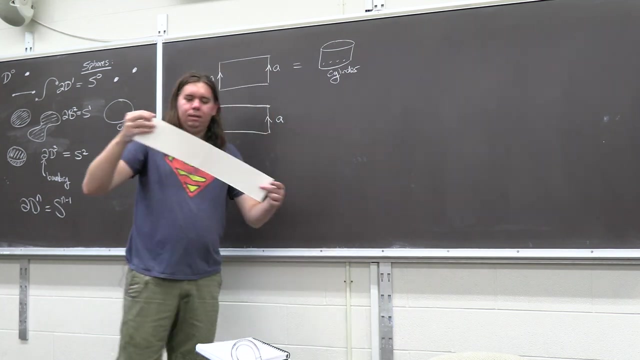 side. What do you get? Yes, we get. this is my way of representing the cylinder. If, instead, I glue the left to the right, but with opposite, flipping the orientation of one of them, what do we get now? Yeah, this is the classic. take a strip, glue together the sides. that's the cylinder. 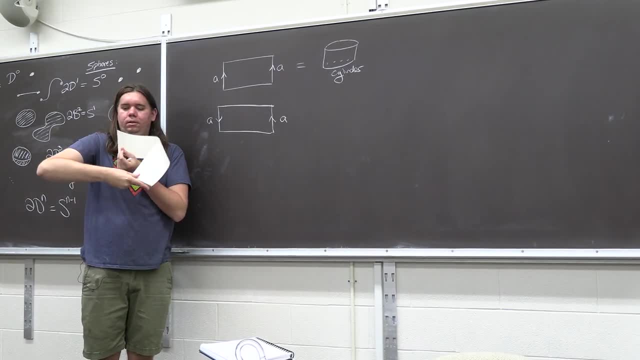 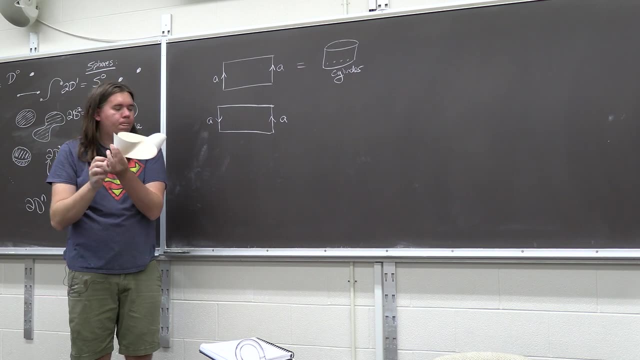 but now we're not going to glue them together the same direction. We're going to flip one over and glue them together And we get this one-sided shape called the Mobius band. So it ends up looking: a little twist gets added. 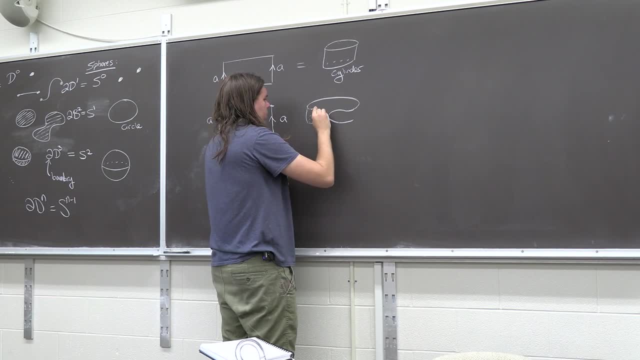 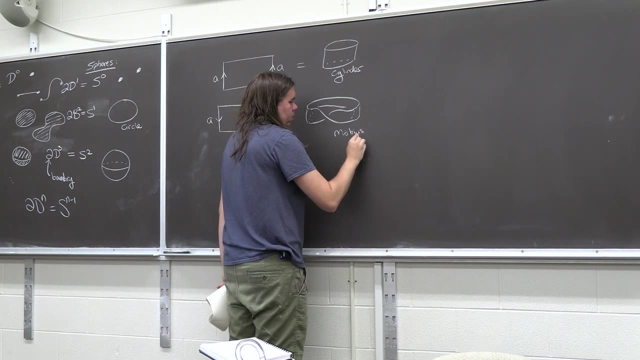 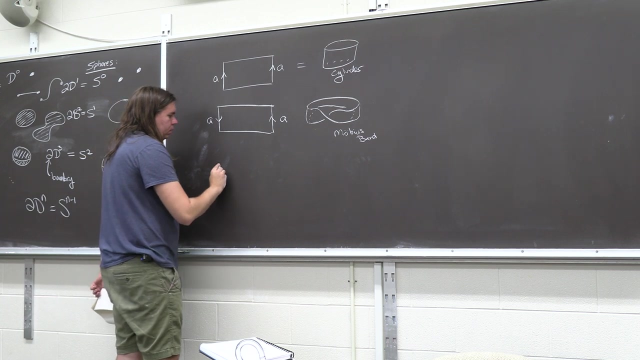 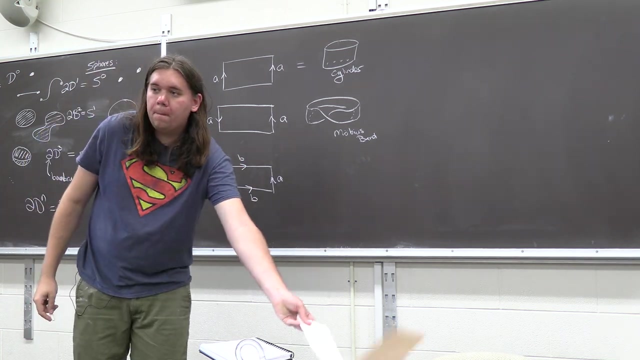 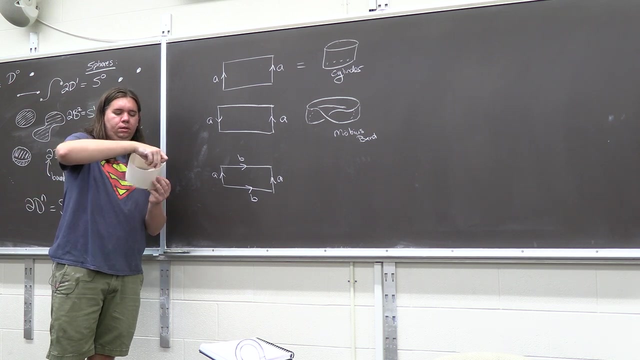 And we get the Mobius band, Mobius band or Mobius strip. Here's one more. Take a rectangle, glue the left to the right. glue the top to the bottom. this is going to be a glue the left to the right. now I want to glue the top to the bottom. what's? 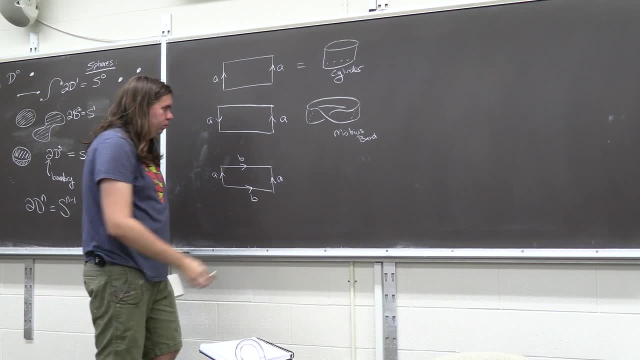 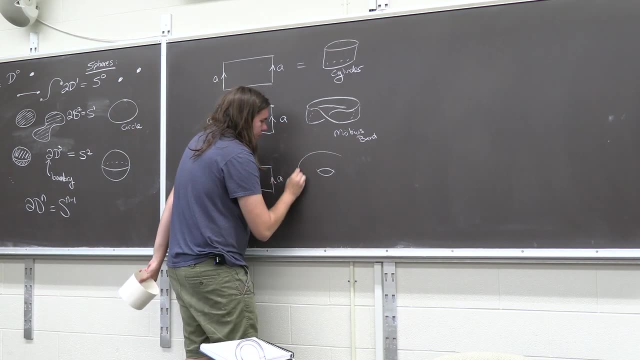 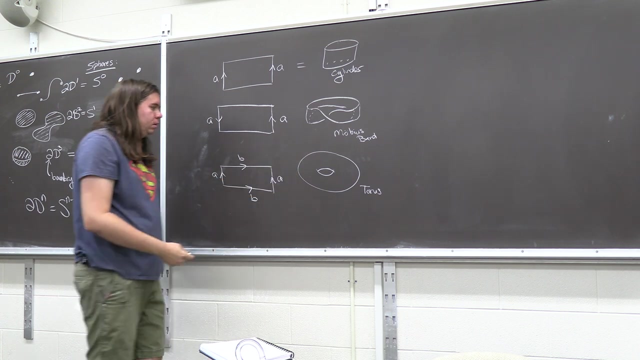 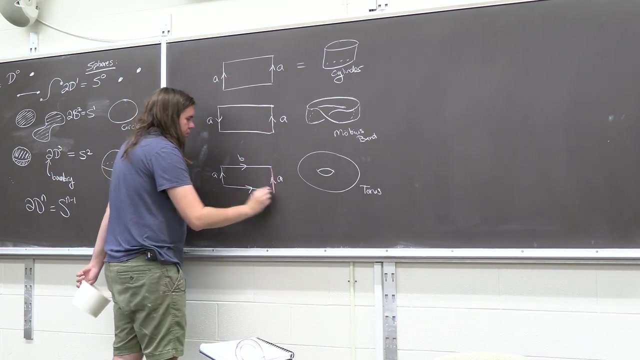 going to happen. if I glue that top to the bottom, we get the surface itself, the torus. not a solid torus, just the surface of the torus. so we, when I say torus, I'm just referring to the surface. it's not filled in, it's just the their surface itself. you can think that this a here got glued. 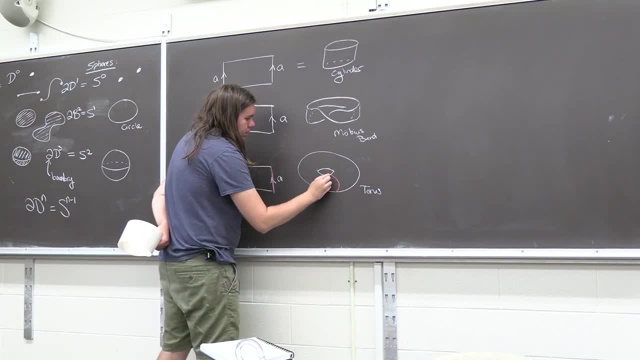 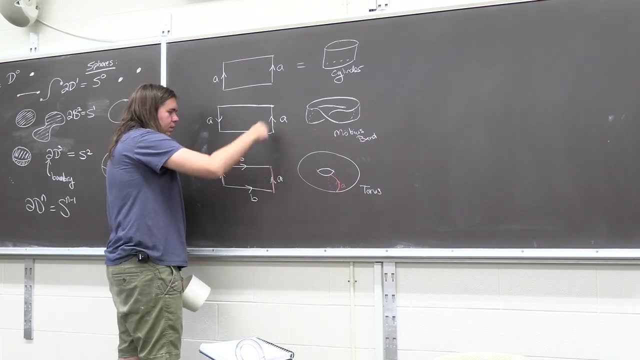 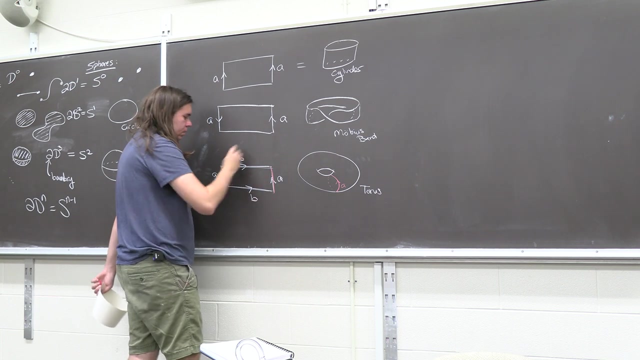 to this a, and when they got glued together, they ended up forming something like this circle. it's a circle because you also glue the top to the bottom, making it a circle, and here this B gets glued to this B, which then gives you a circle going around the other direction. 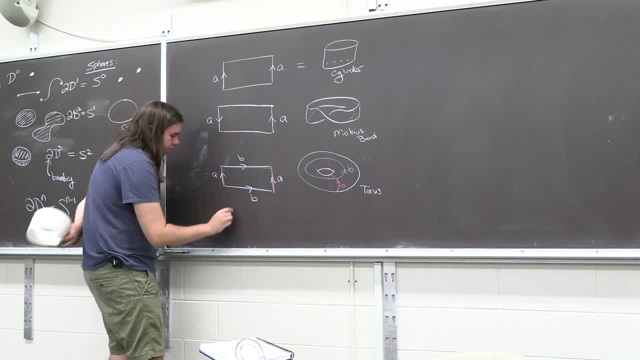 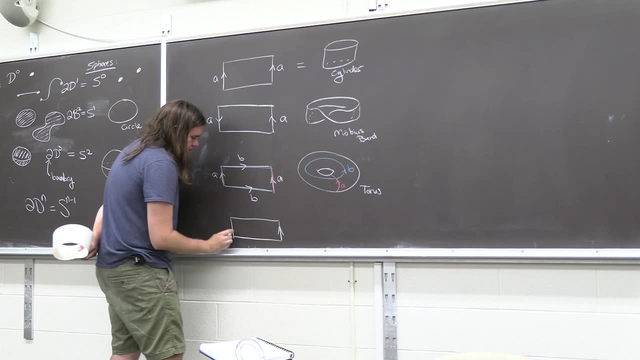 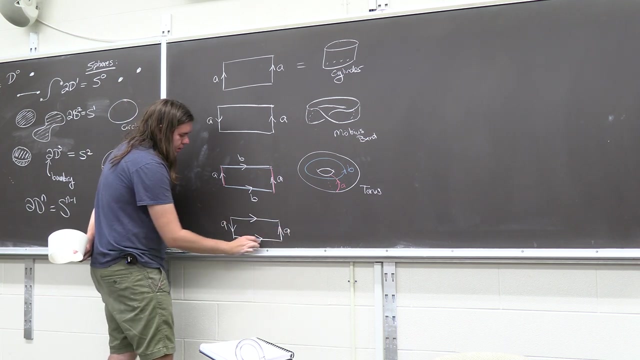 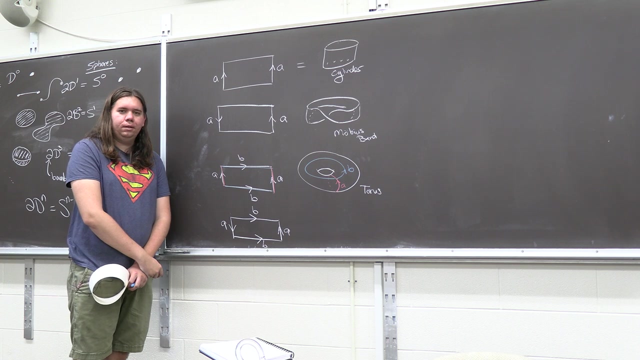 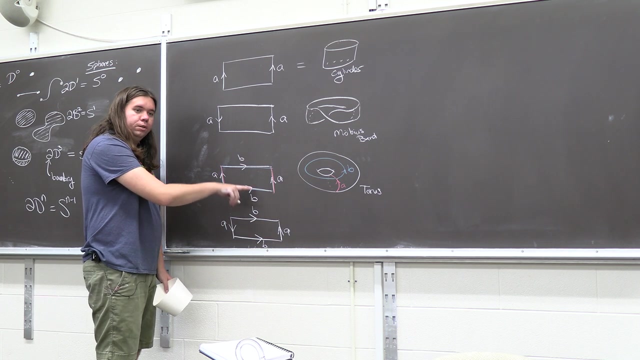 okay, one last one. we're going to do the same thing, but I'm going to flip one of the directions. so a with a, B with B, but I flip one of the orientations. what am I going to get now? yeah, so the way you can think about it is, if you glue that B with B, you get a cylinder. 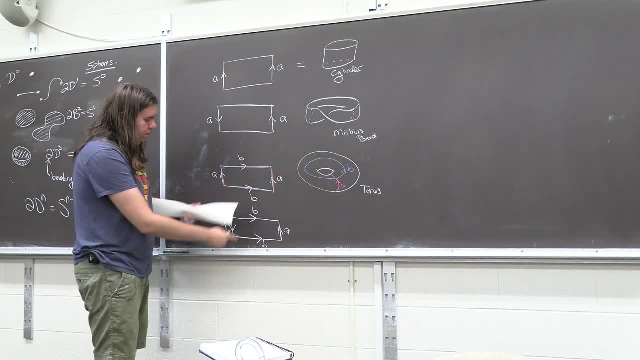 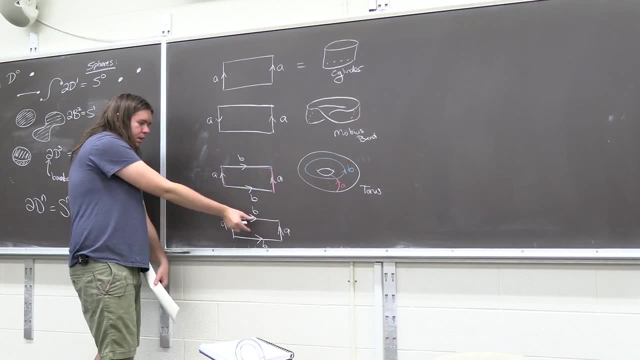 so now I have a nice long cylinder. if I'm gluing that B to B, I want to attach the A to the A, but I can't attach it around this side because the opposite orientation, so I have to attach it by bringing in. so what you get is you get some cylinder. 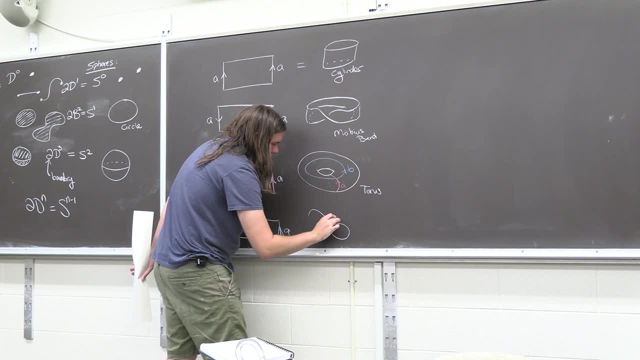 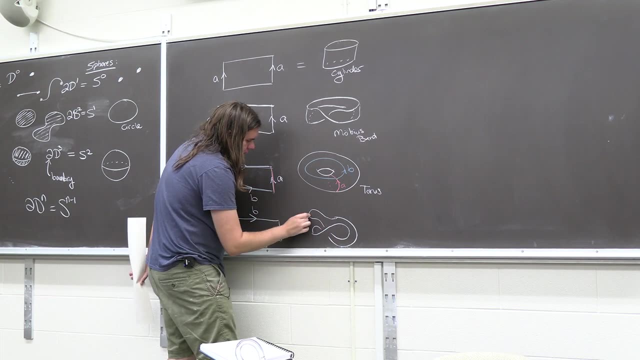 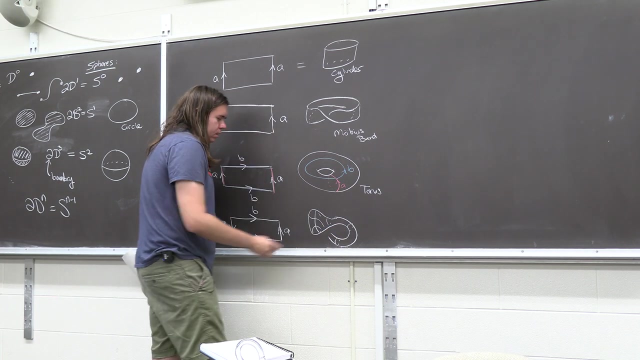 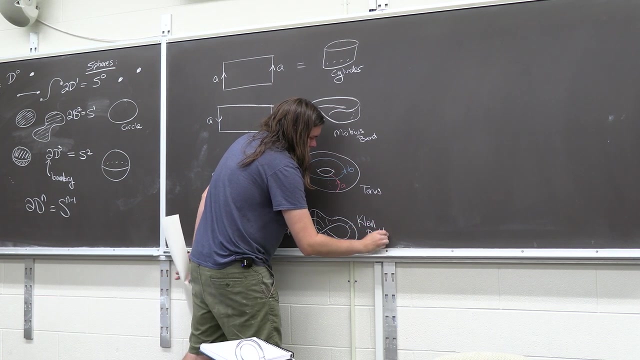 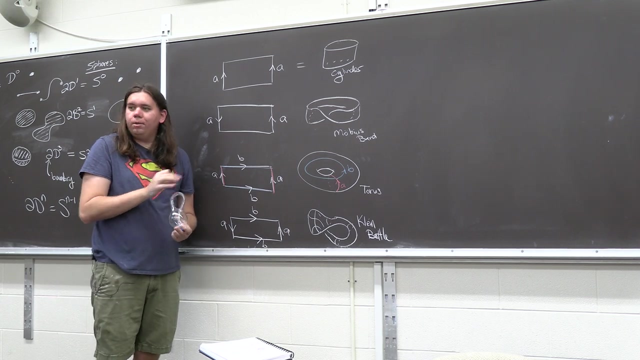 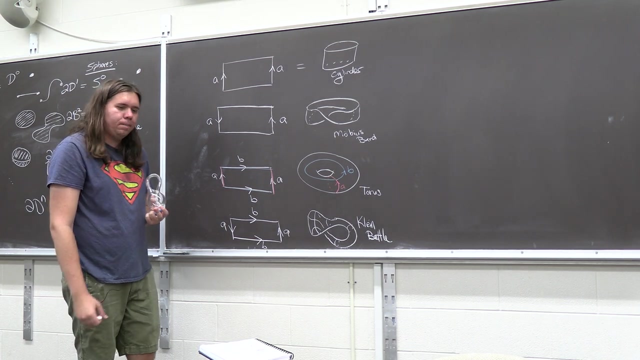 but then this part needs to attach back down to the base, not by coming around, but by coming inside and attaching to the base. and so you end up with my attempt to draw on a Klein bottle, which you can see right here, the Klein bottle. okay, are we happy with this way of drawing things? okay, well, let's try and step it up a level. 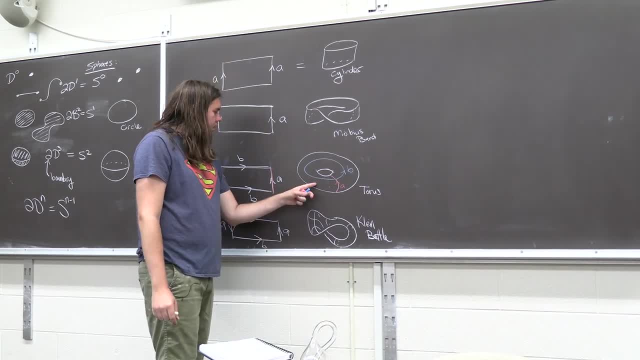 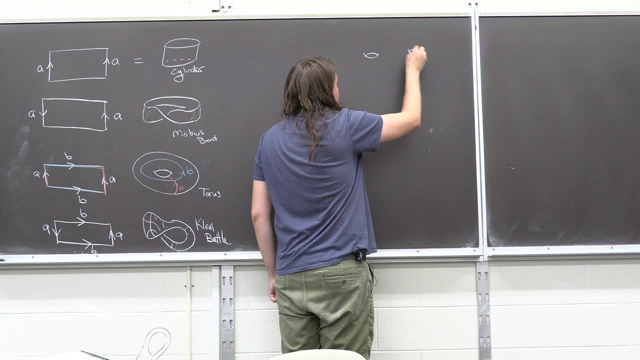 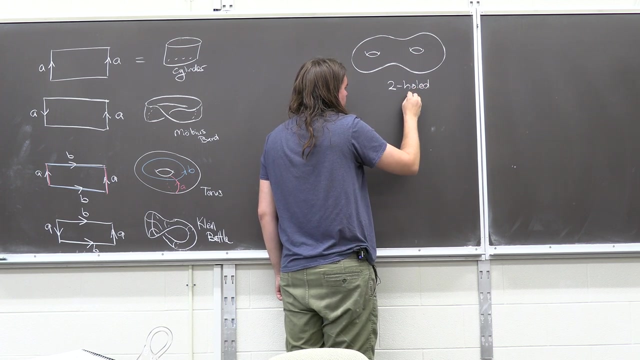 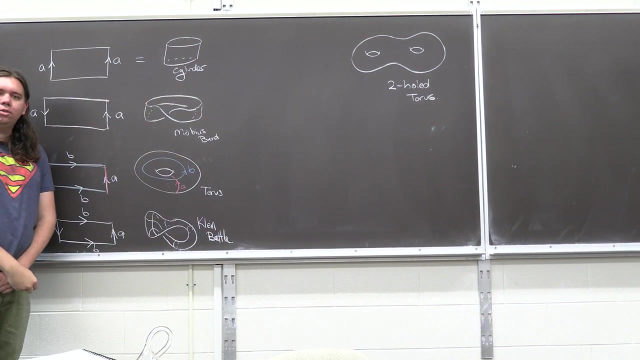 what if, instead of drawing a torus, I want to give gluing instructions to draw a torus that has two holes in it? so this is my two-hole torus, genus two, if you've heard that were genus before. this is my two-hole Taurus. what set of gluing instructions will give me a two-hole Taurus? 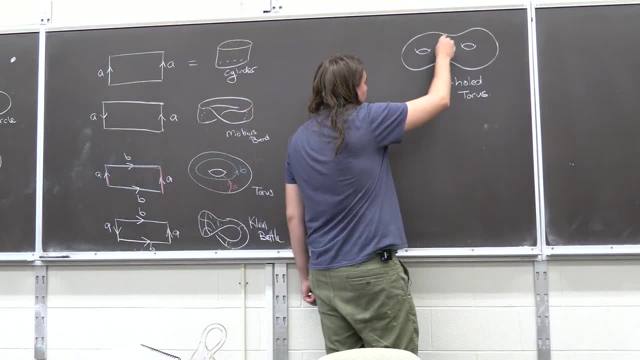 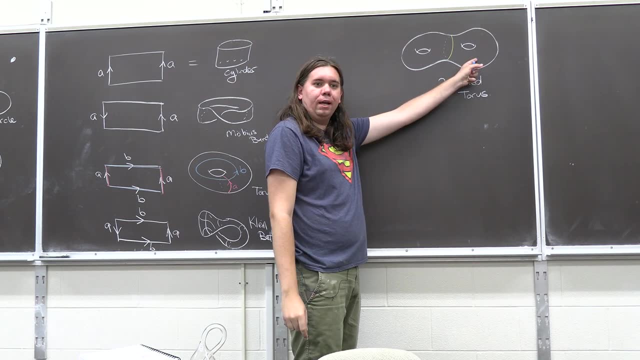 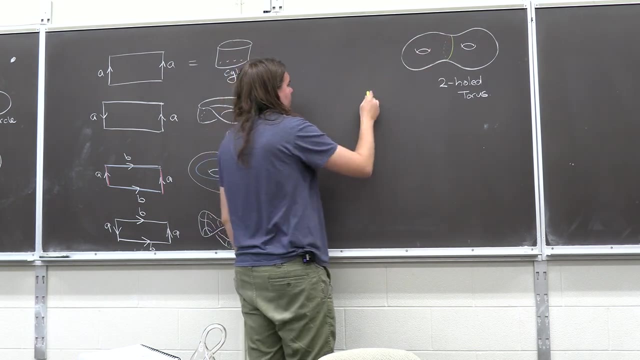 the way we can think about this is: I'm going to cut this two-hole Taurus in half. let's first figure out how to just glue this right hand side. this right hand side is a Taurus that someone took a bite out of right, so the right hand side is just a Taurus. 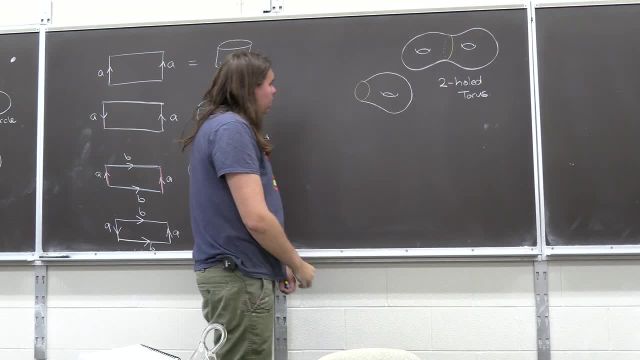 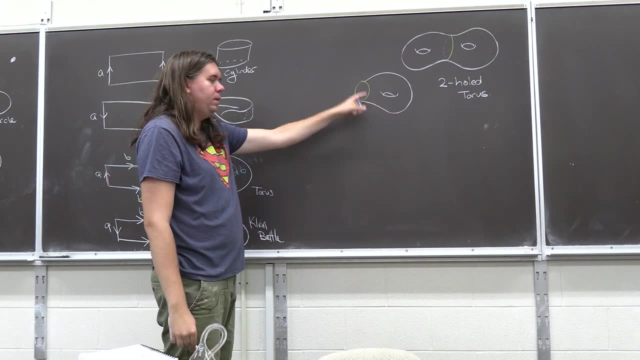 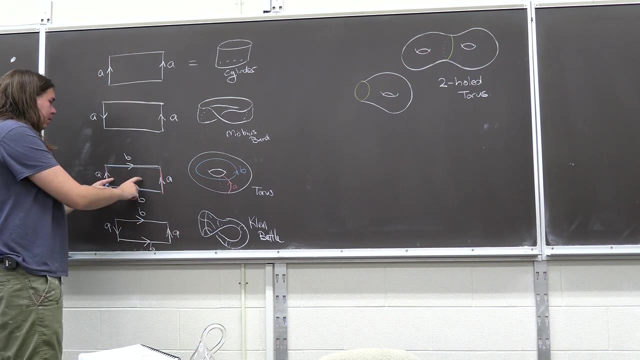 that somebody took a bite out of what set of gluing instructions will give us this. well, this yellow piece should be left over. so this yellow piece is going to be glued to other things. it's going to be left over and see if you can convince yourself. it's exactly the diagram for. 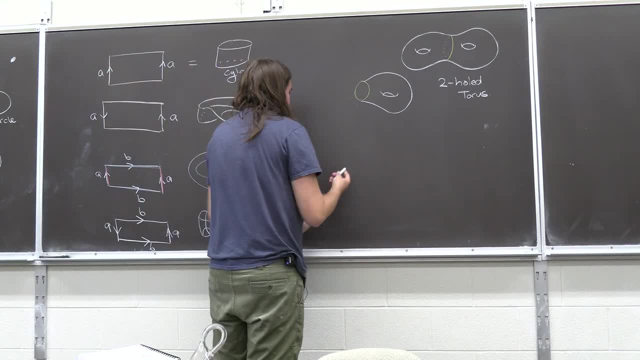 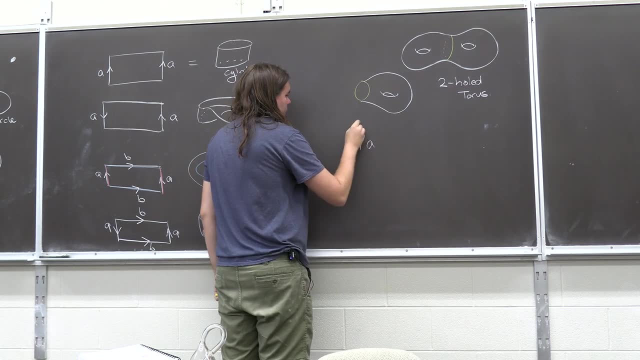 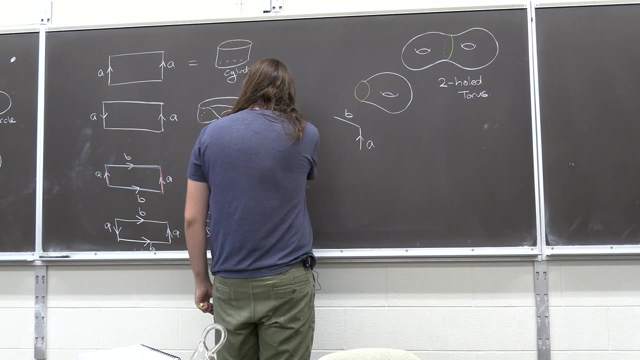 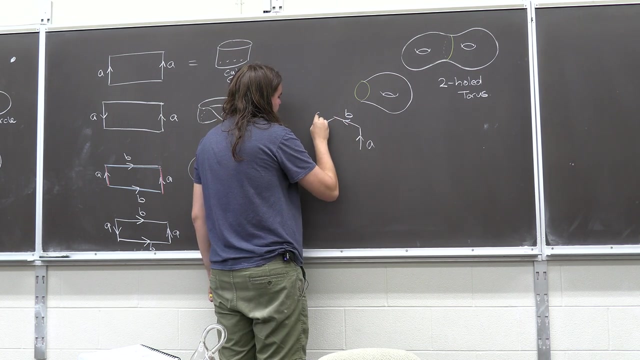 the Taurus except. so let me start drawing the diagram from the Taurus. so you have your um a and then you have your B. okay, we can draw it this way- I'm going to draw it slightly different- and then we have A and then we have. B. if, if I completed this for this hanging balance, let's say I get, the opening is right, I want to end on A. so if I complete this, I'll end on B, and then I'm going to same way. you had this diagram's For Т an. if I complete this, I'm going to shift to right hand side. 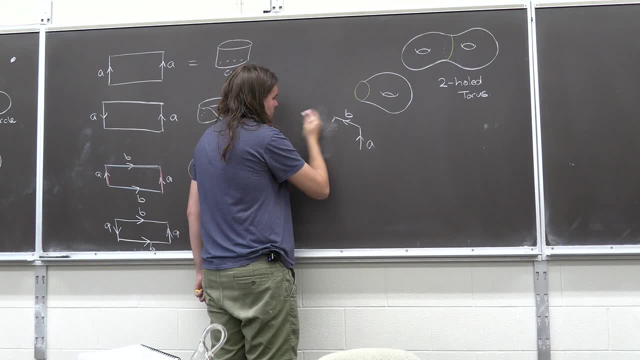 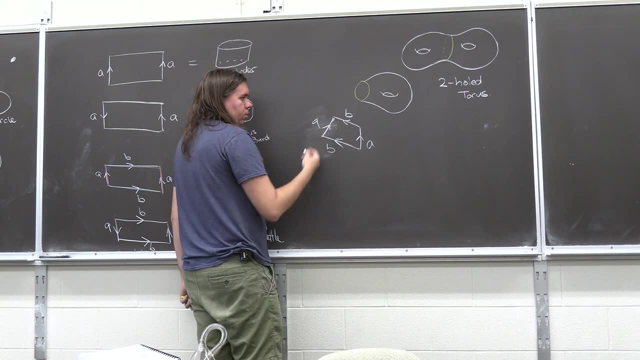 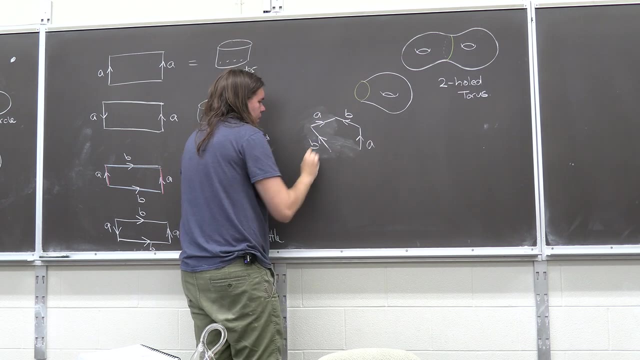 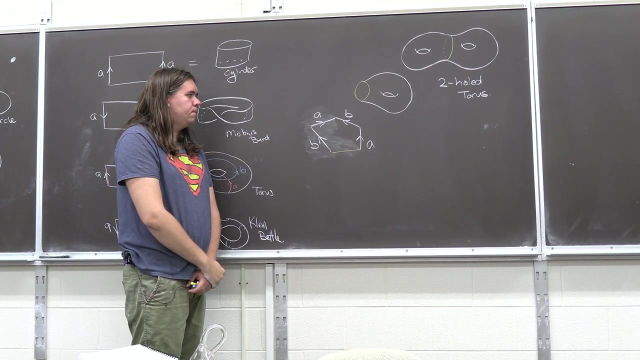 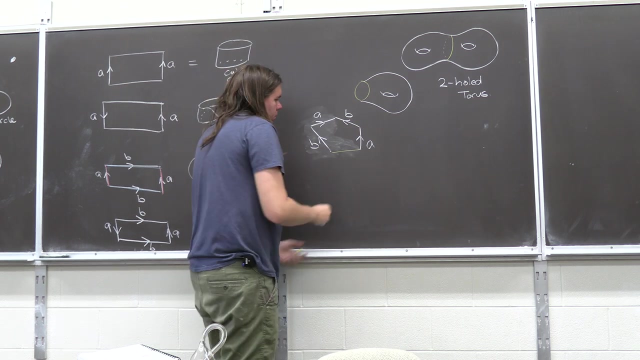 this if I had just drawn AB AV. that's just a torus, right, that's just a torus. what I'm going to do is, before I complete it- a, B, I'm going to stick this line: you, what happens to our lion in the end? well, the bottom of a gets identified with the. 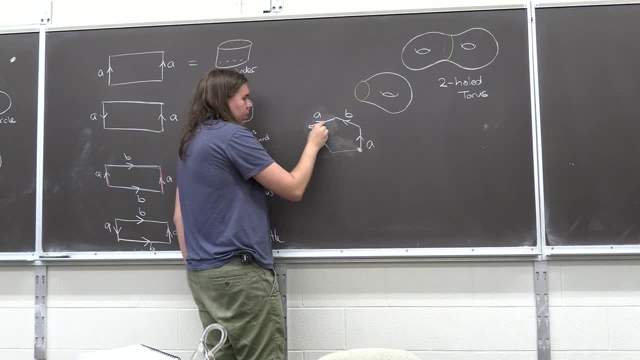 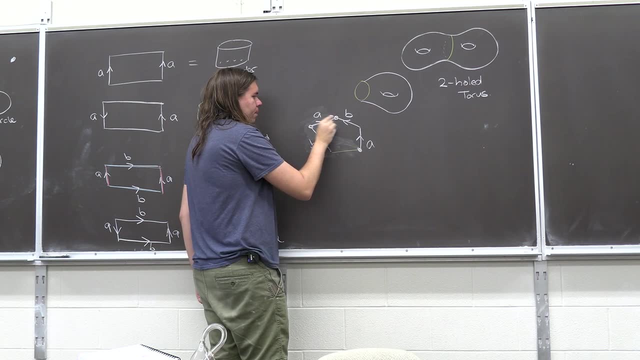 bottom of a. when you glue these together, so 19 at the top of B. so it's identified with the top of B. so it's identified with the top of a, immediately with the bottom of B. so, terrified, the bottom of B. this will get glued together at the. 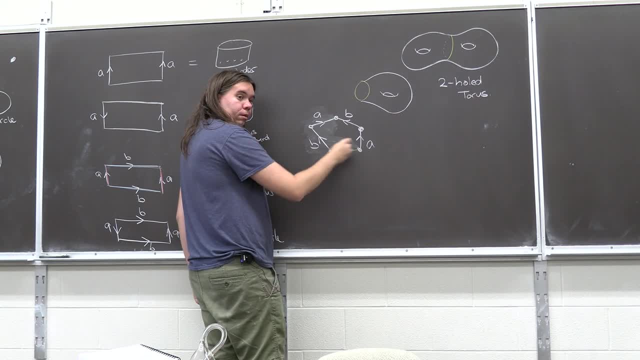 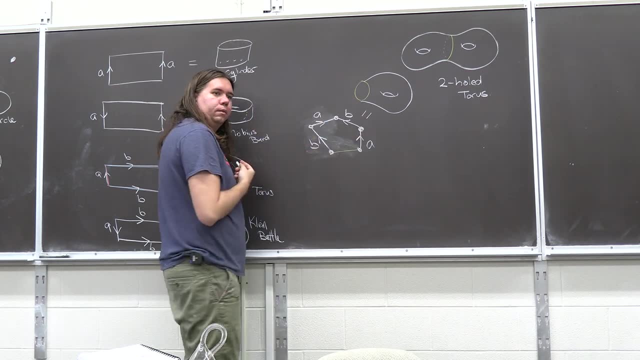 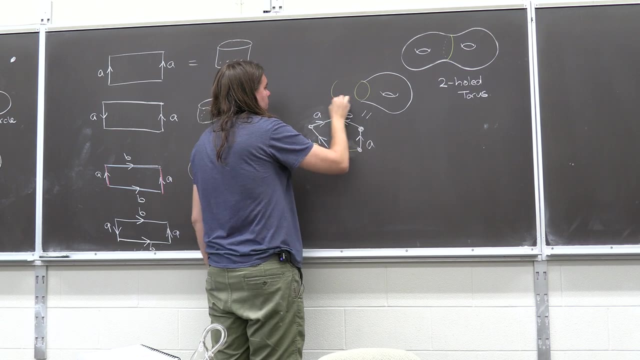 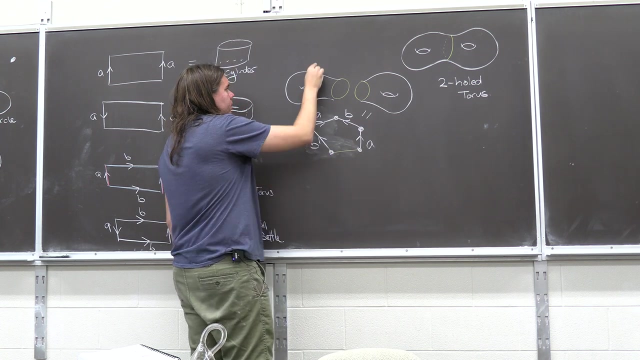 to itself. This will become a circle, and the rest of this folds into a torus. So this is the gluing instructions for the left-hand side. Then, similarly, we can think of the right-hand side as just being another copy of a torus, So another. 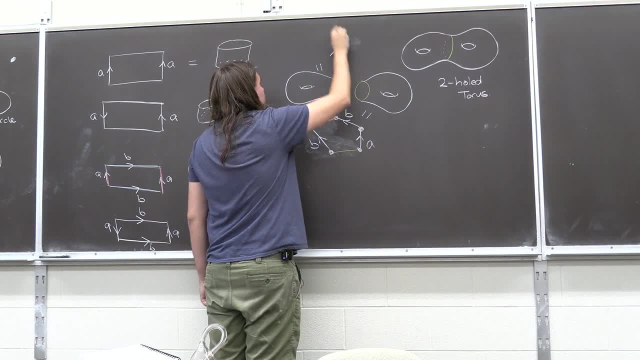 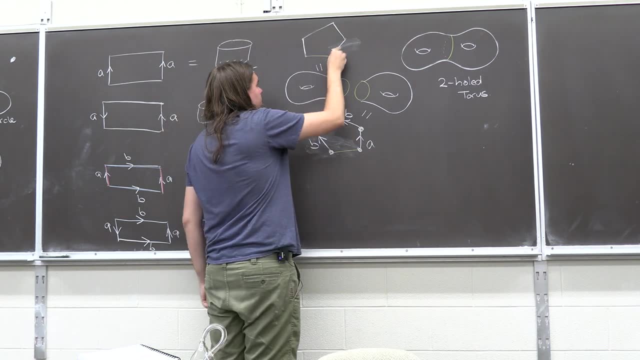 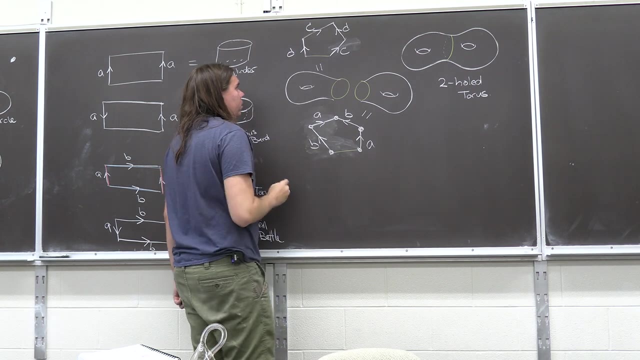 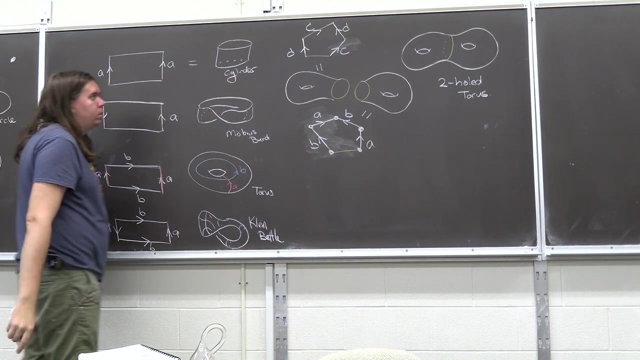 copy of this. But since I've already used A and B, I'm now going to use C and D. Notice the pattern: Two in the same direction, two in the opposite direction, Two in the same direction, two in the opposite direction to get the torus. That makes sure when. 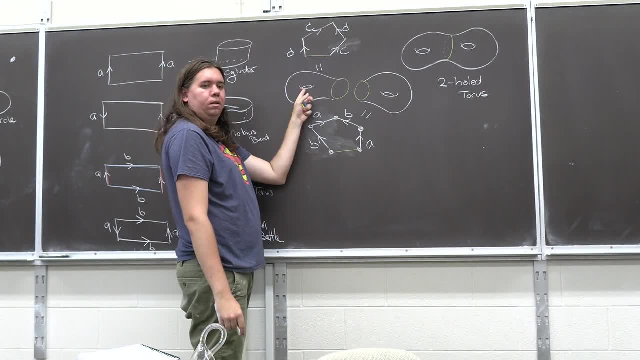 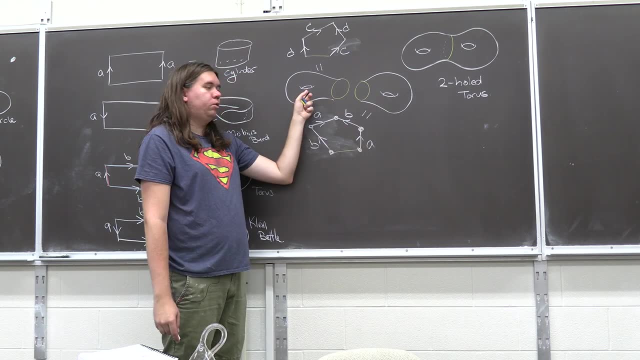 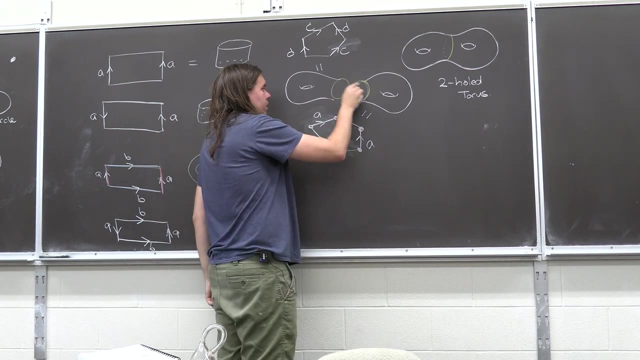 you glue these C's together and glue the D's. you get the torus. So now we know how to build the left and the right-hand side of the two-hole torus. How do we end up with the two-hole torus? Well, we just glue together this. 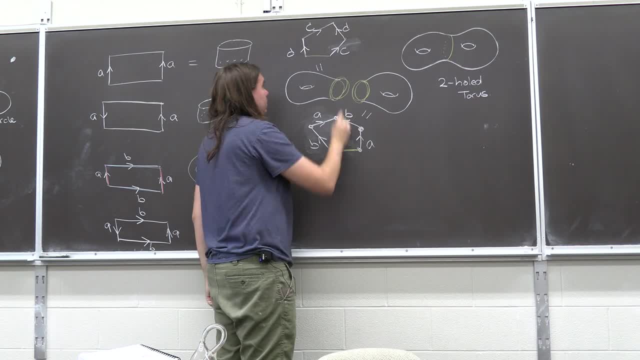 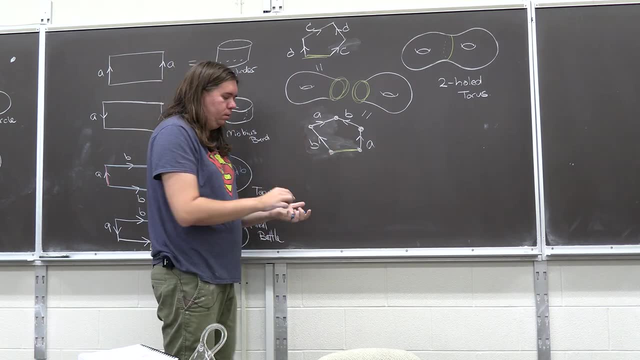 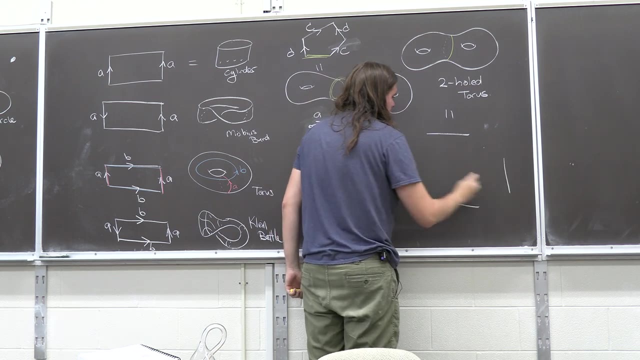 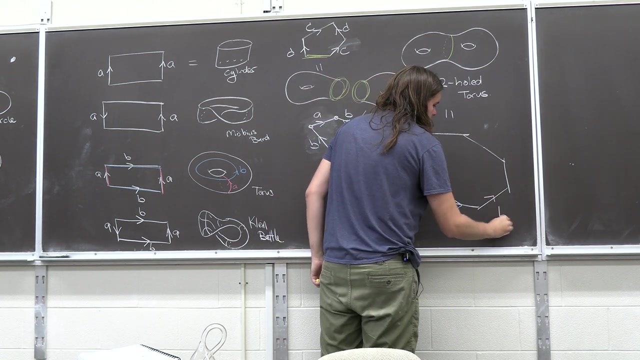 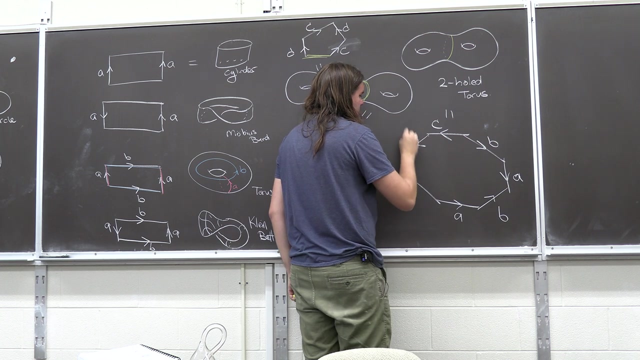 piece with this piece. So we just glue together this piece with this piece And when you glue them together, what we're gonna end up with is an eight-sided shape. So the two-hole torus you can get From gluing together this eight-sided shape that goes A, B, A, B, C, D, C, D. That's a two-hole torus. 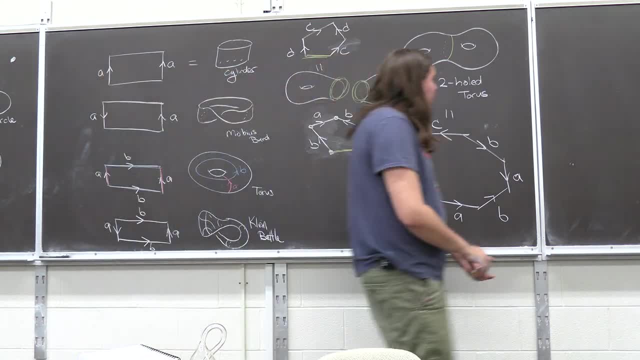 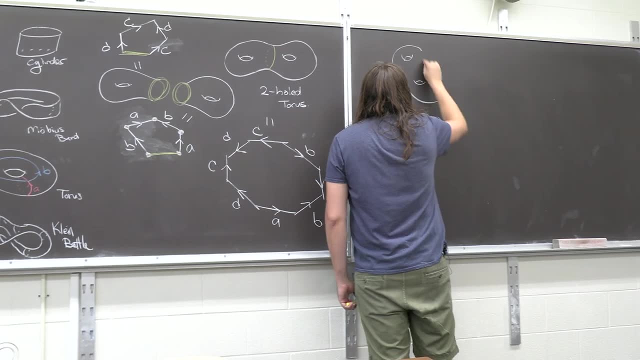 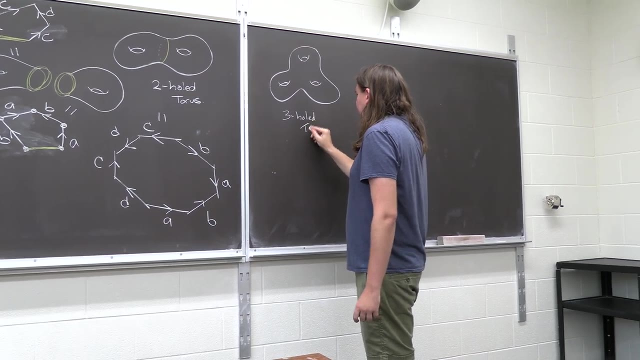 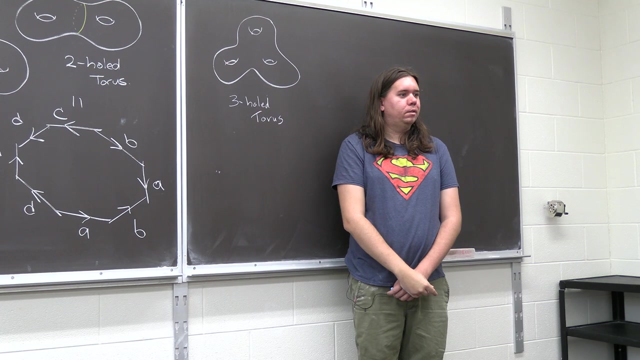 So now I'm going to test to see if you understand the idea. You tell me what are the gluing instructions for a three-hole torus. What can we glue together to get a three-hole torus? For two holes you need a stop sign. 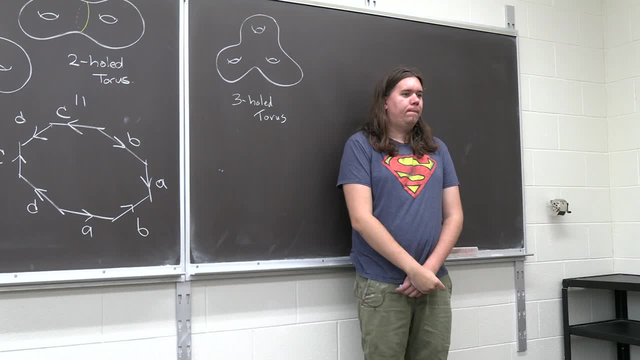 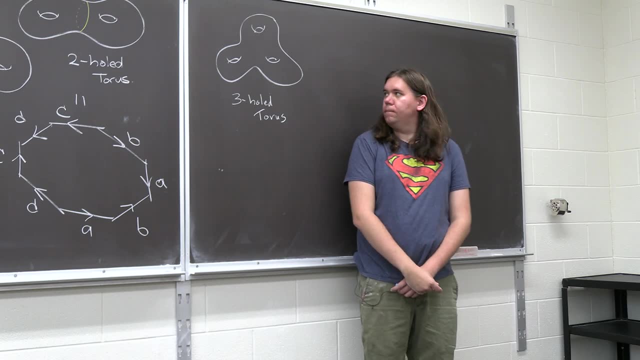 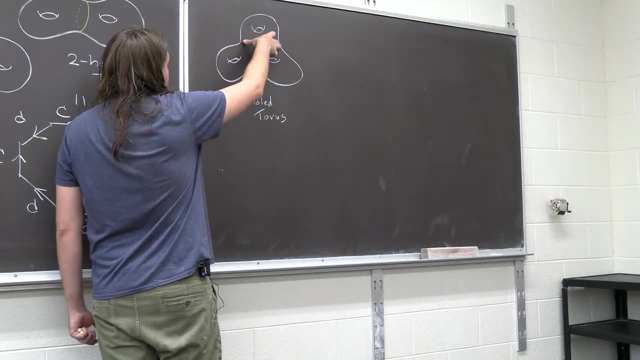 What do you need for a three-hole torus? Can you take a cross-section that separates one hole from two holes? Then you can take our diagram for the two-hole torus and have like an extra. Yeah, so you can be like this: If you cut this guy off, you'd have a two-hole torus with a line on the side. 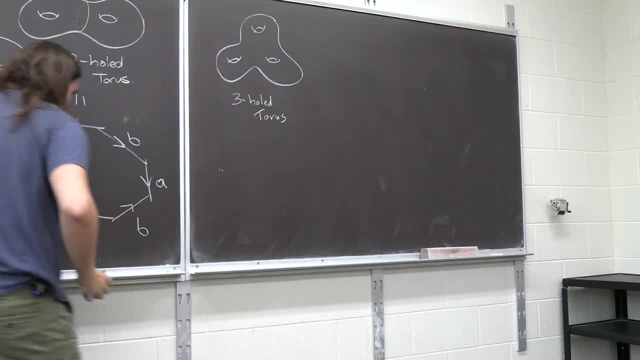 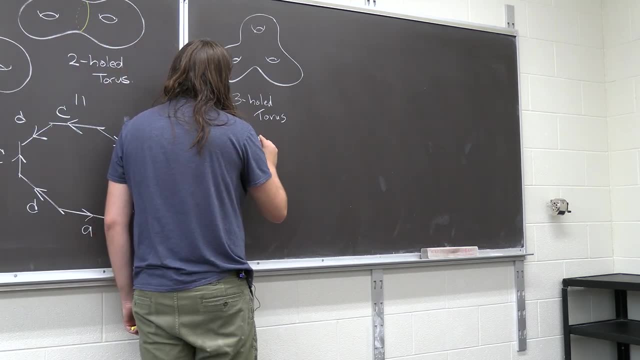 So there's like an extra line on the side right here And then you just add in a torus to it, So you're sticking in four more sides. So what are you gonna end up with? A twelve-sided shape. Twelve-sided shape, That's right. So let's try and sketch a twelve-sided shape. 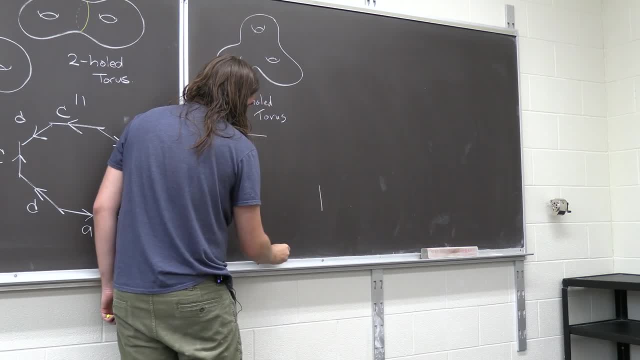 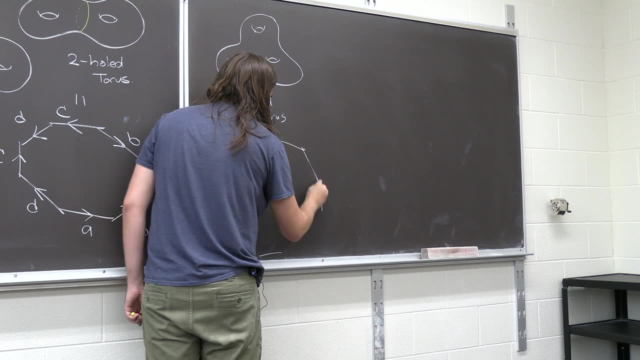 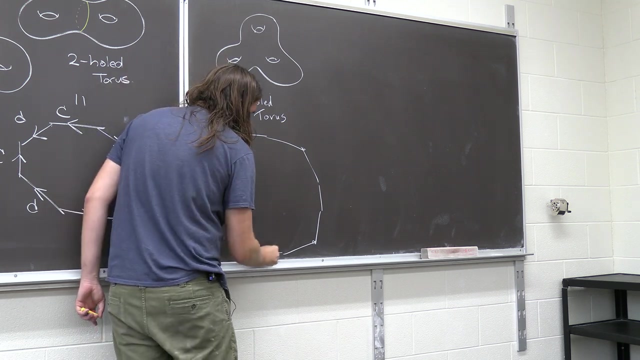 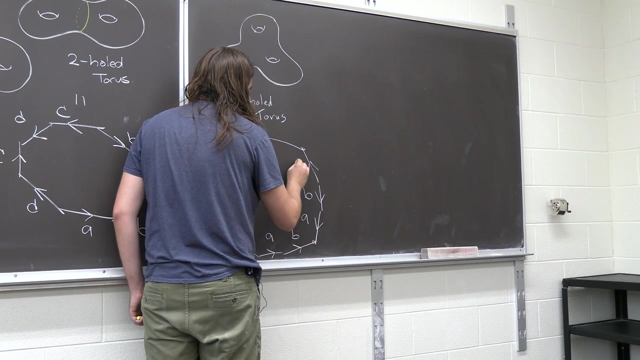 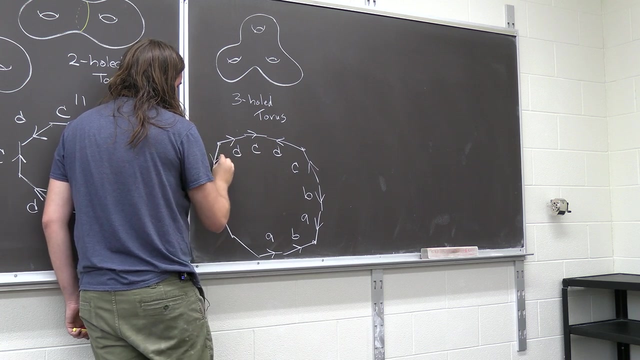 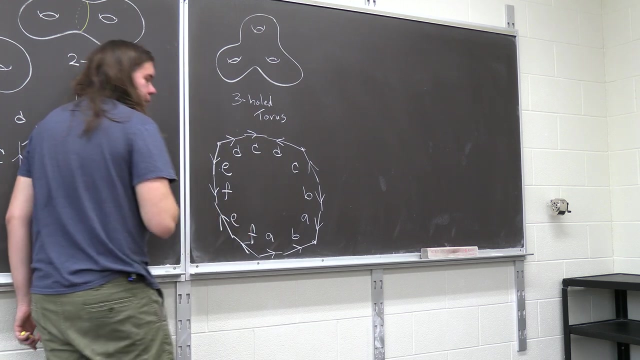 So twelve is, We can first do the four and then we'll break these up into two each, And now we can read it off as A, B, A, B, C, D, C, D, E, E, F, E, F. 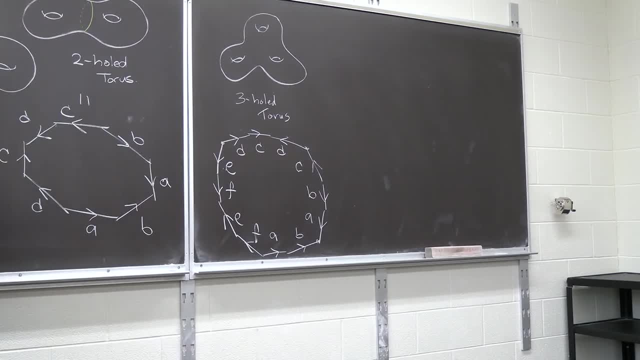 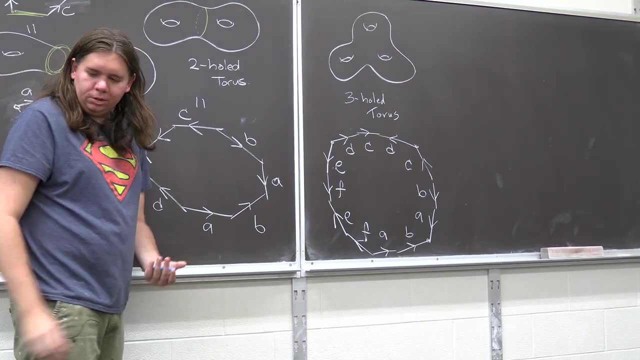 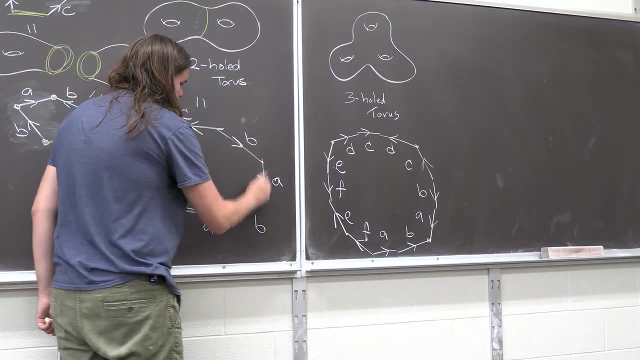 This gives you the three-hole torus. We got to see a little bit more what's going on here. If we look at what this A piece is, well, it depends how you fold it, But let's say A, let's say all these points. 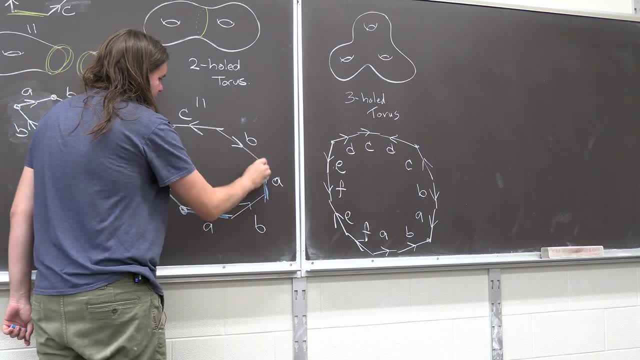 I mean these points are all the same point, Like this point. it's identified with this point. Now it's at the head of B, so it's identified with this point. Now it's at the head of A, so it's identified with this point. 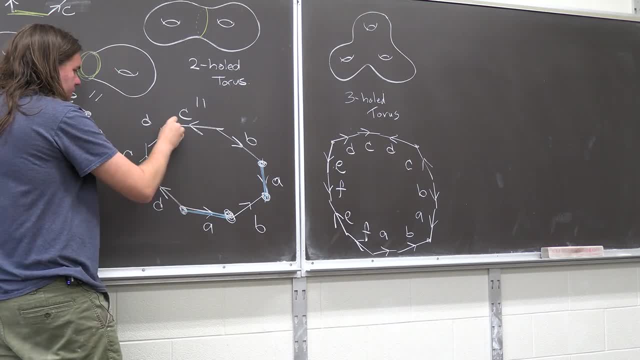 But it's also at the back of D, so the back of D gets glued to the back of D. Now it's at the head of C, so it's glued to the head of C. Now it's at the head of D, so it's glued to the head of D. 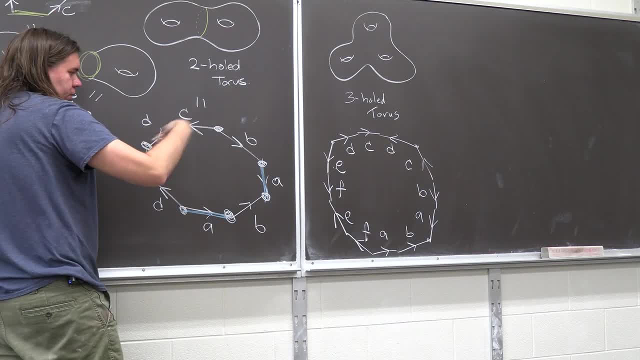 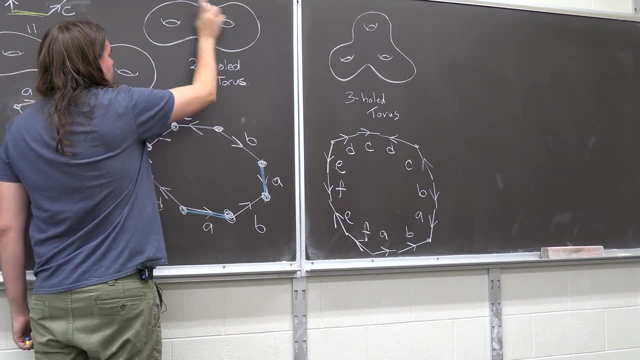 Now it's at the back of C, So all those points are the same. There's just one vertex here. It's all the same vertex. Let's just put that vertex like: right there, right, I'm going to forget about this yellow line now, because we glued it together, got rid of that. 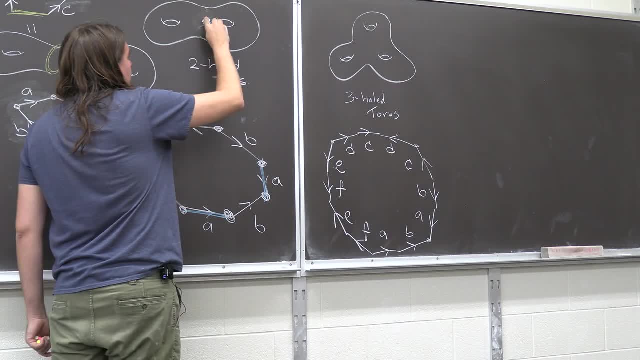 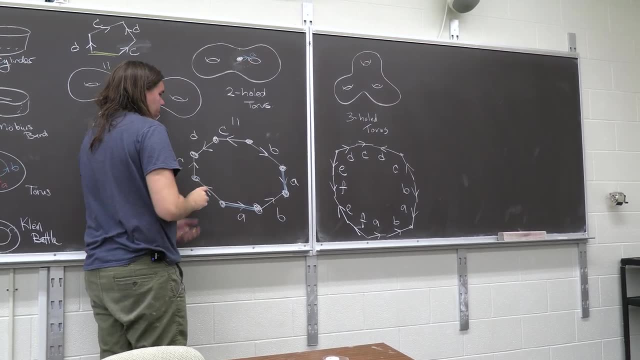 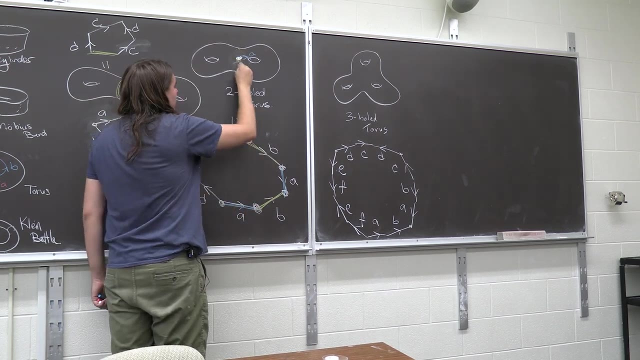 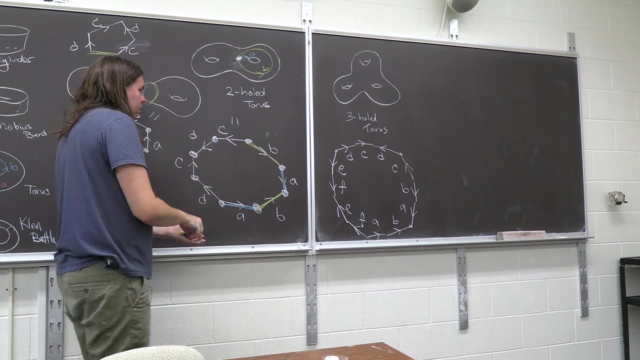 Then you can think of this A as just like some loop that goes around that part of the torus, So some loop. And the B is another loop where the B is like transverse. So you're tracing out this direction And your C. 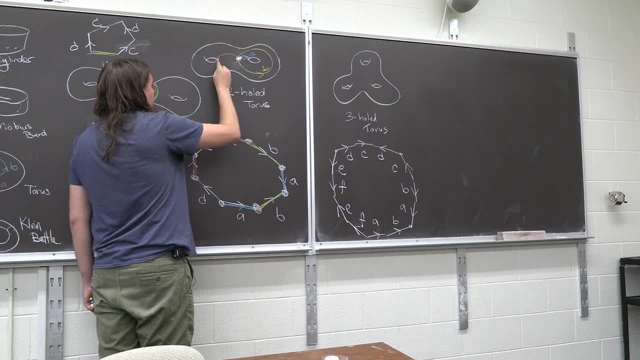 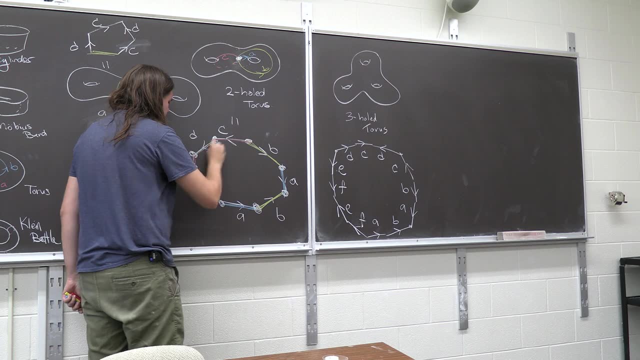 Where would C be Around the other side? Yeah, just around the other side, And you can change the order of these. that's fine. The point is your D. I'm out of colors, let's just do white is something like this: 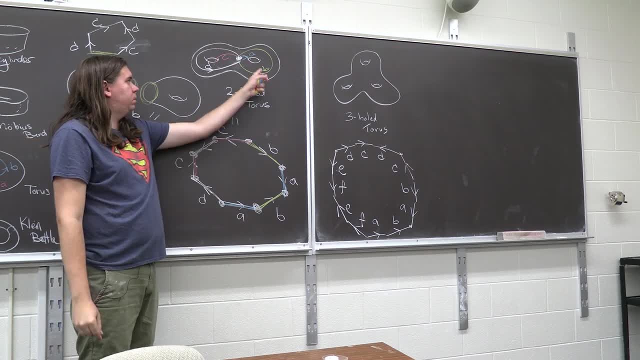 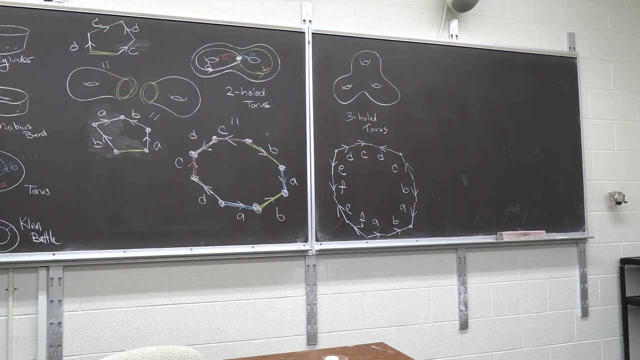 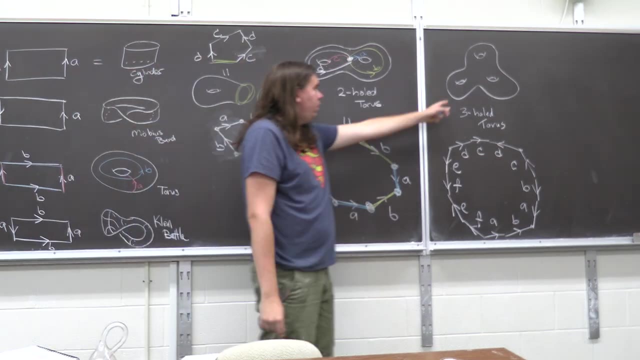 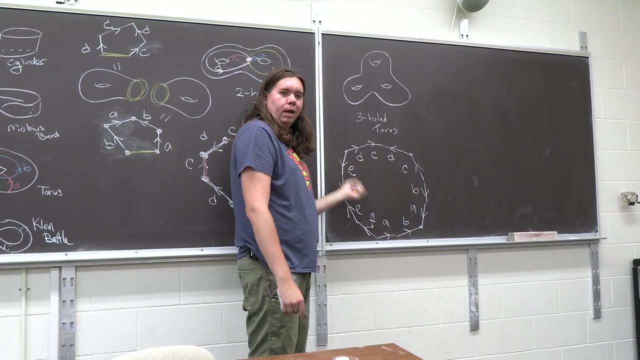 So you need two loops to describe a whole, Just like your original torus was described by two loops, And so when you have three holes, you're going to need six loops, But since you're gluing two together, you need 12 sides. 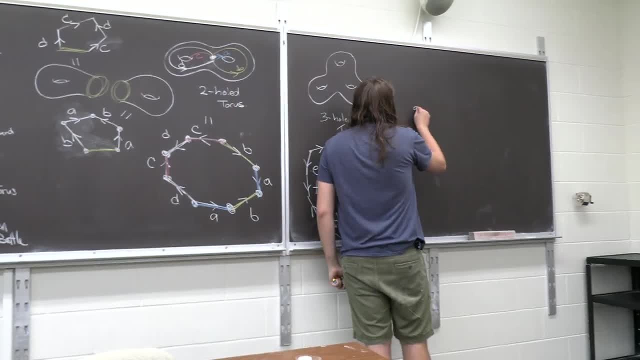 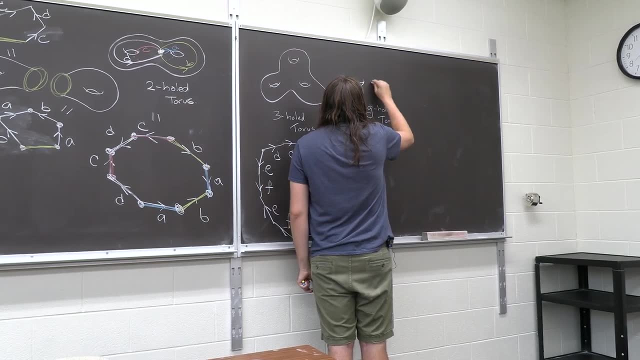 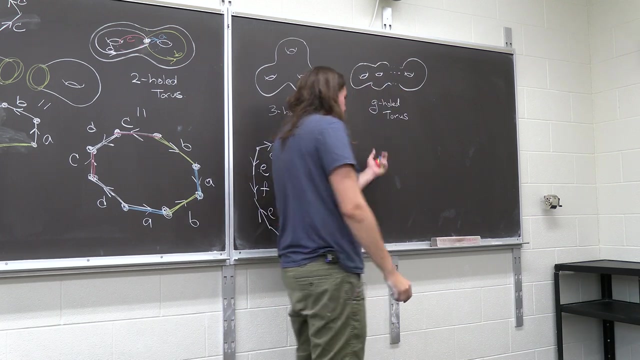 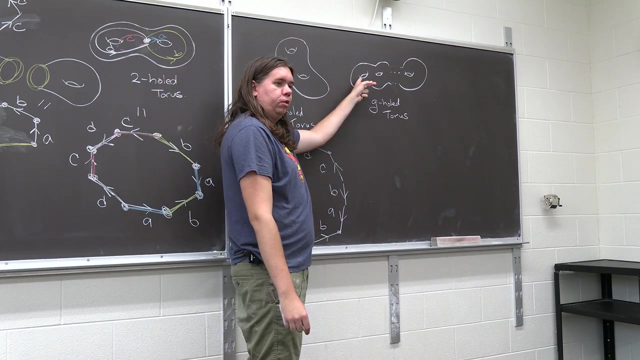 And in general, a G-hole torus- Where we want to have G-holes- Is going to need how many sides. You need two loops for each of the G, So you need two G loops, But then each loop is represented by two sides. 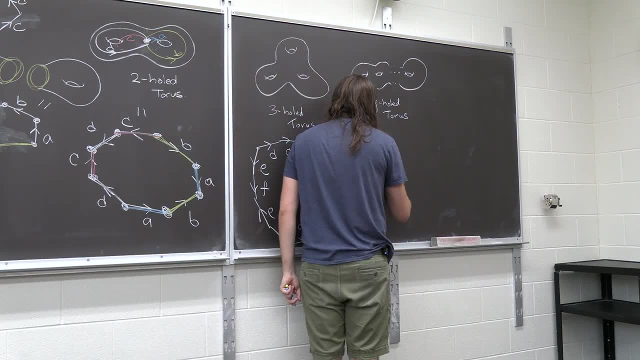 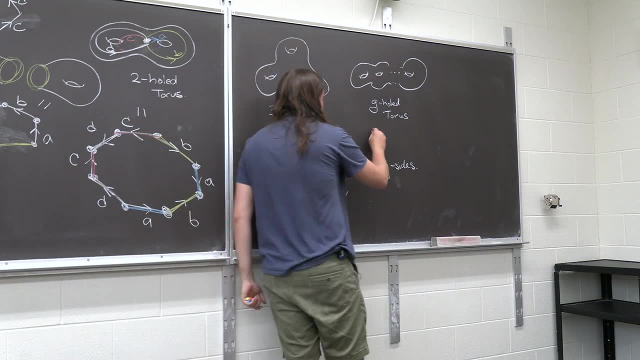 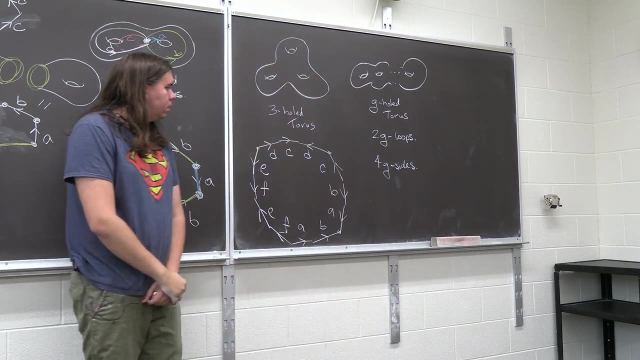 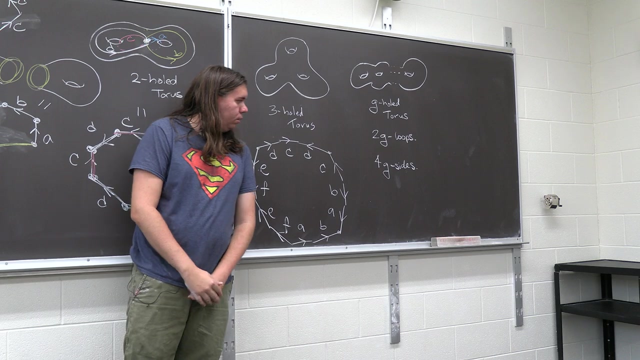 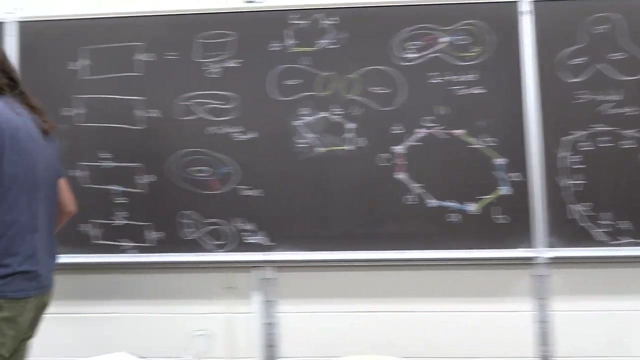 So two times two G, it's going to be a four G-sided shape Where you have your two G loops, Okay. So we can keep building up things like this, But what I want to do is describe a general way, Okay. 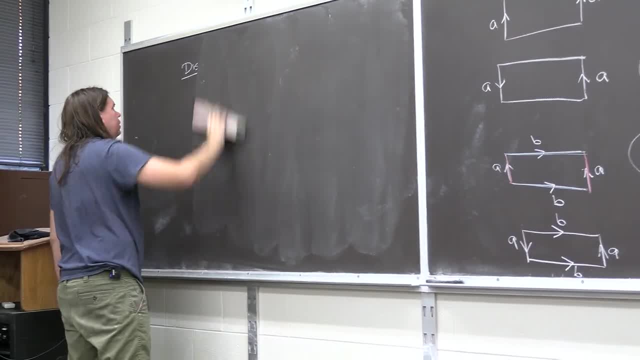 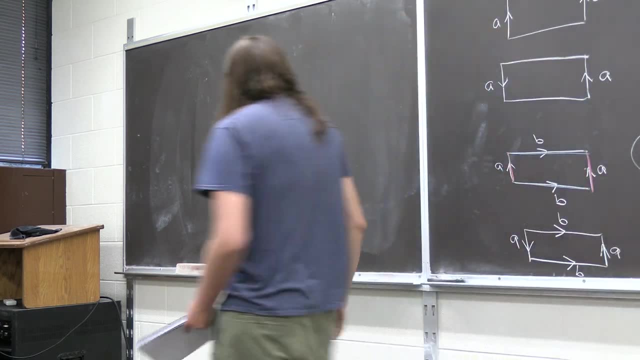 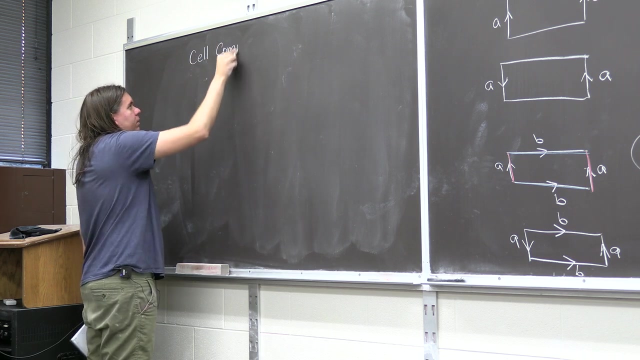 Of building such spaces, And what I'm going to describe now Is how we build what we call a cell complex. We're going to see. all these things are examples of cell complexes. A cell complex. Sometimes you'll also see this referred to as a CW complex. 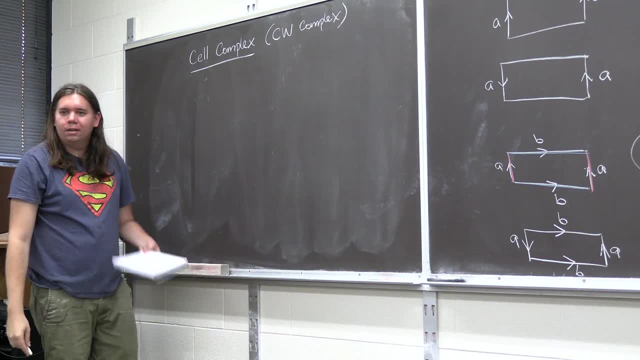 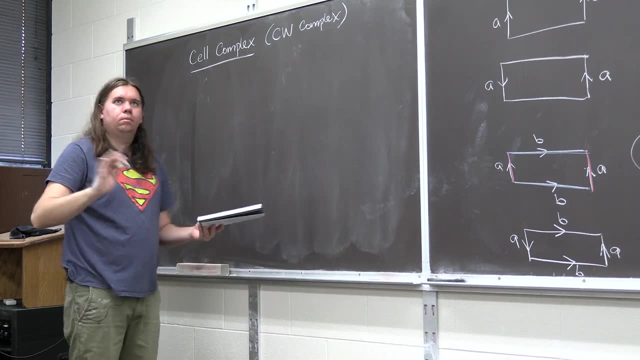 CW is not a reference to the failed media company. It's a reference to So. C is closure of finiteness, W is weak topology. We may get into this a little bit. Don't worry about what that means for now. But let's talk about how we build a cell complex. 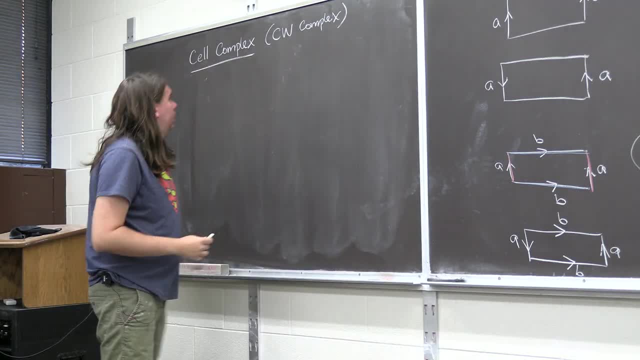 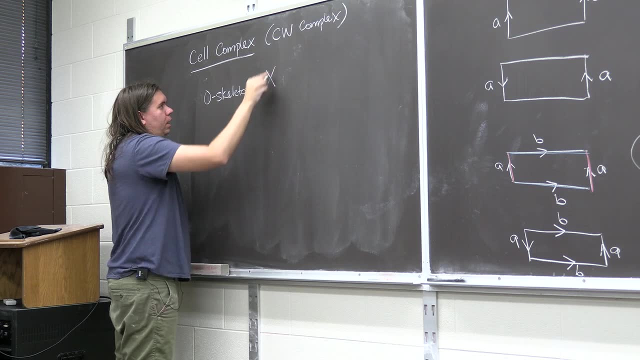 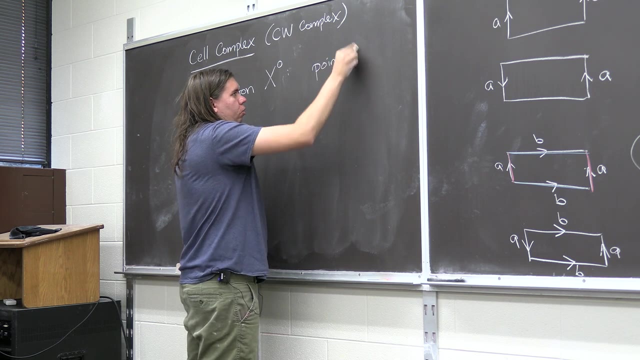 So the way you build a cell complex Is you begin with what I'm going to call the zero skeleton, Which is denoted X, zero. And what the zero skeleton is Is it's just some collection of points Or points, So maybe several points. 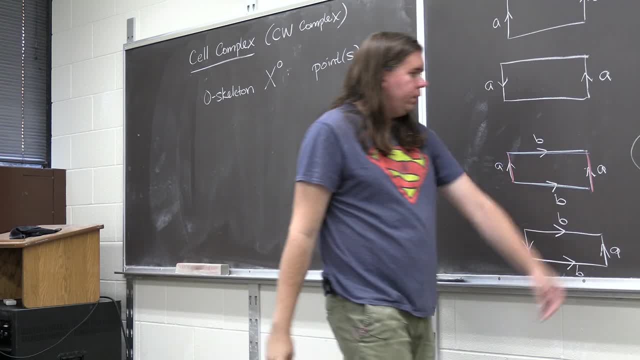 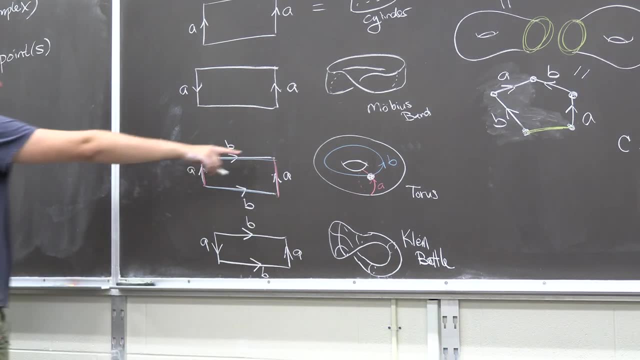 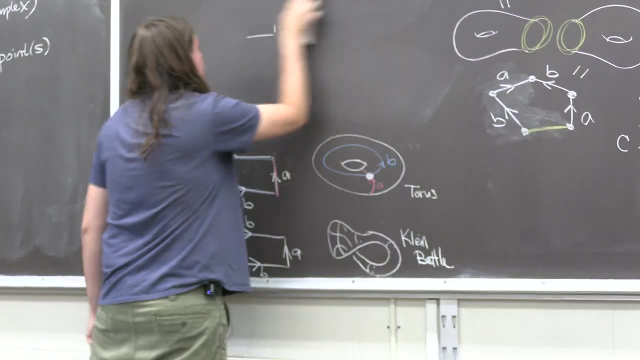 Over here in the example of the torus, My skeleton would be just a single point. So if I'm thinking about the torus, I have a single point. Let me up here, build the torus One step at a time. So my zero skeleton for the torus. 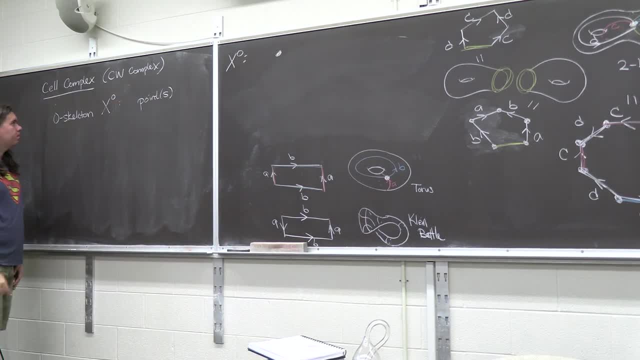 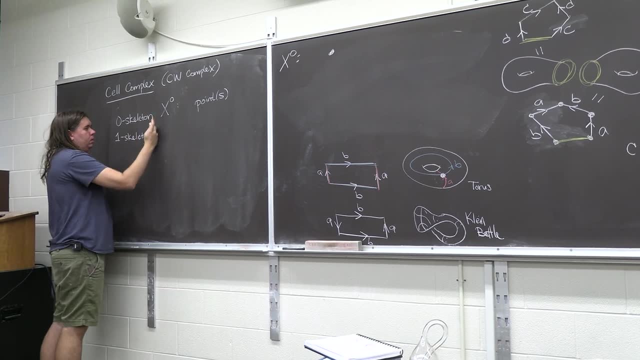 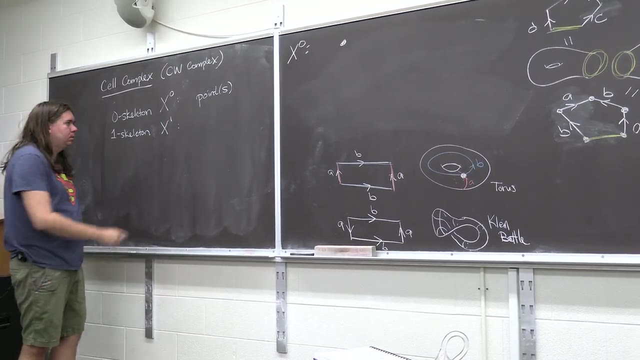 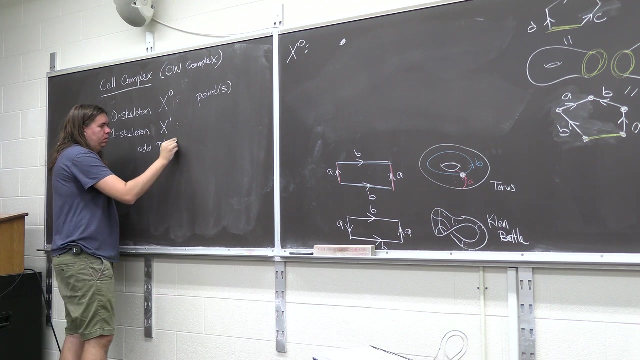 Is just a single point, Then My one skeleton Is what's going to happen when I take that point And I add to it some lines. So I'm going to add copies of D1 or of lines, Possibly one, possibly several. 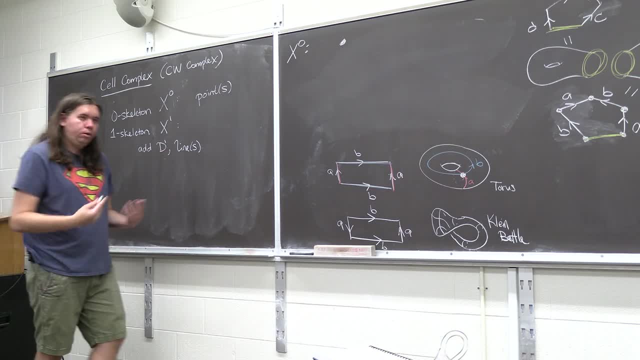 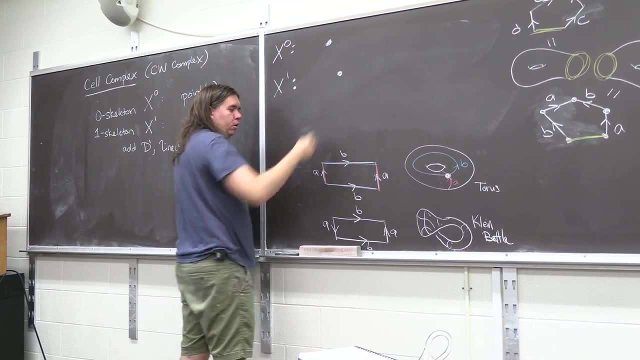 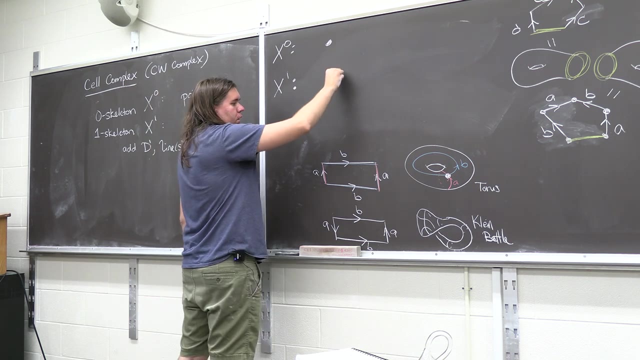 In the case of the torus, You only need to add two lines. So your X1. Is your dot, With two lines added, One which I'll draw Like this And one which I'll draw like this. I added two lines. 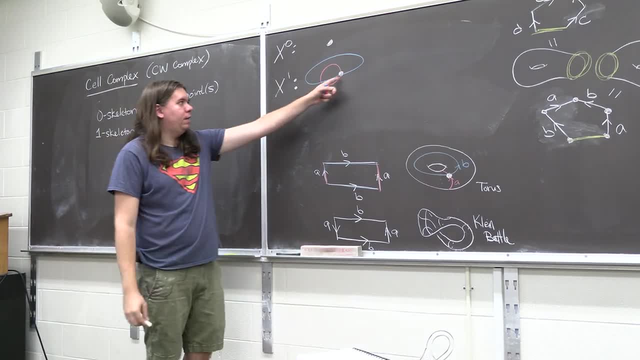 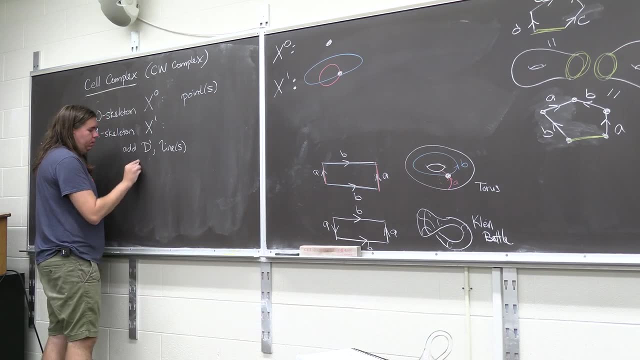 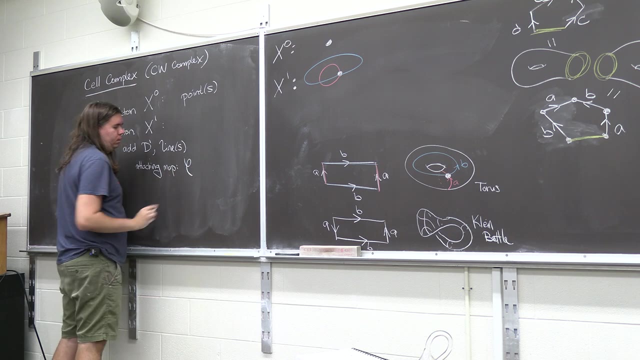 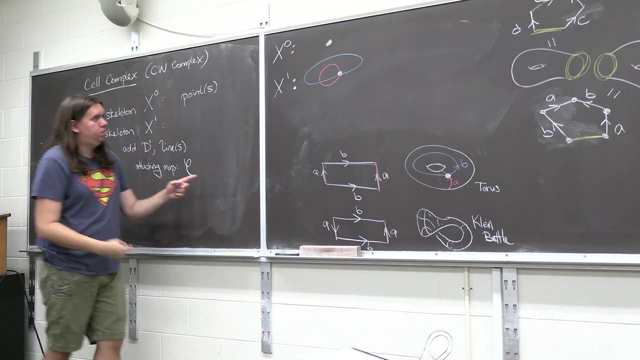 But notice, those lines Were attached to the zero skeleton And so for each D1. There's some attaching map That explains how D1. Gets attached to the zero skeleton. In particular It explains how the endpoints get attached. So it's a map. 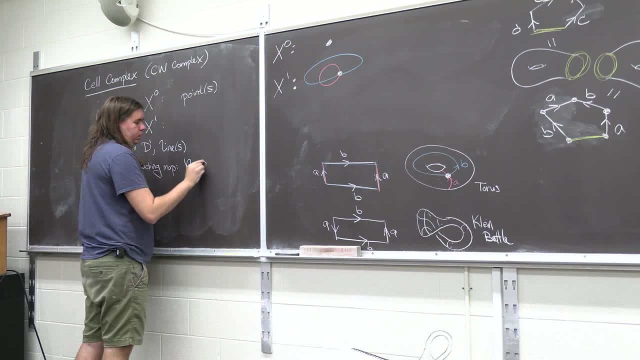 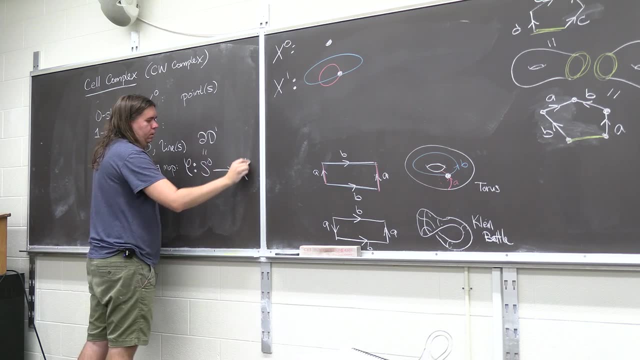 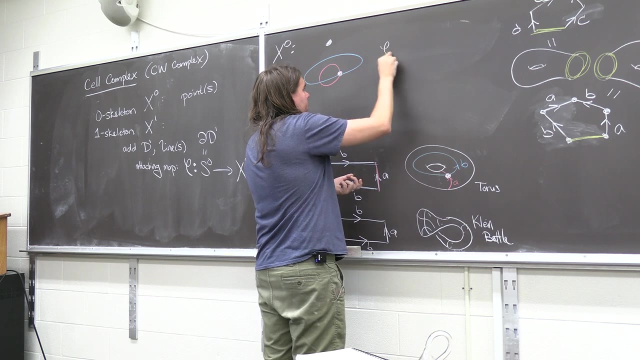 From the boundary of D1.. Which is S0.. That's the boundary of D1.. This is the boundary of your D1.. Onto Your zero skeleton, And here This is a really trivial map. Your phi Is just the map. 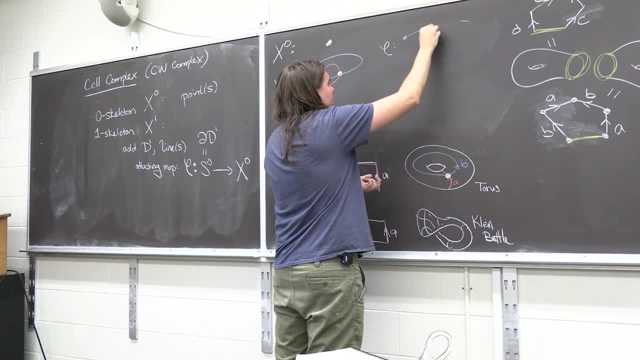 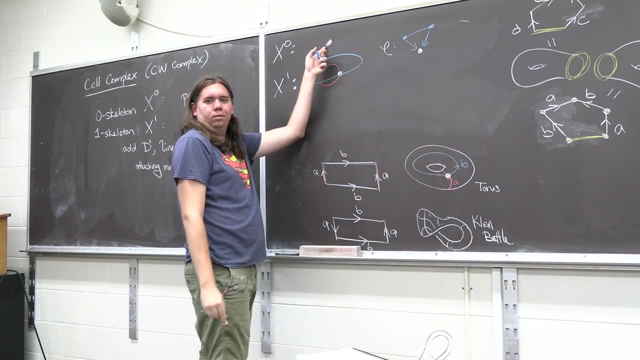 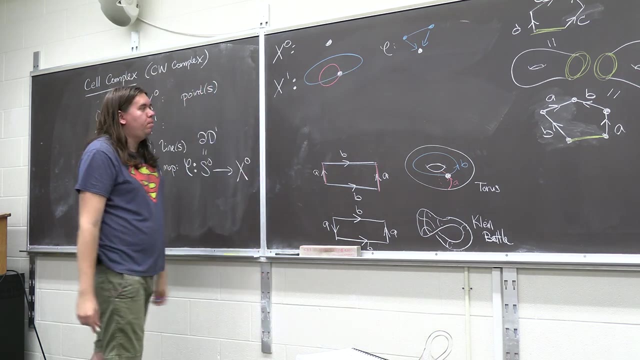 That takes Both endpoints And sends both of those endpoints Onto Your point in the zero skeleton Right, And same thing, Same thing for the red one. So this is a really trivial map here. But you might have Say, if you start with two points, 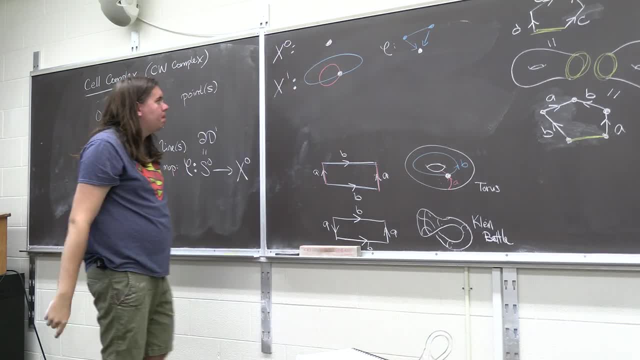 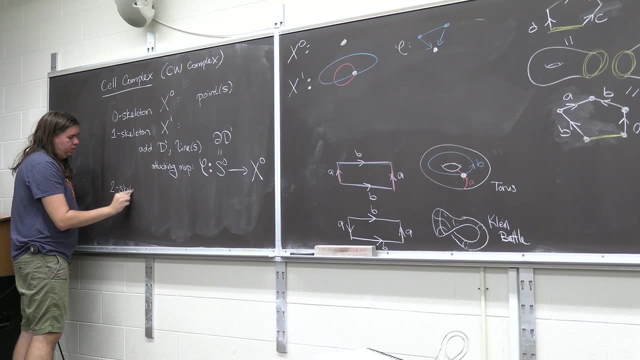 You could also have lines That connect those two points. Right, It could be more interesting. What we're going to do next Is we're going to move up To the two skeleton, Which I'll denote by X2.. And what I'm going to do now? 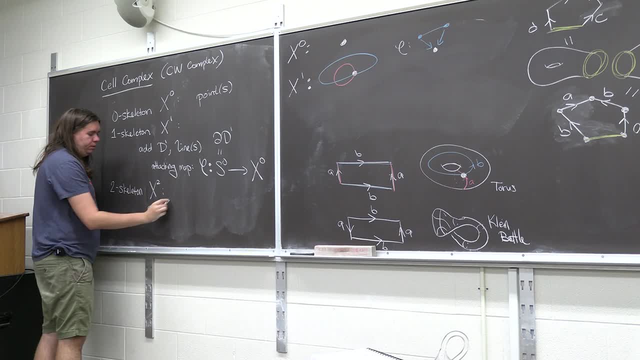 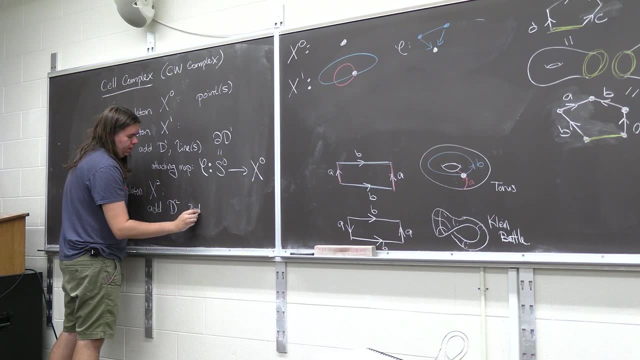 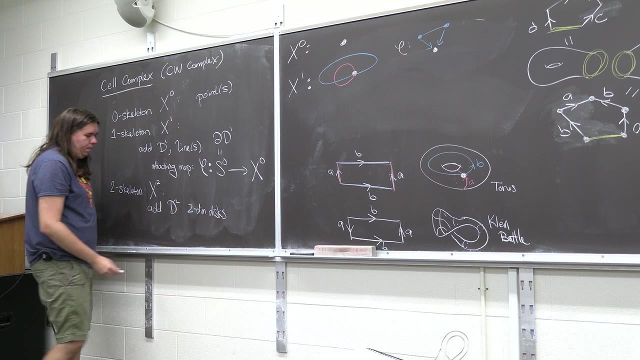 Is. I'm going to add some copies Of D2.. Some two-dimensional disk. So these are now My two-dimensional disk, My two-dimensional disk. According to some map, That's going to take The boundary of each disk. So the boundary of a disk is a. 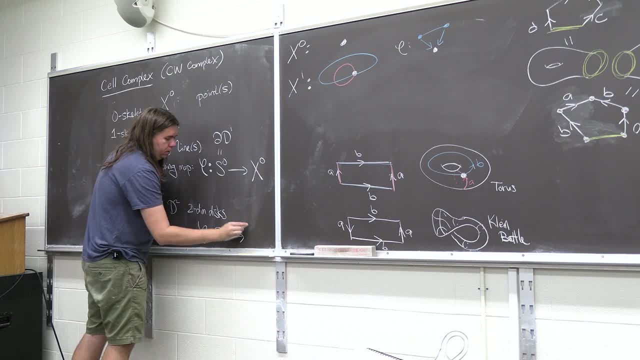 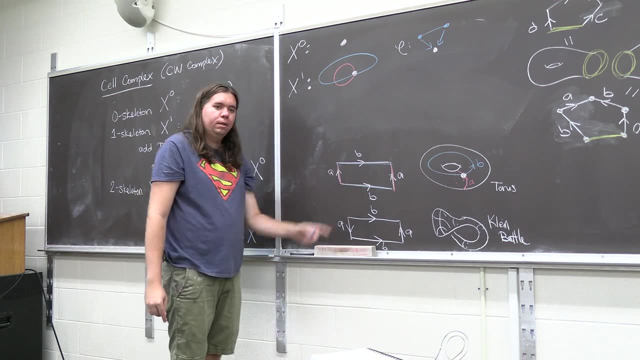 Circle S1. And attach it To my one skeleton, And I claim that's exactly what this is doing here. This is a copy of your map, Because what it's saying is: You Glue the circle By beginning to glue it onto A. 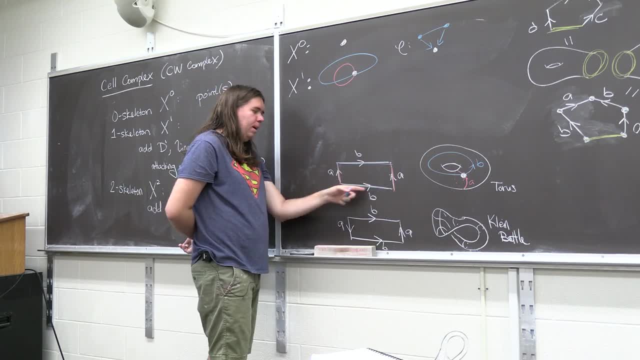 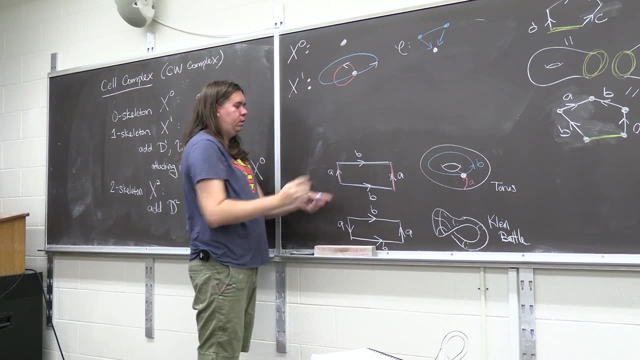 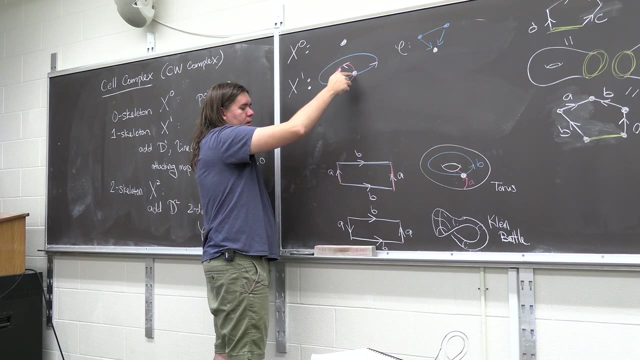 Then onto B, Then onto A, Then onto B, Respecting these directions. So if I give these guys Some directions, The way it takes a circle And you can imagine beginning to glue the circle First along this A And now that's glued along this A. 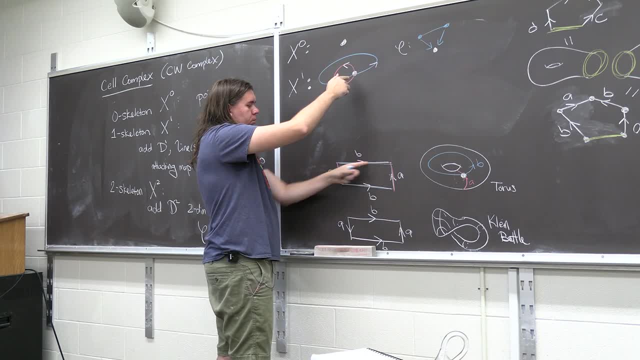 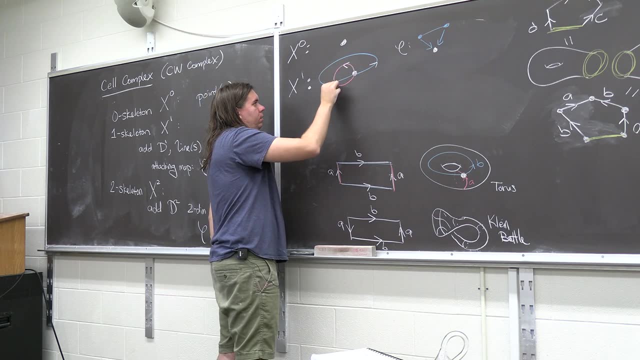 You're going to glue it along B. In this picture it's going Against the arrow, So we're gluing it now here. So what it does is it starts Gluing a circle along here, Then it glues it Along here. 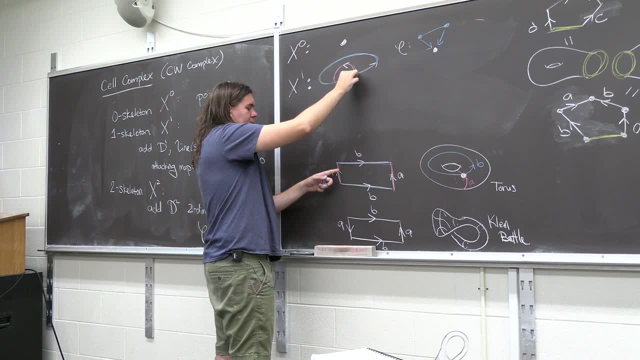 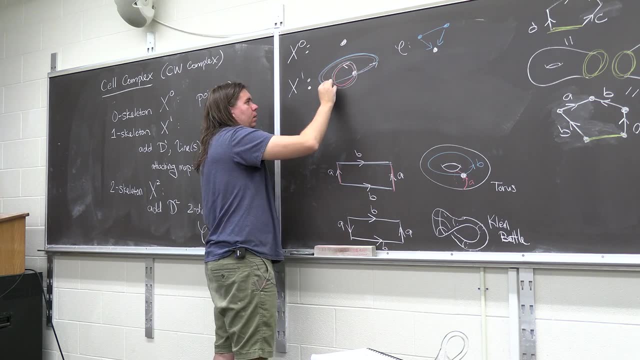 And then it glues it against A, Going against the flow, So going this way along A, And then glues it back along B, And so you should take Like a minute to convince yourself That this is indeed how you build a torus. 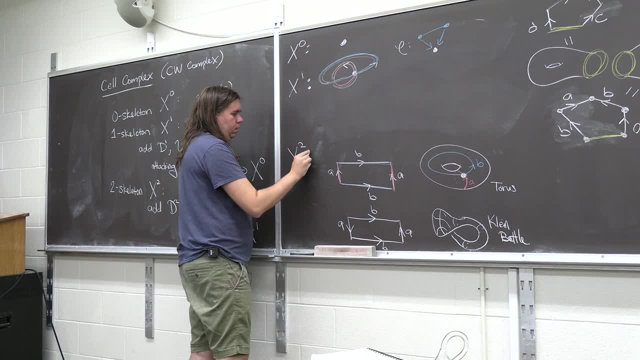 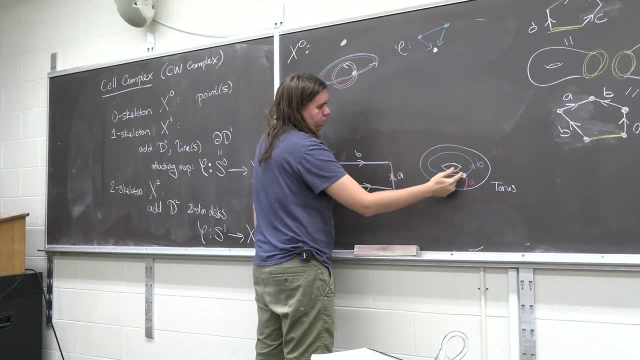 This right here just is The two skeleton for a torus. You take that circle, You begin gluing it onto A, Glue it onto B, Glue it onto A, Glue it onto B, And you might want to build like a wire mesh of this. 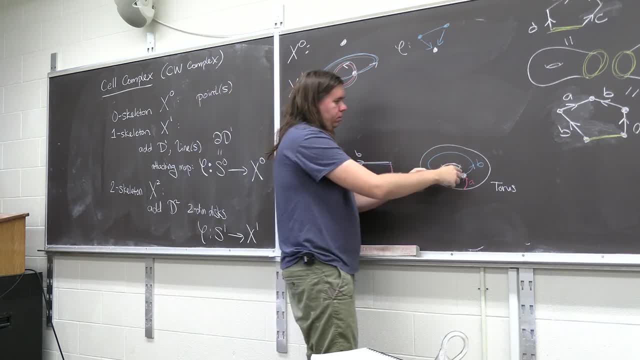 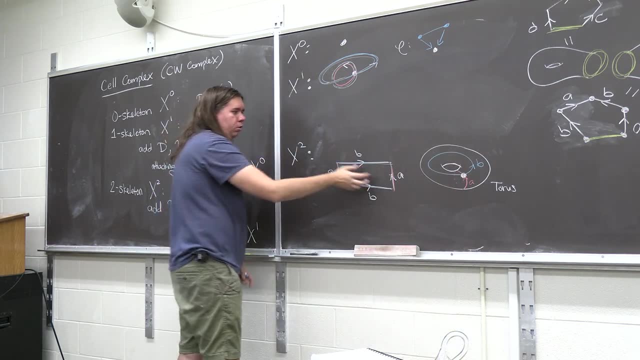 And imagine gluing on the. You know How you would have to glue on each one of these, The four sides of it, But that's really what this here is. This is a map describing how you glue the disc Onto your one skeleton. 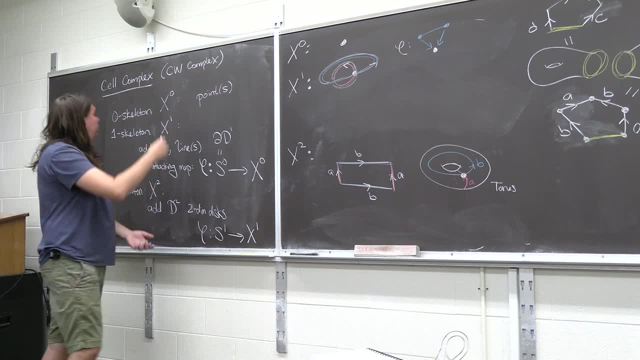 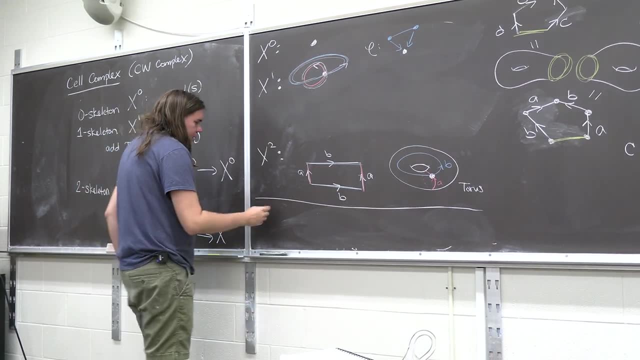 Okay, And you could continue this, You know, if you want to, If you want to go higher, If you have a higher dimensional object You're trying to build In general, you could have some end skeleton Xn, Which is just adding some. 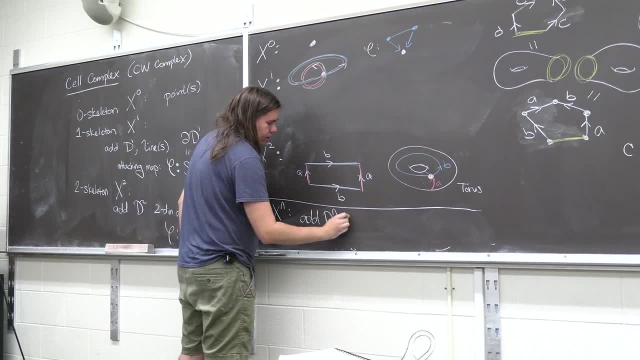 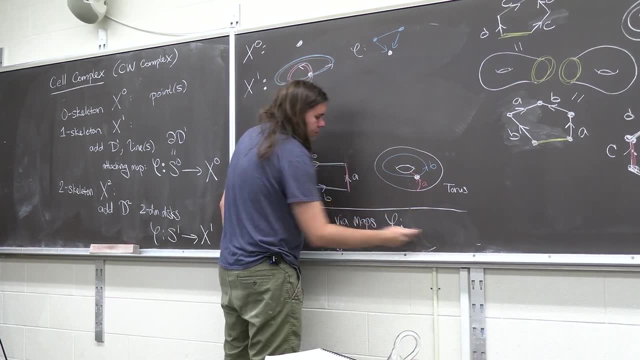 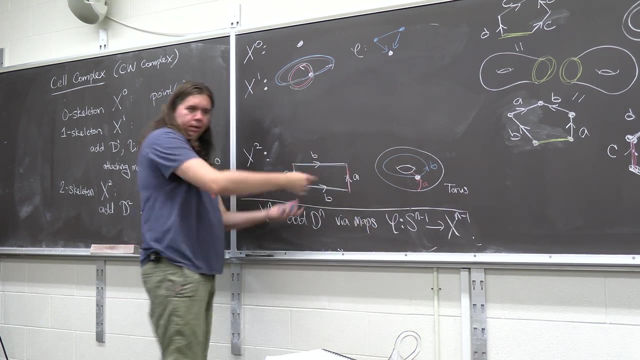 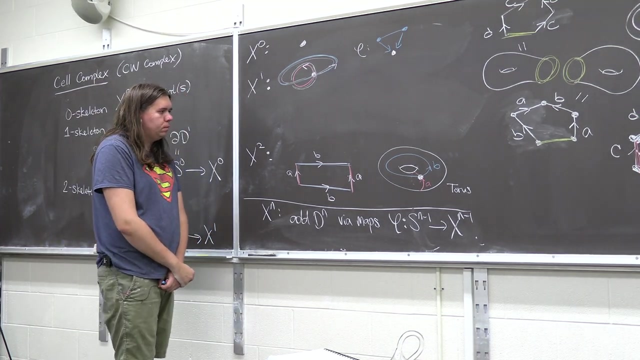 Copies of Dn Via maps That are attaching Each boundary Of Dn, So each Sn-1.. To the n-1 skeleton, And you can keep doing this. Okay, So this is a Cw complex. 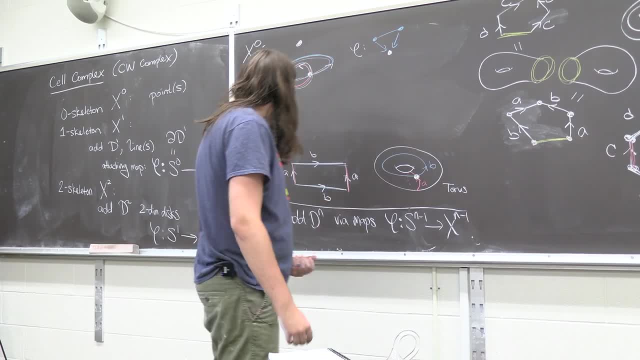 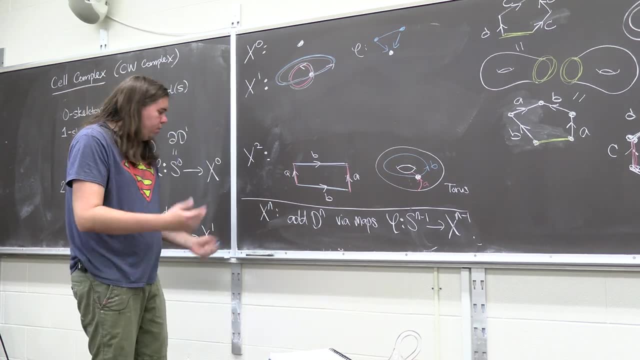 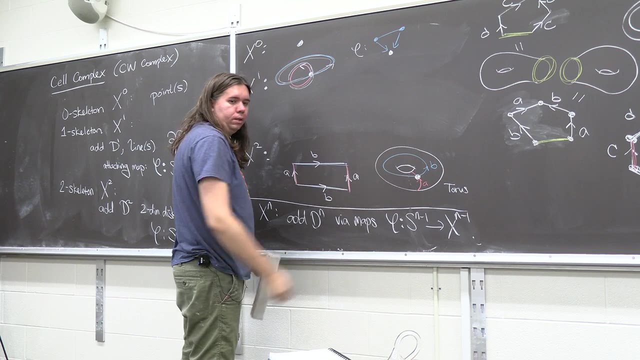 Or a cell complex. Here I showed you one way To build the torus, But there are other ways You could have built the torus too. You didn't have to use One point and two lines To build your torus. 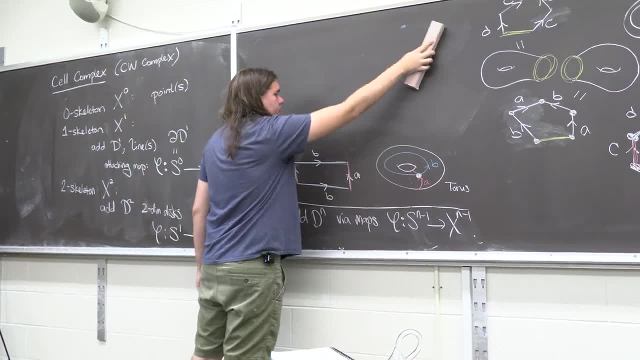 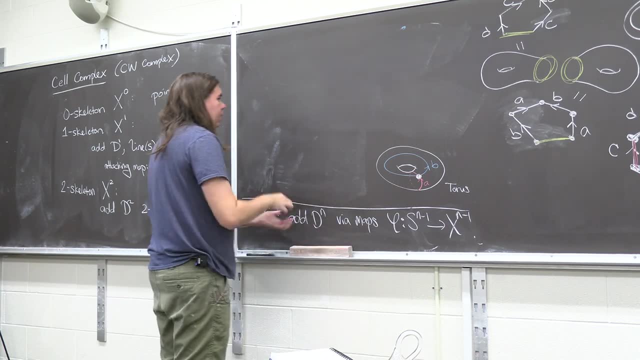 What's another way You might have built your torus? So here I have one point and two lines, So I'll just record some data here. I've built my torus here So that if I count the number of D0s, 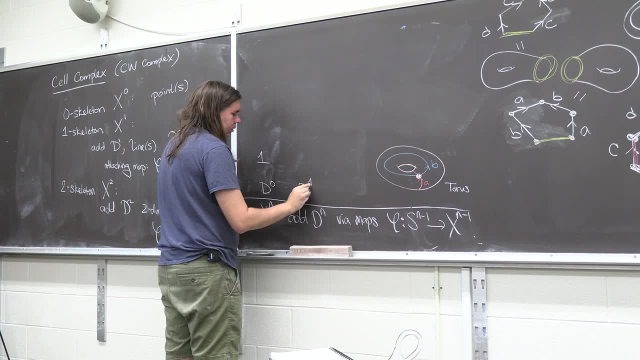 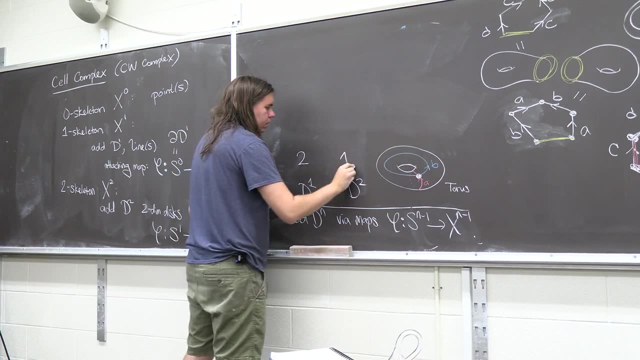 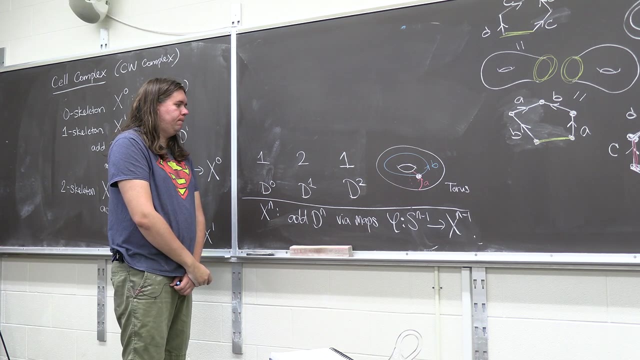 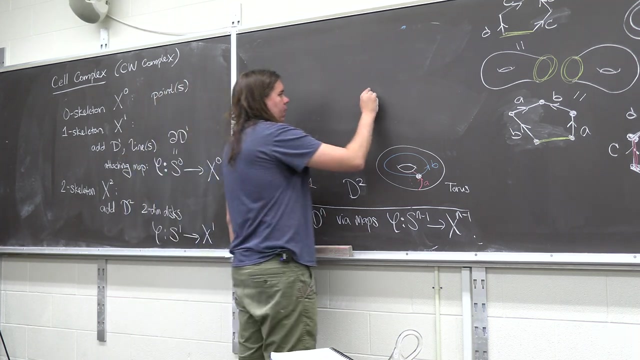 There's one of them. If I count the number of lines, There's two of them, And then I count the number of discs needed. There was one. Give me another way to build a torus. Let's use more points, So I'll give away the final shape. 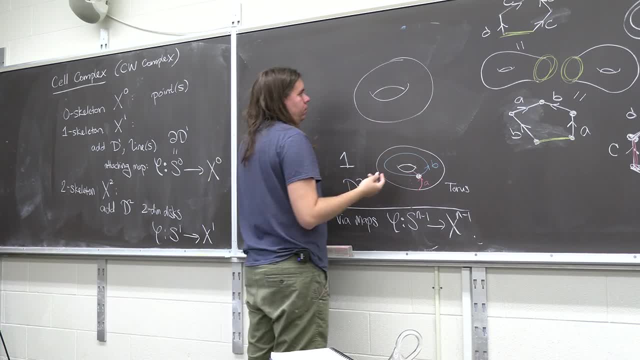 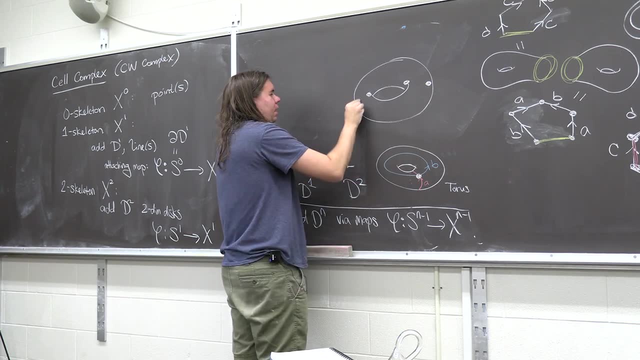 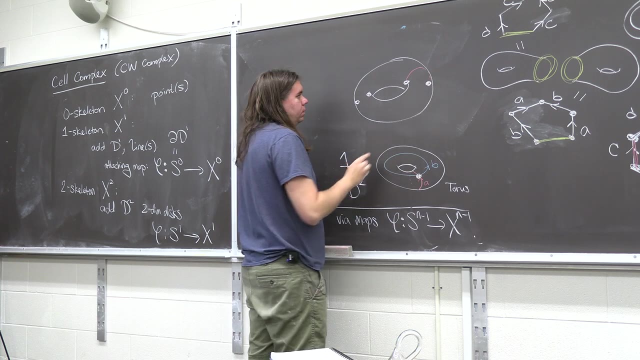 But let's use more points. Let's use, say, Four points. Try and put this on the opposite side. Try and put this on the opposite side. Then what I could do Is I could attach these two points Above the torus. 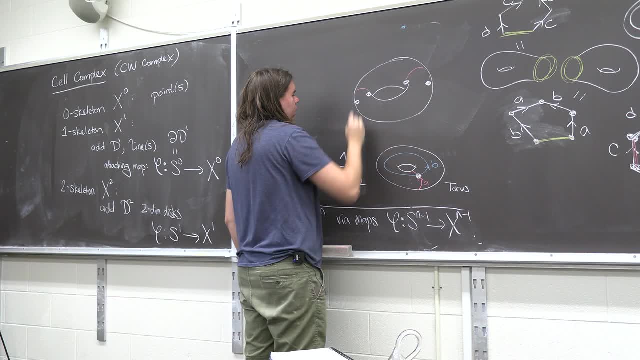 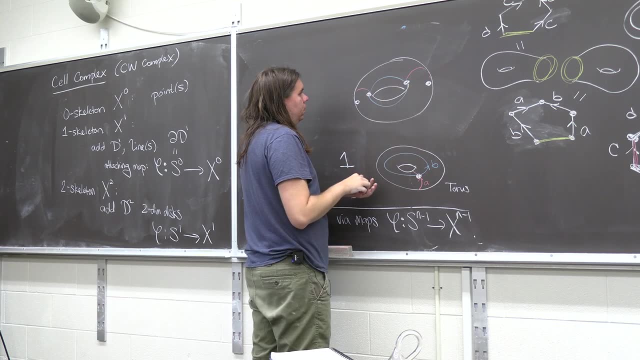 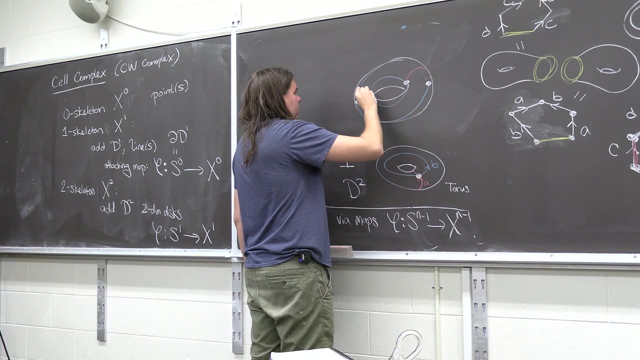 Attach these two points Above the torus. Attach him going around. Attach him going around. I'll also attach him Going around like this And I'll attach him Going around And I'll attach those two points at the bottom as well. 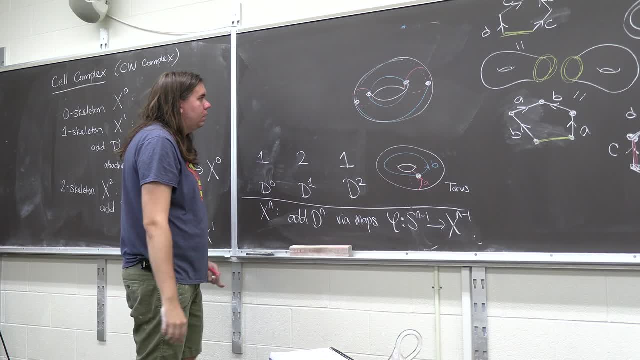 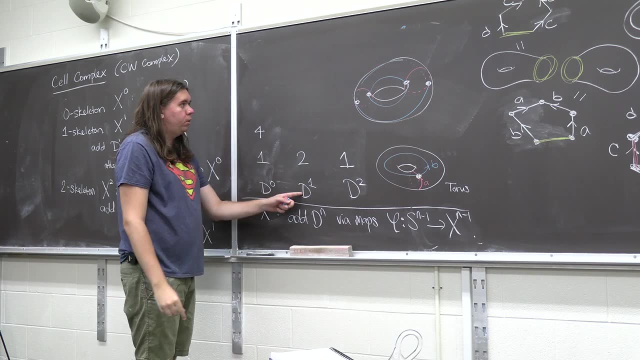 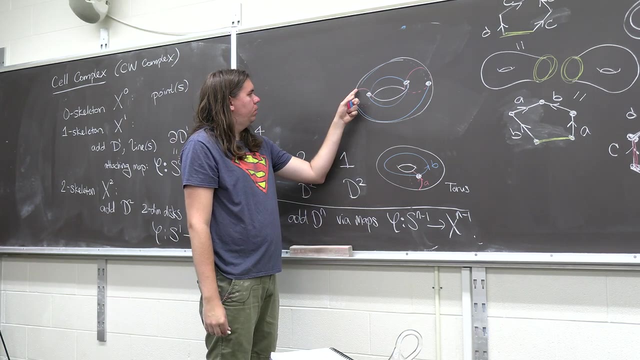 Okay, do you see this wire mesh I'm trying to build? So let's keep track of how many points we used. Four points, The zero skeleton is four points. For the one skeleton, how many lines did I add? Okay, one, two, three, four, five, six, seven, eight. yeah. 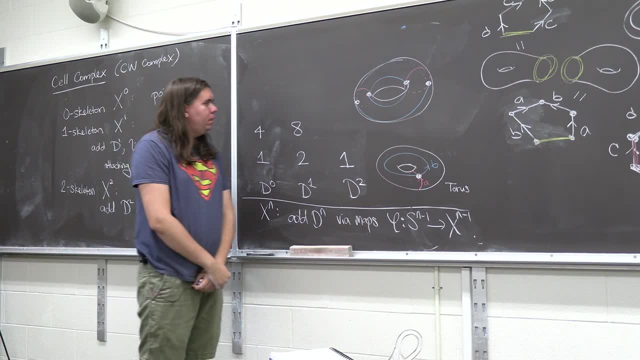 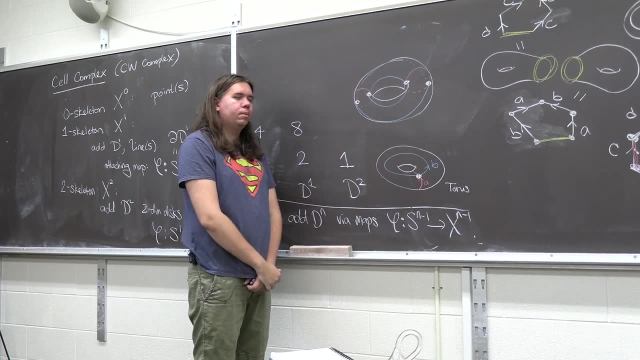 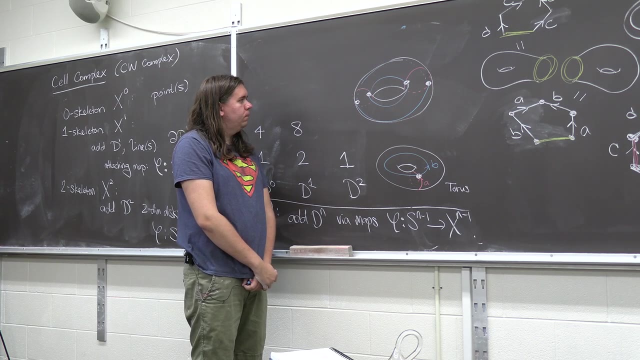 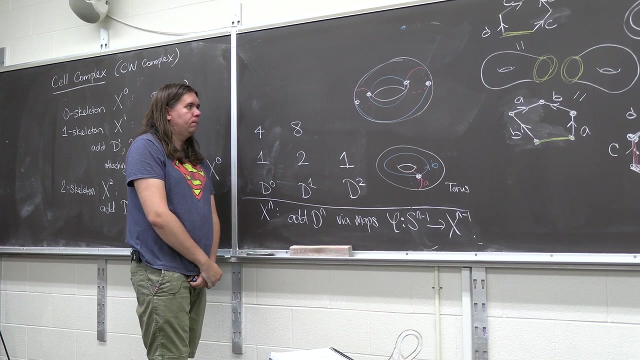 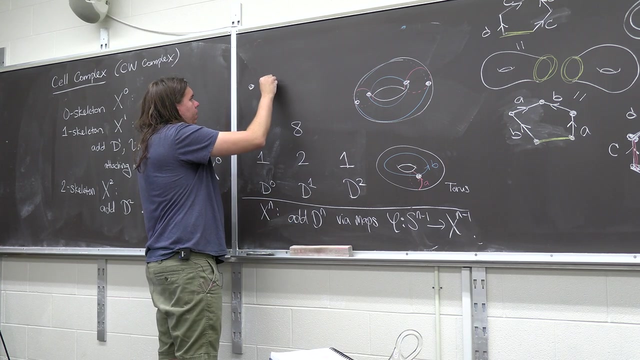 And now's the moment of truth. Can you tell me how many discs it takes to glue this together? How many discs I glue on to finish this guy up? Four, Yeah, that's right. So maybe this wasn't the optimal diagram, but I can try and draw it again here. 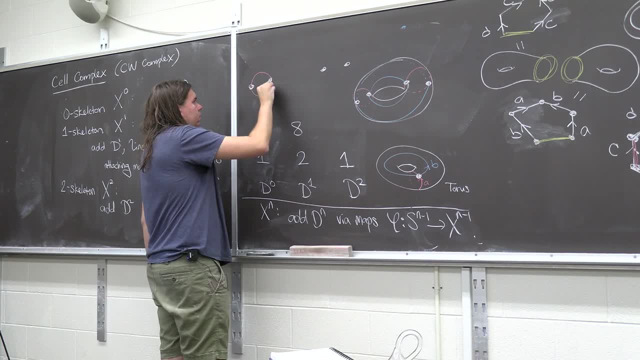 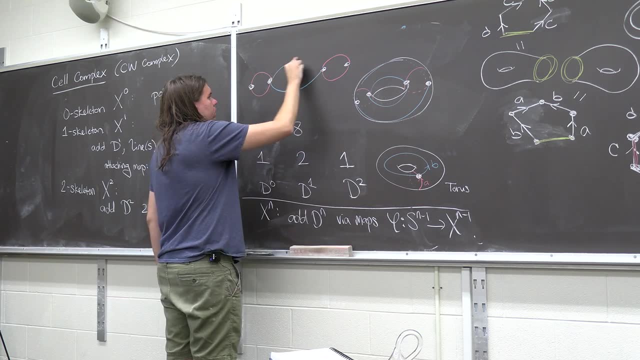 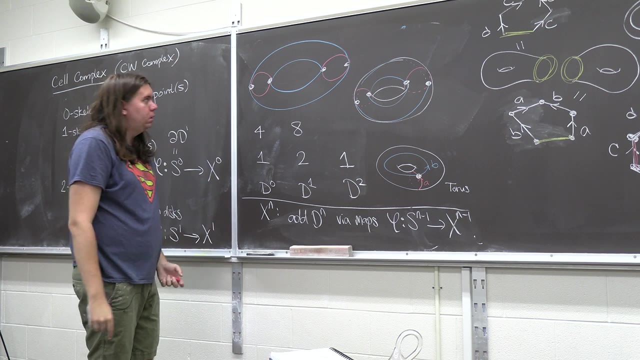 And maybe this will make it a little bit clearer. So what we have done is we've built this, We've built this wire mesh- right, This is the one skeleton. It's your wire mesh. And now how do you glue on your disc? 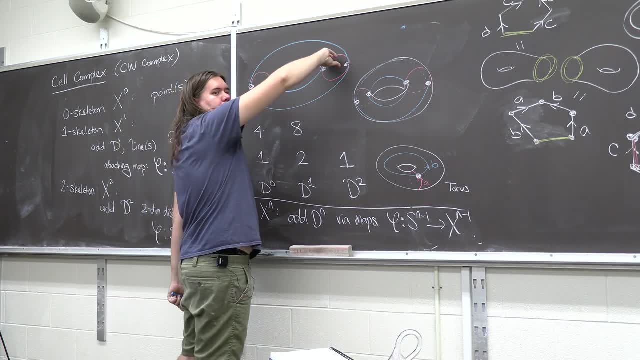 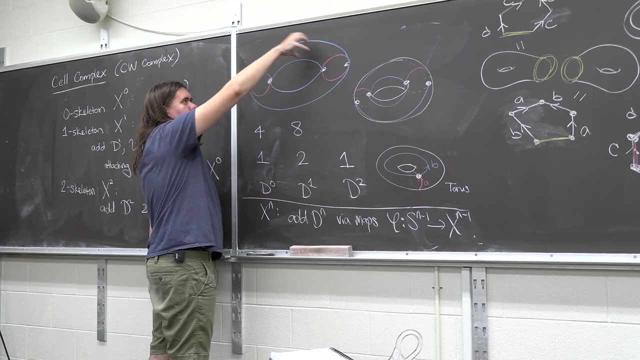 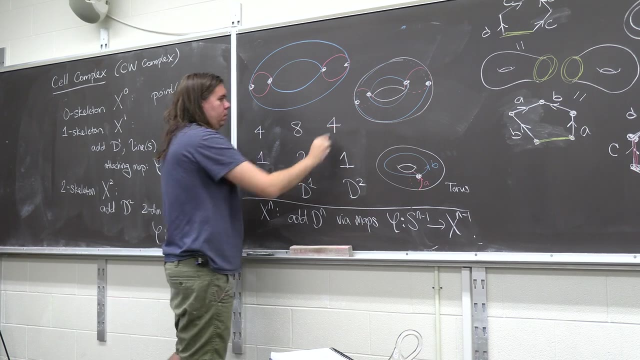 Well, one disc you glue here and along in there. That's one on top of the front, And then you have one on the bottom of the front, And then one on top in the back And one on bottom in the back. So you end up with a total of four discs. 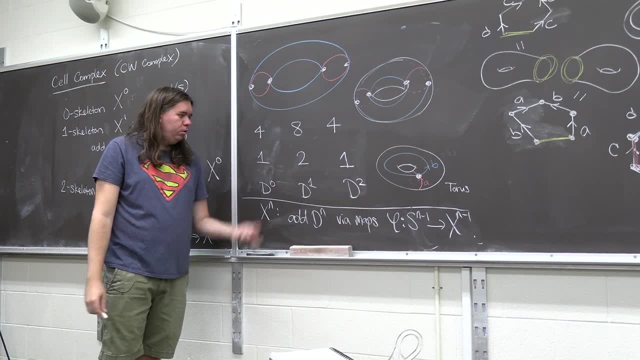 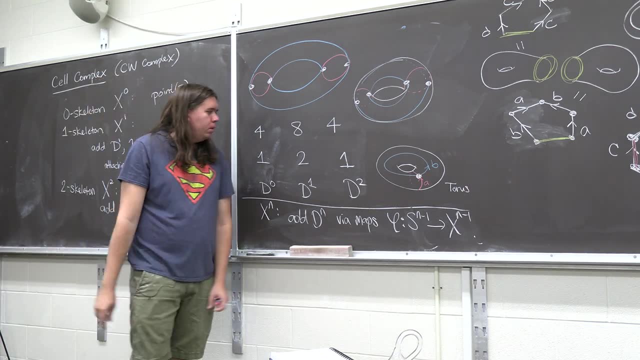 Okay, Either way, you can build a torus. So now you tell me those who have like seen anything related to topology before. what can we do with these numbers? What does this remind you of? Ah, the Euler characteristic. 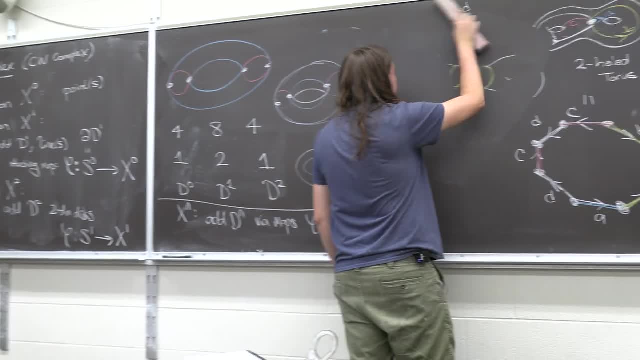 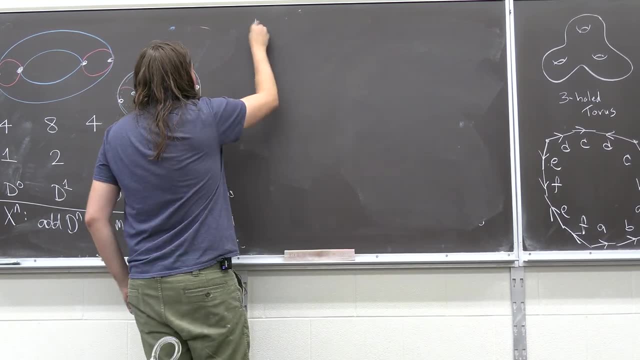 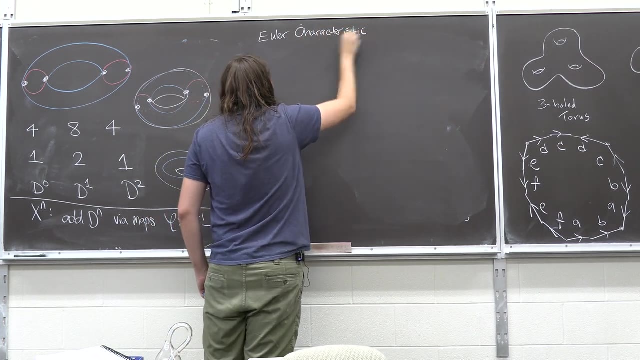 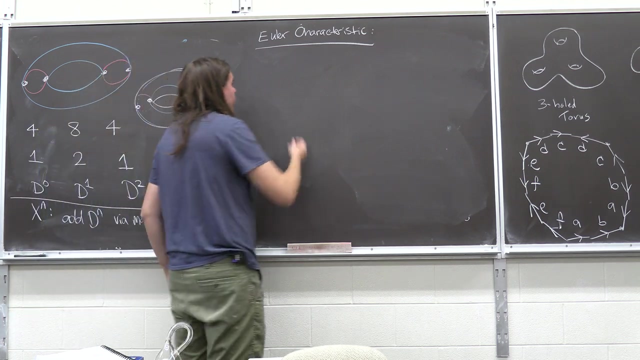 So the Euler characteristic you've probably seen defined as something like the Euler characteristic. So you may have seen this in graph theory for planar graphs, or you may have seen this with polyhedron right, Where you had some formula like the Euler characteristic denoted by the Greek letter chi. 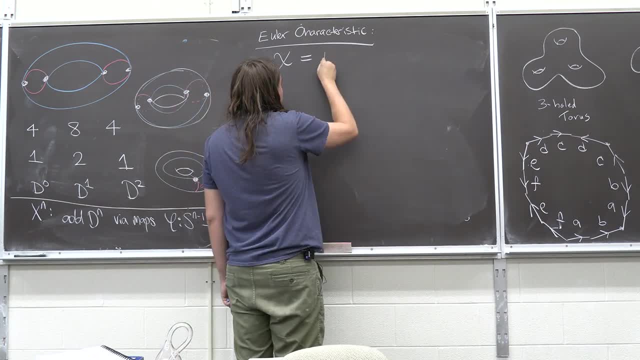 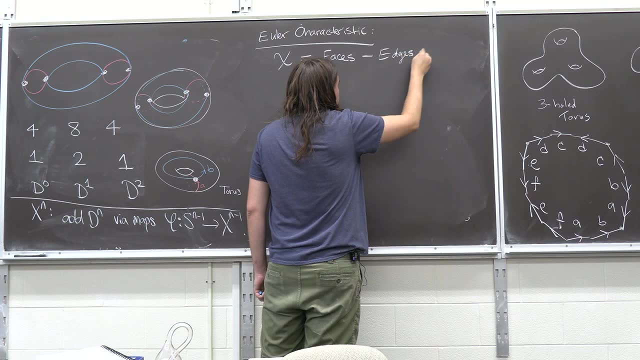 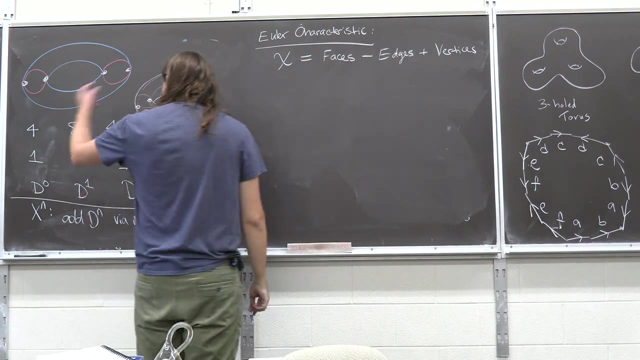 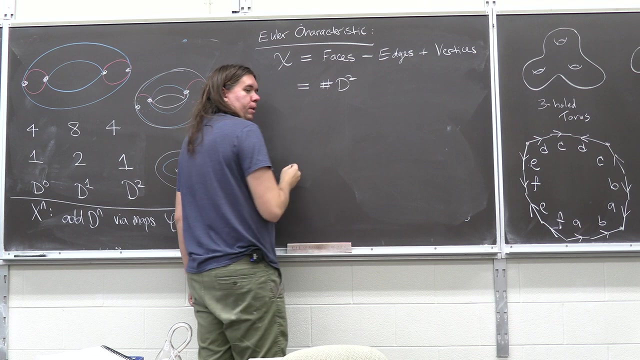 for characteristics is often calculated as something like faces: number of faces minus the number of edges, plus the number of vertices. Yeah Well, now, using this language, it's just the number of two-dimensional discs minus in your two-skeleton. 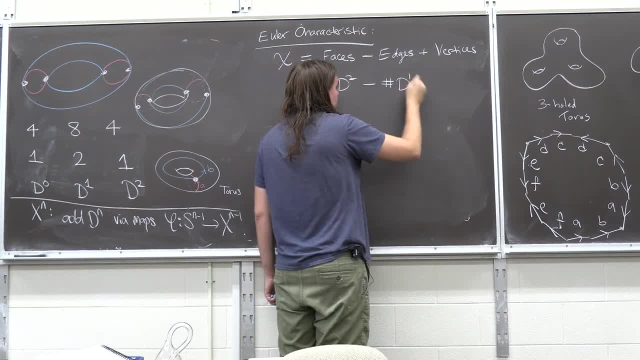 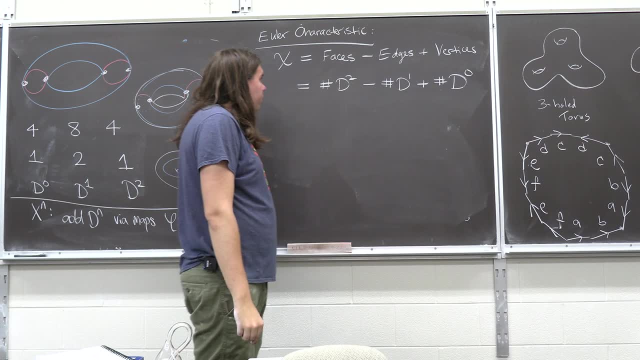 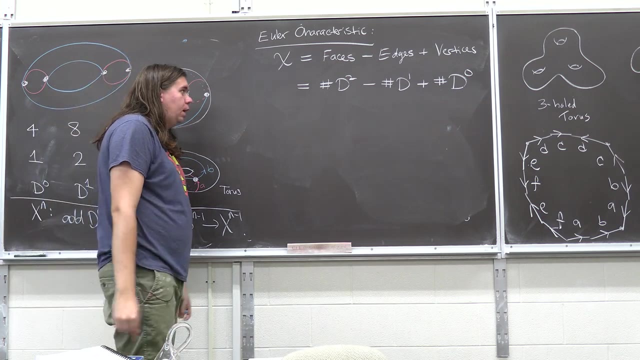 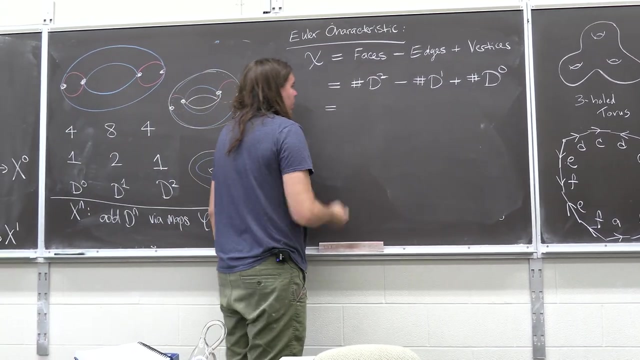 minus your number of one-dimensional discs, plus the number of zero-dimensional discs. But this is only if I have a two-dimensional cell complex, right, I could be n-dimensional. In that case you just continue the alternating sum Or, in general, you put a plus in front of all the even-dimensional ones. 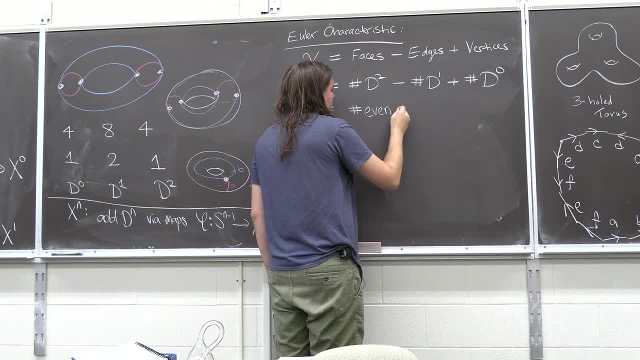 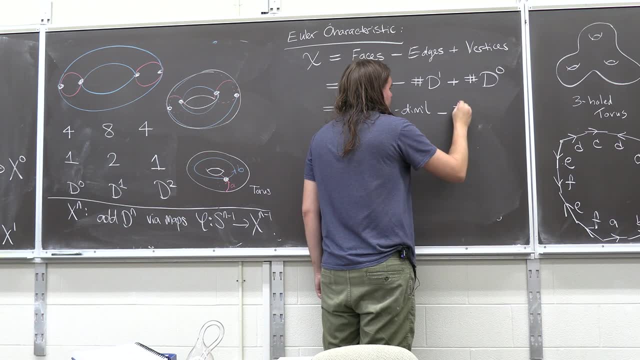 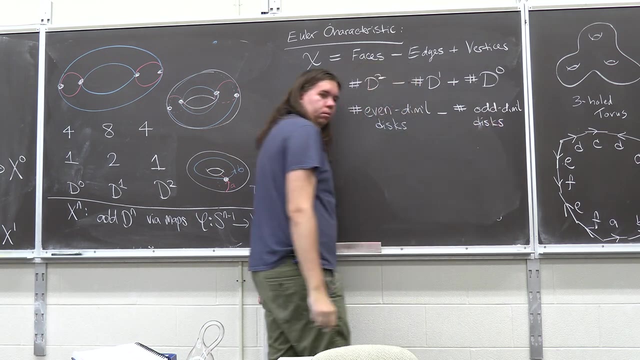 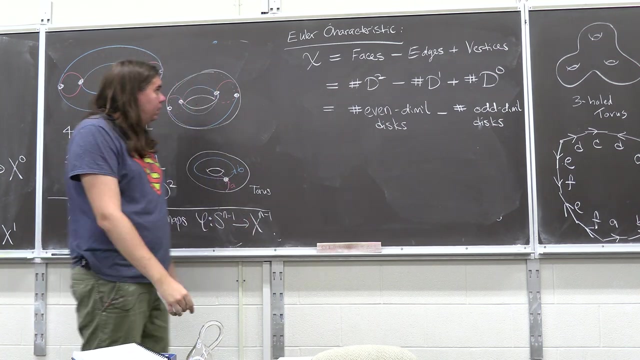 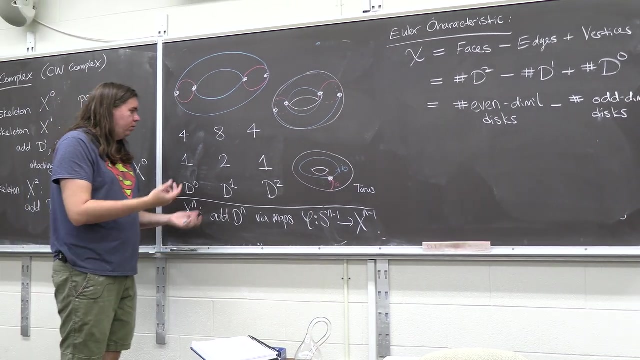 So it's the number of even-dimensional disc minus the number of odd-dimensional disc. So now you can define it for arbitrarily many dimensions. And the nice thing with the Euler characteristic is that, independent of how you choose to construct your object, the Euler characteristic is the same. 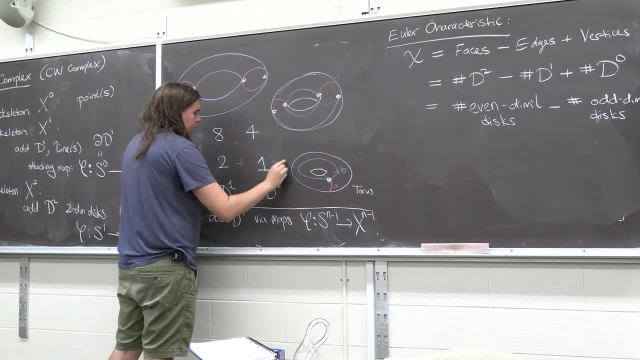 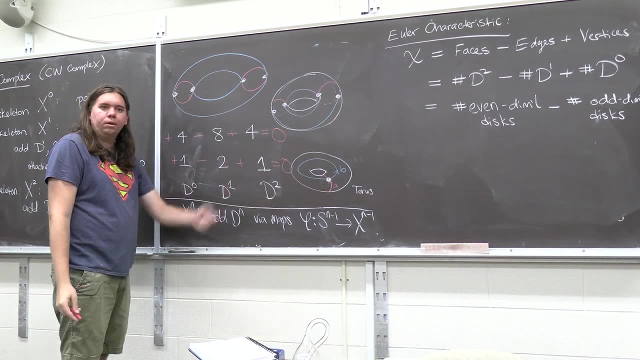 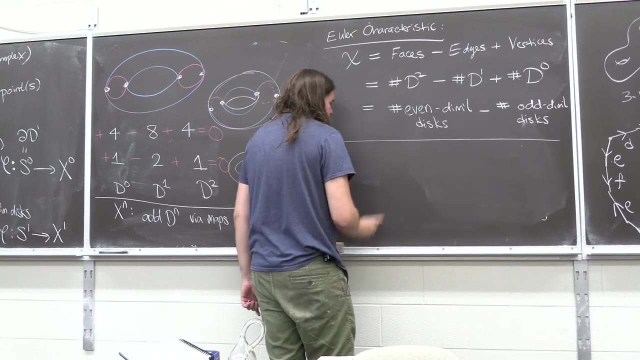 If I take the alternating sum of this, I get zero. Or if take the alternating sum of this guy above, I get zero. The Euler characteristic of the torus is zero, By way of contrast. In contrast, someone tell me what is the Euler characteristic of the sphere, the 2-sphere? 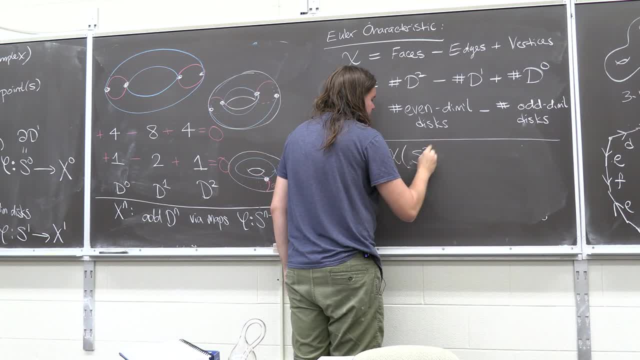 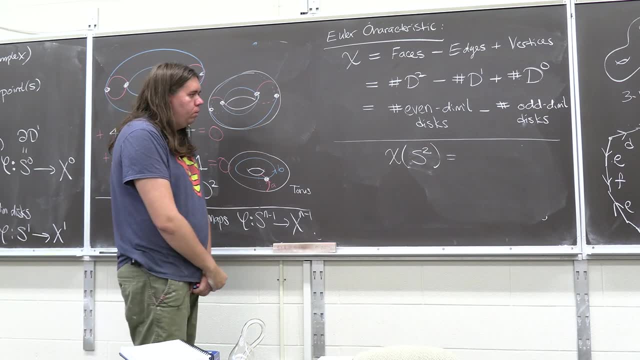 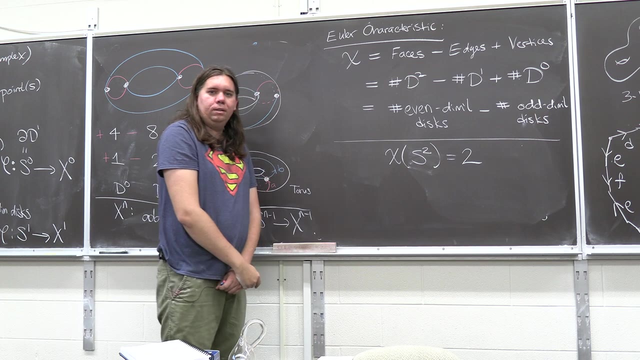 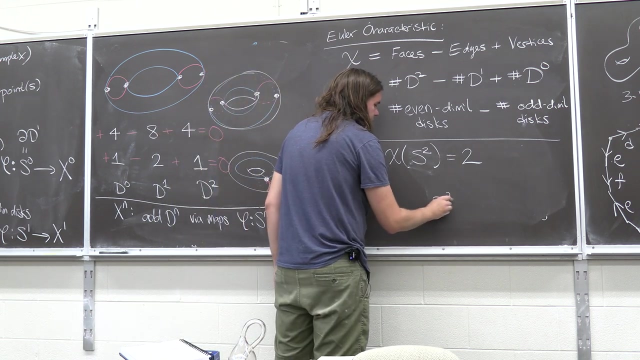 So I'm asking for the Euler characteristic- I'll just write it here- of S2.. Why is it 2?? You're right. Can we see it here? Why is it 2?? Well, how do you build S2?? There's a couple of ways you can build S2.. 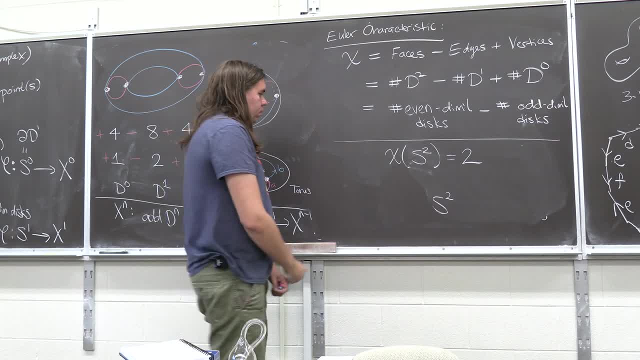 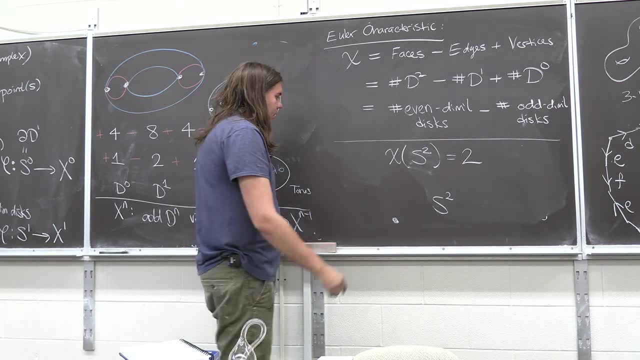 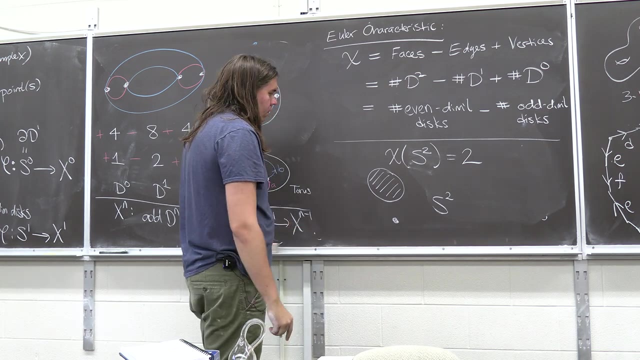 Here's the easiest way to build S2.. You just take a single point, that's your 0-skeleton, no lines for your 1-skeleton, and then a single disk for your 2-skeleton, And then the map to attach the disk. 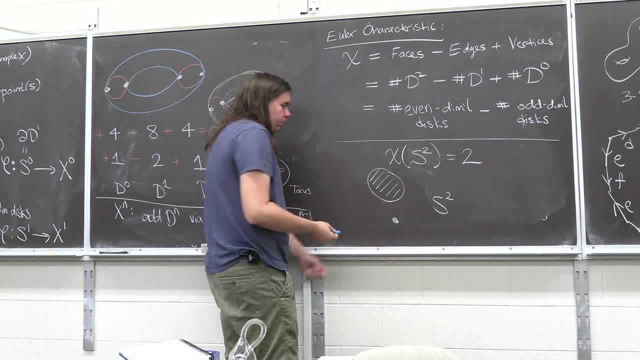 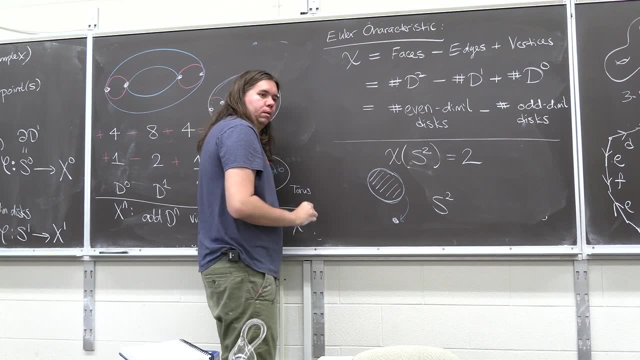 Okay, Okay To your 0-skeleton, which is also your 1-skeleton, because you're adding things to. the 1-skeleton is just the map that takes everything on the boundary of the disk and glues everything onto that point. 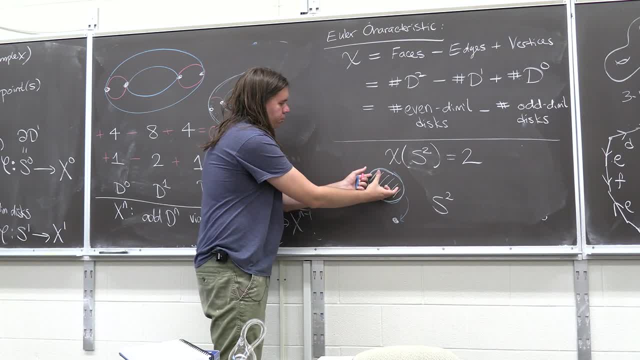 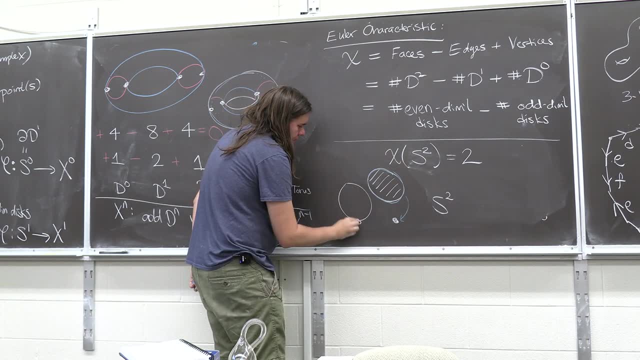 What do you do if you glue the whole boundary to that point? It's like you've bunched up all the edges together to a single point and you end up with a picture like: well, I'll put the point down here. you end up with your disk some. 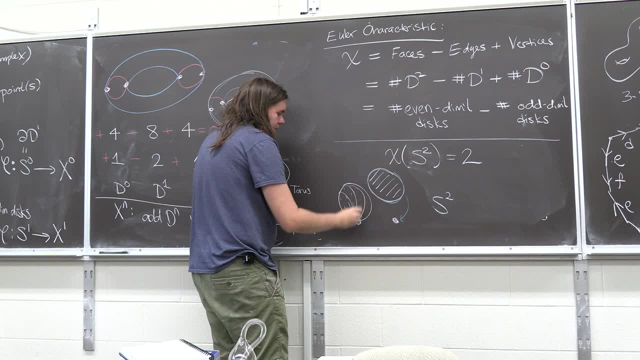 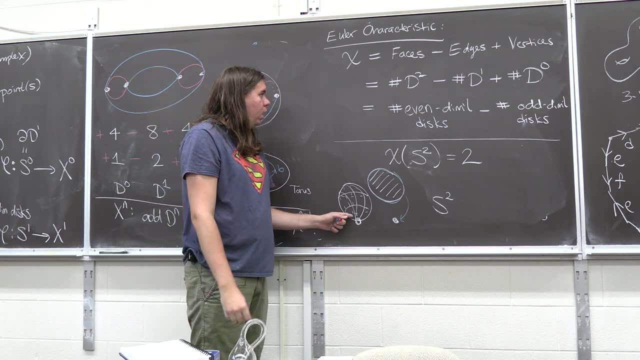 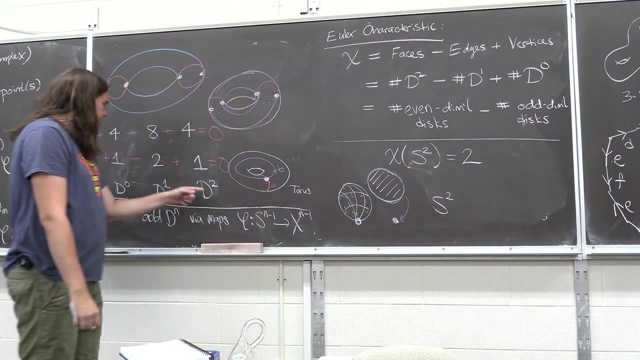 picture like this. These aren't lines, I'm just trying to show you. It has some three-dimensionality right, so you get your sphere. So it has one D2 and one D0. So when you add it up, there'll be one for D2, one for D0, and nothing in the middle. 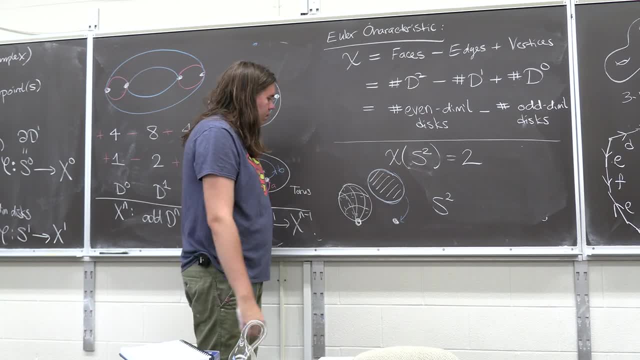 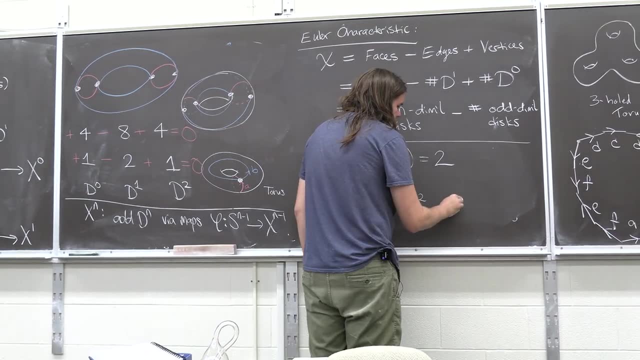 so it ends up being just one plus one for your Euler characteristic. But there's other ways you can build S2.. Another way to build S2 is lots of ways, I don't know. let's take a point and let's stick a line around it. 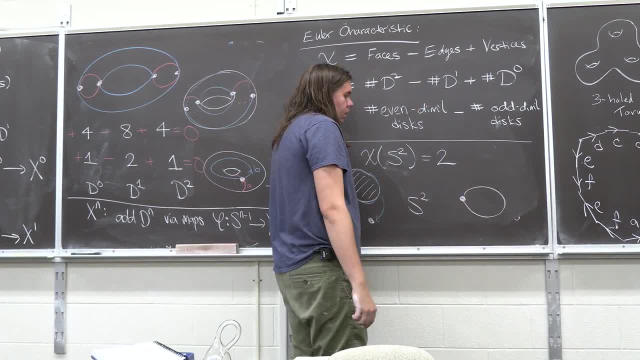 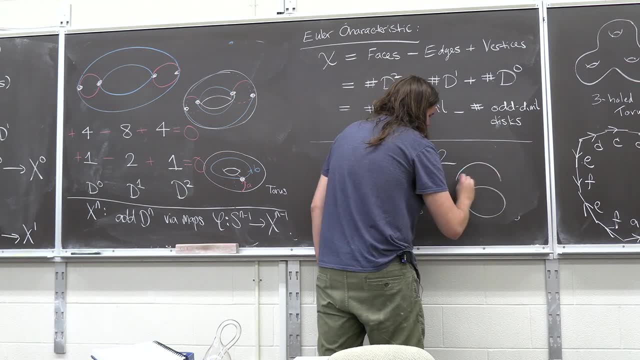 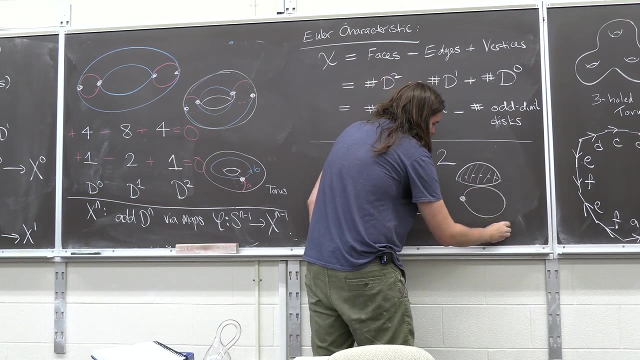 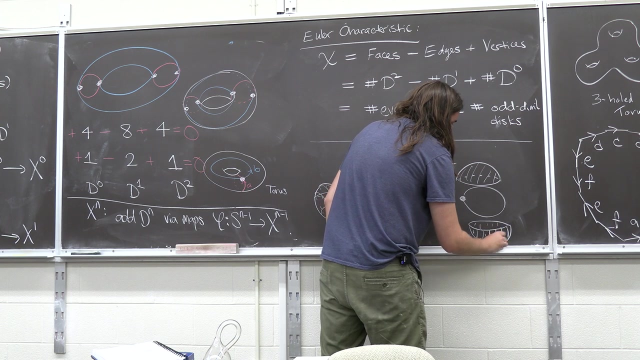 Now I have my equator. Now how many disks do I need to attach to it? Two, One on the top. so I'll glue one disk along the top to my equator and I'll glue a second disk. here's my second disk I'm going to glue. this is me trying to give it some shading. 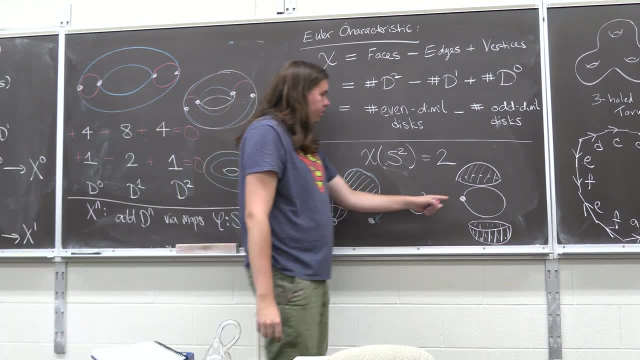 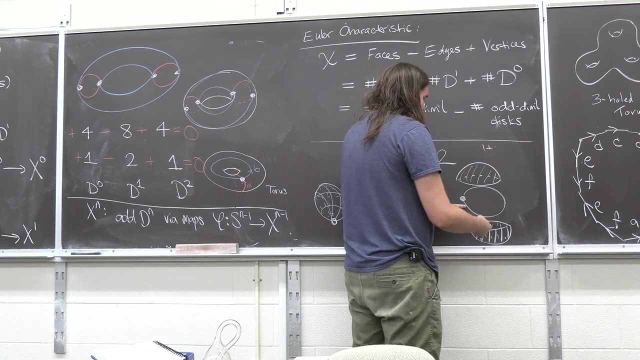 glue a second disk to the bottom, And now The number of two-dimensional points is one. the number of one-dimensional disks is lines, in this case is one. so it's minus one plus the number of disks. I added two disks for 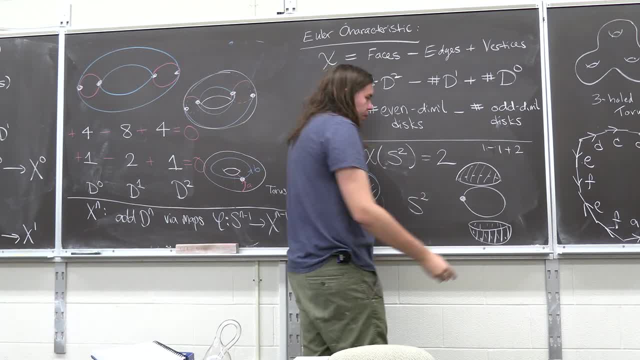 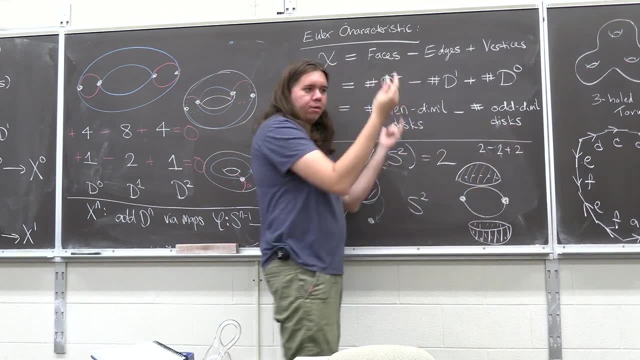 the two hemispheres still comes out to be two. Or if you started with two points, you now have two lines and two hemispheres. you know, however you build it, the Euler characteristic stays the same. So that's it. 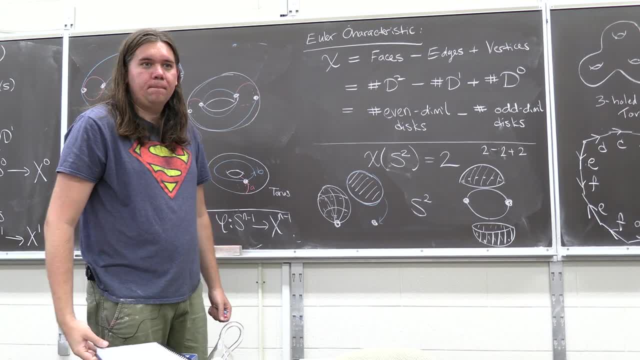 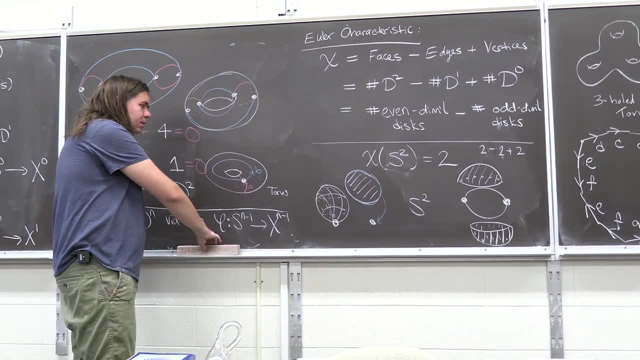 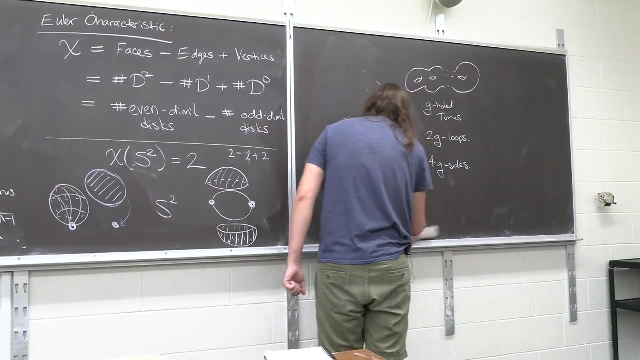 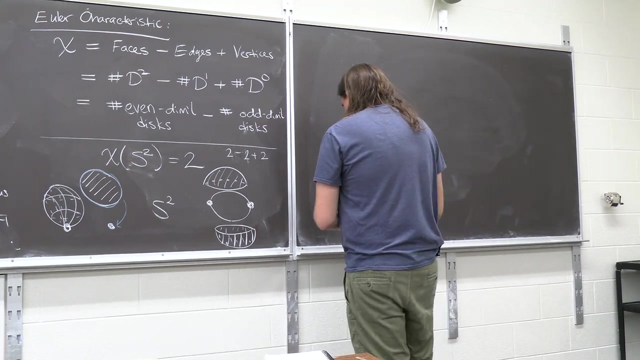 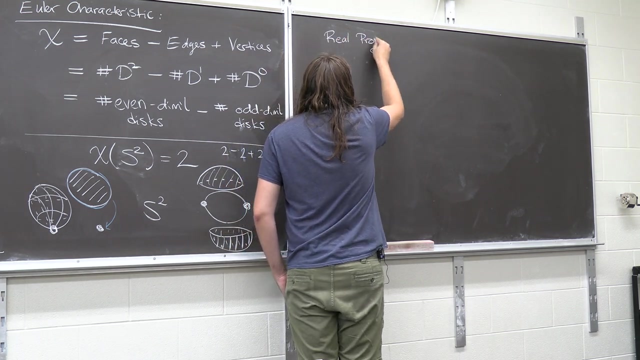 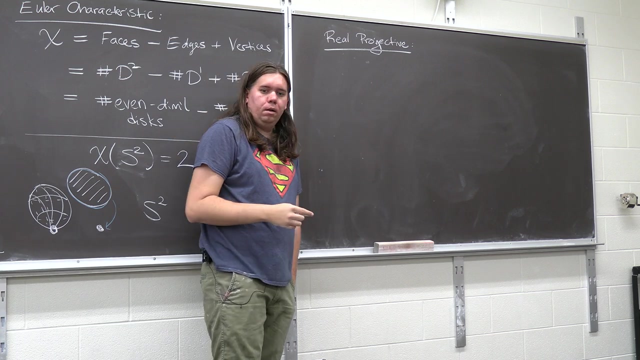 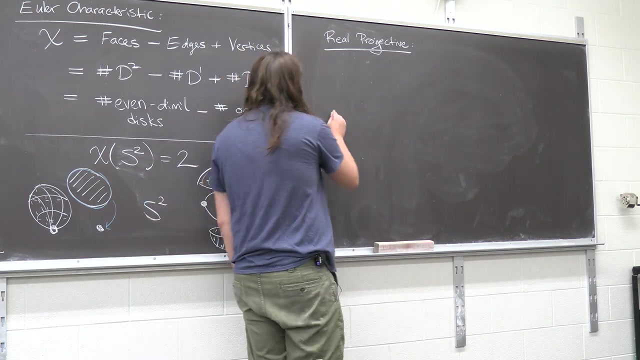 Thanks for watching. See you next time. Okay, I think we're getting a pretty good grasp for how we build up spaces from disk. Let's look at a more complicated space. Let's try to understand real projective space. So we began with RP1, let's say: 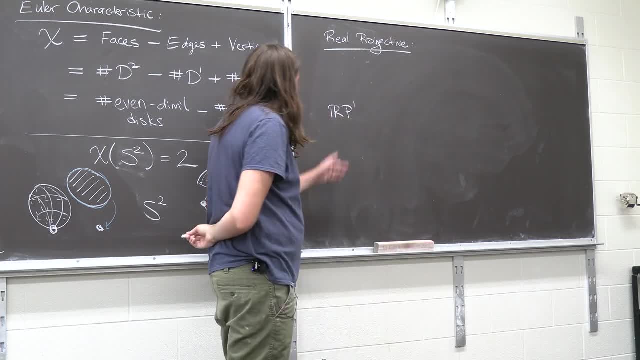 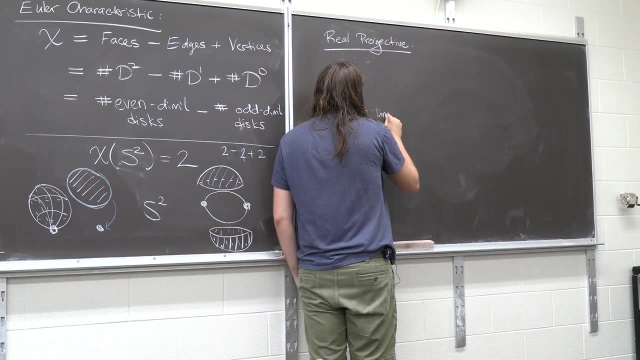 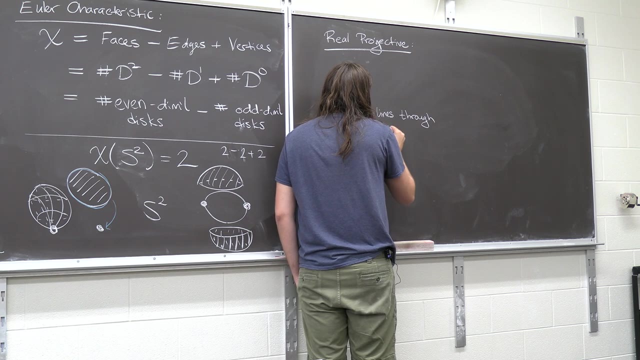 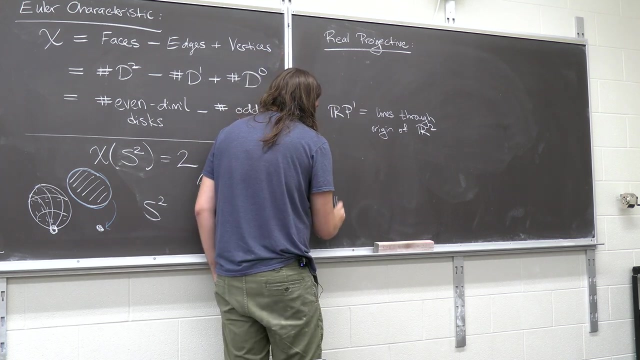 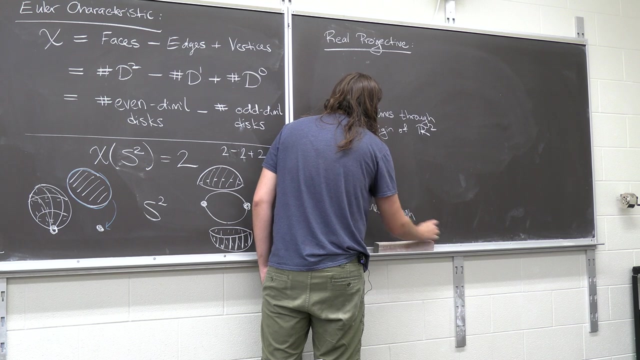 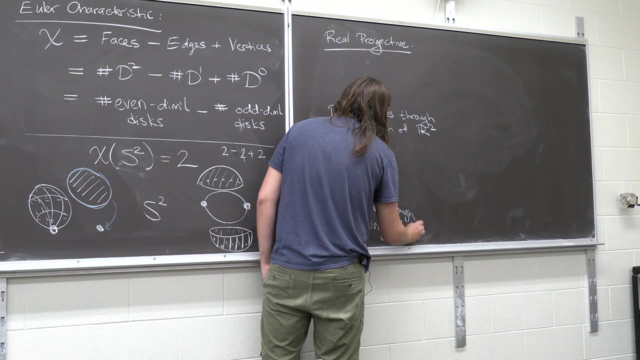 RP1.. So do you know the definition of RP1?? This is the set of lines through the origin of the set of lines. Okay, Okay, Let's try that. Okay, so the set of lines of r2.. In general, rpn is just your set of lines through the origin of rn, plus one. 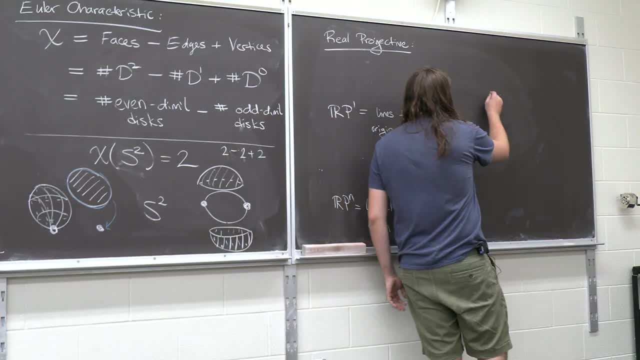 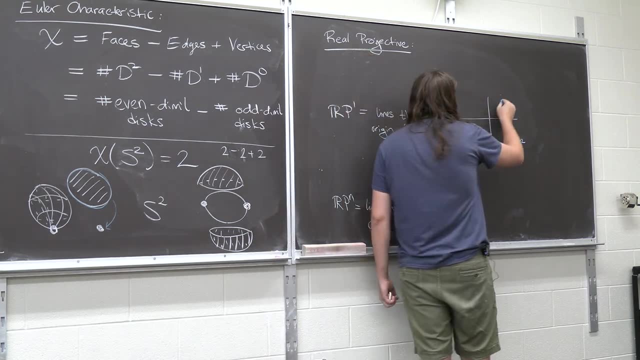 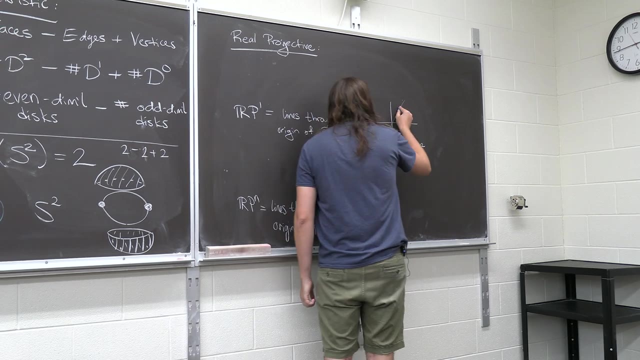 Okay, so let's try to understand this a little bit. So I have r2, but each line in r2 corresponds to a point of rp1.. Kind of weird. This is a point, and then, very close by, is this other point, and then this other point, and so forth. These are each points. 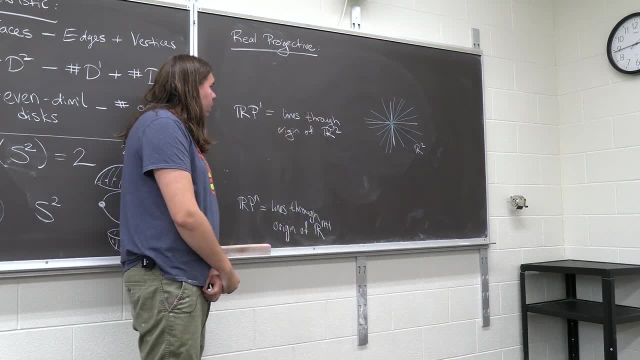 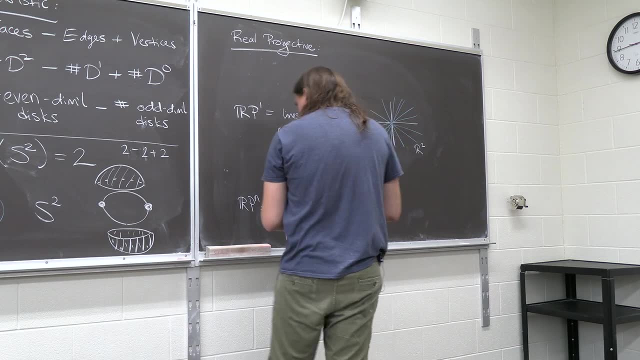 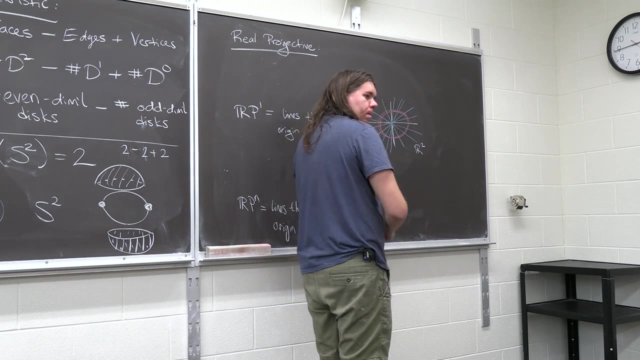 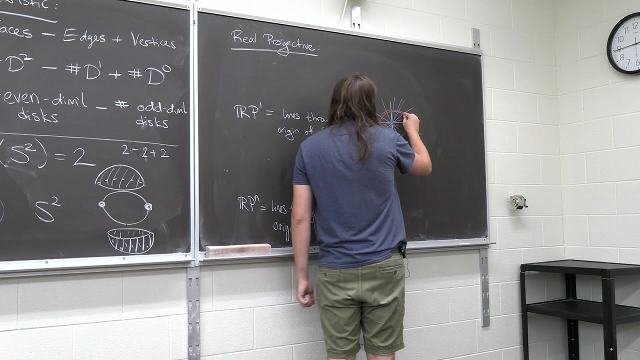 So there's another way you can think about this. Another way to think about rp2 is you could say, okay, well, each of these lines you could think of by where it hits the unit circle, And then you can say: it's points on the unit circle, except this point and its antipodal point. 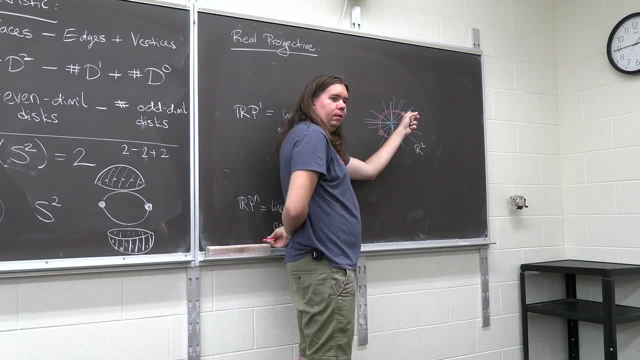 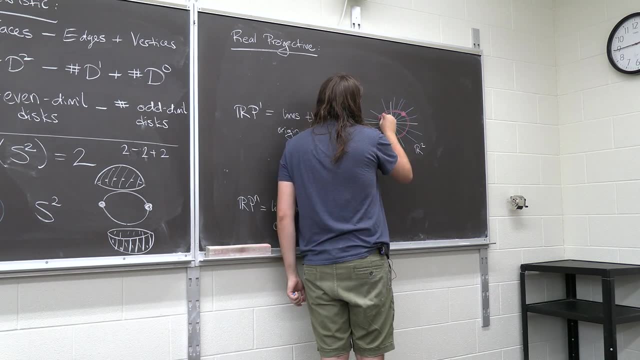 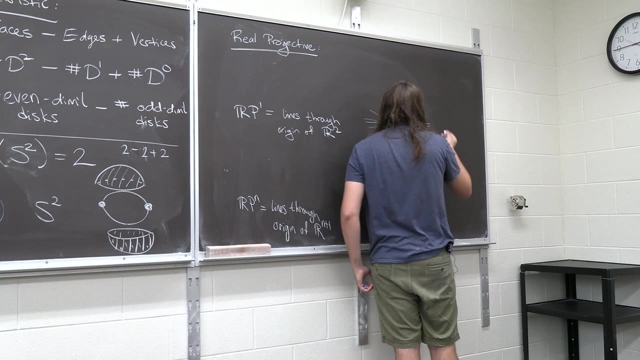 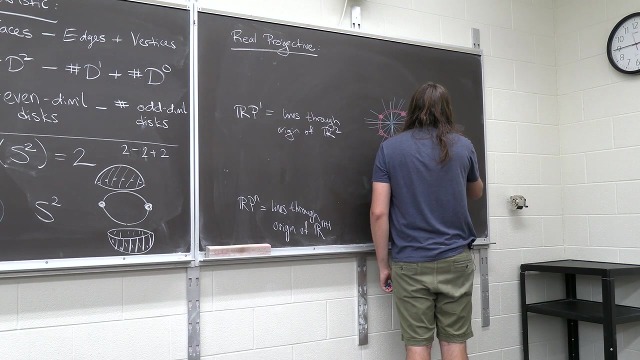 its point on the opposite side. both represent the same line so therefore it represents the same point. So it's points on the unit circle where you make the opposite points antipodal points identified. So I could say this is s1, identifying antipodal points. 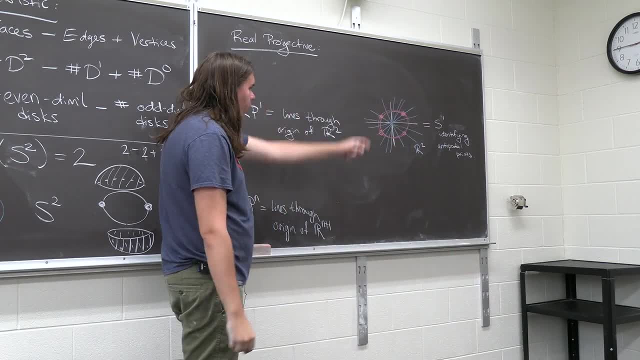 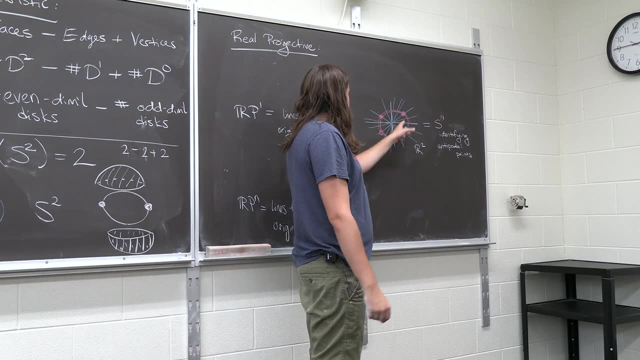 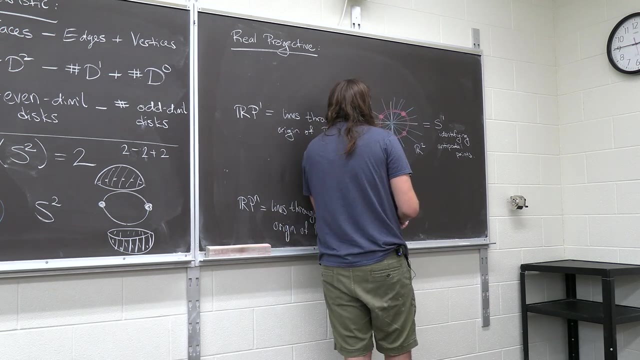 Antipodal, which means opposite, Opposite pole antipodal. But if all the points on bottom identified at the point on top? now this is redundant. so we might as well just think about this as the top half, the top hemisphere. 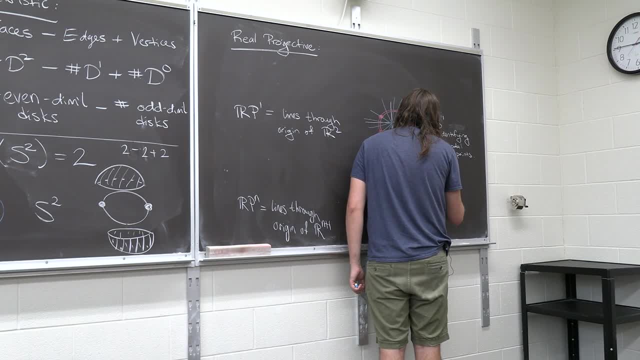 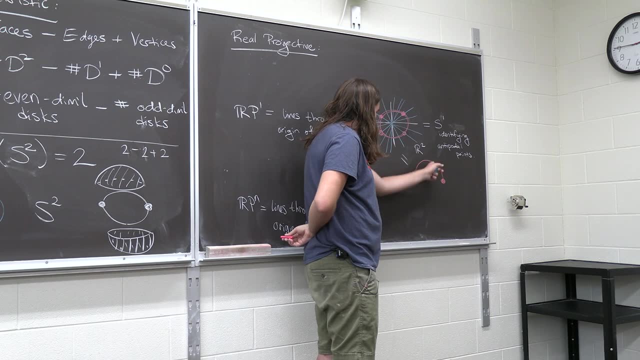 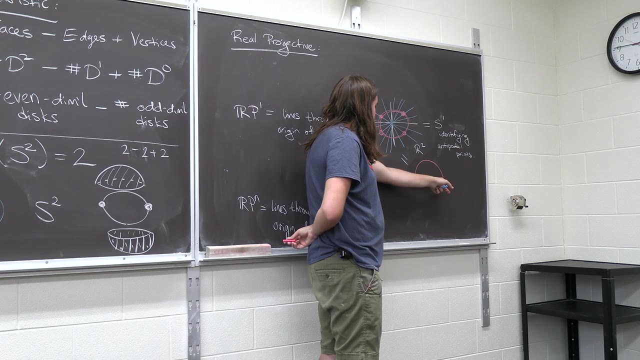 where this point on the right is identified with this point on the left. All these points on top are identified as something on bottom. so we can just collapse them all Now we just have the top arc, top half of the circle, but we need to remember that this point on the right is going to be glued. 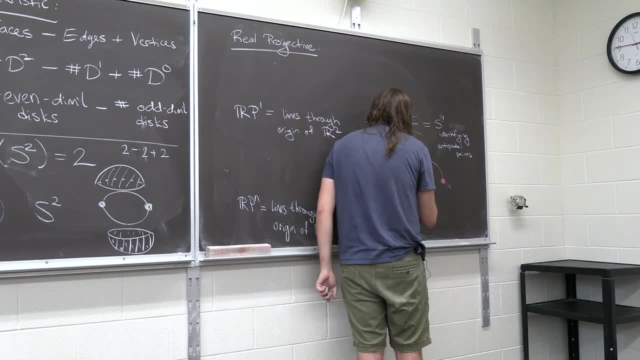 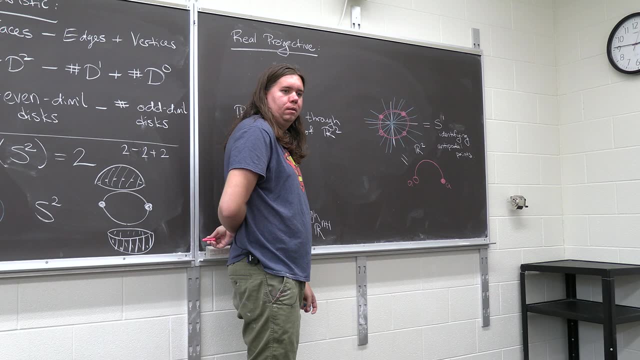 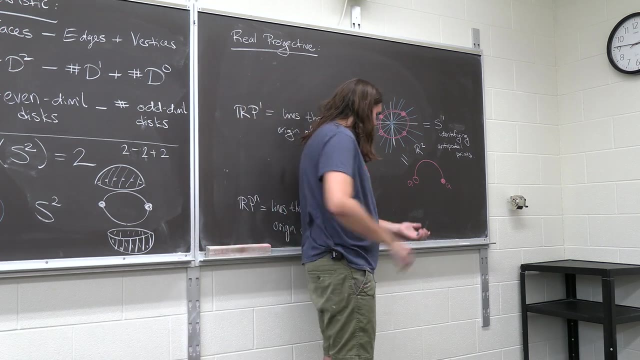 to this point on the left, Maybe I'll just put like an a next to both of them. so remember, these get glued together. What is that? Yeah, It's just s1.. It's just s1.. It's just s1.. 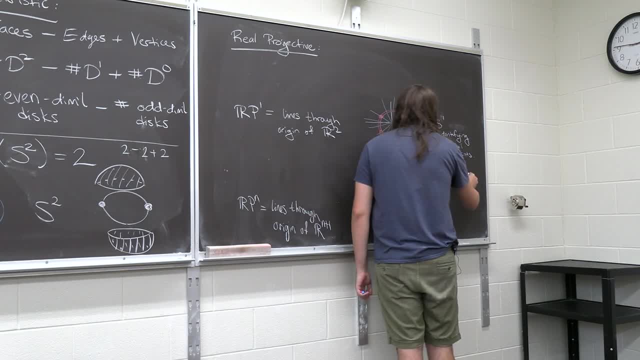 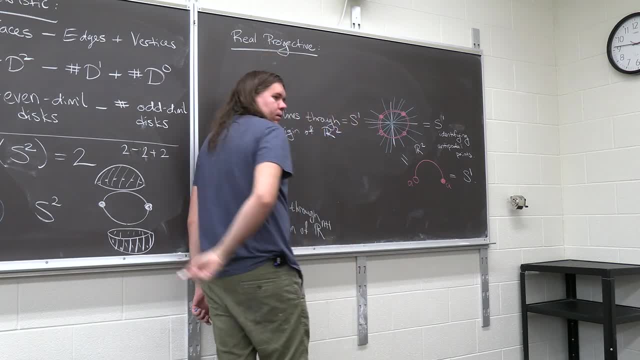 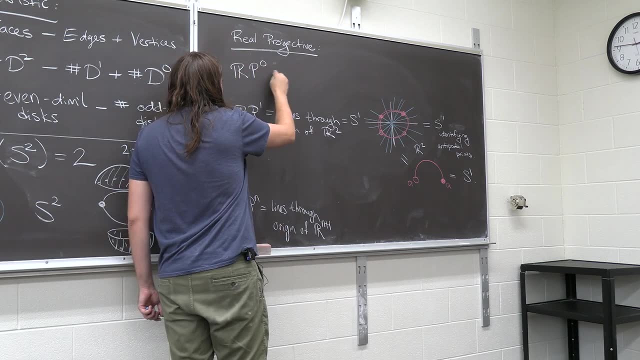 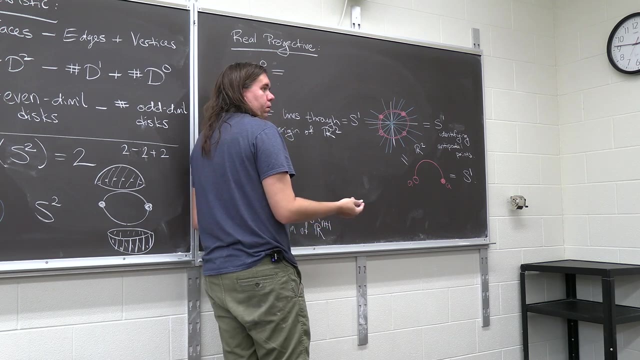 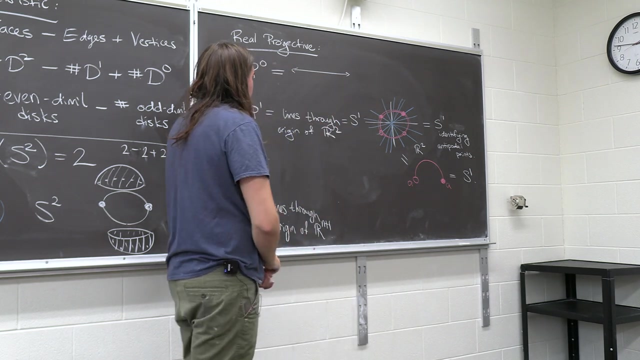 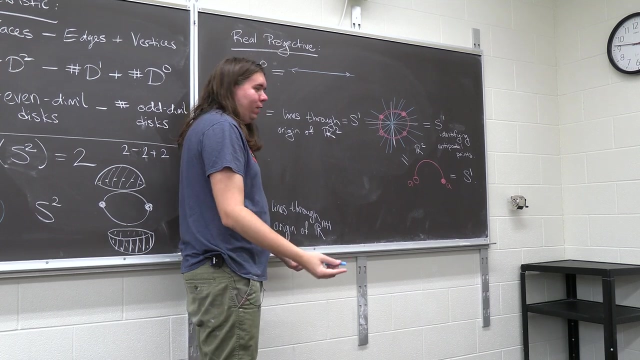 So rp1 is just s1.. Okay, how about rp0?? Now, instead of lines passing through r2, it's going to be lines passing through r1.. So lines passing through r2.. Well, there's just one of those lines, right? so it's just one line. so this itself is just. 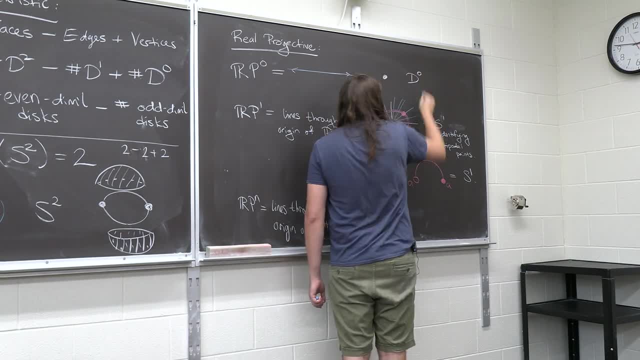 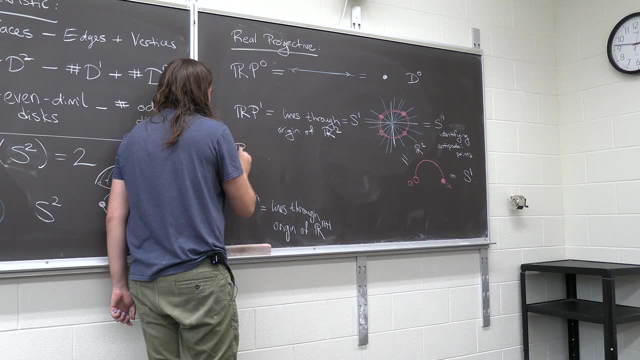 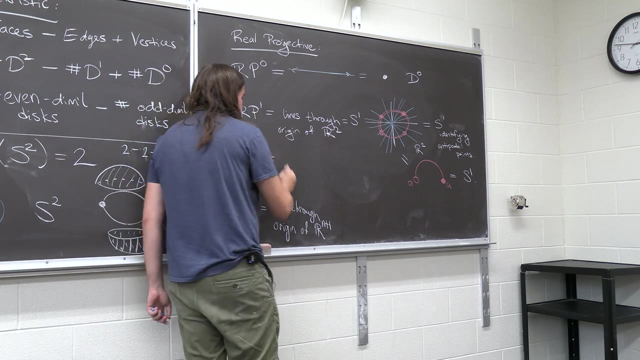 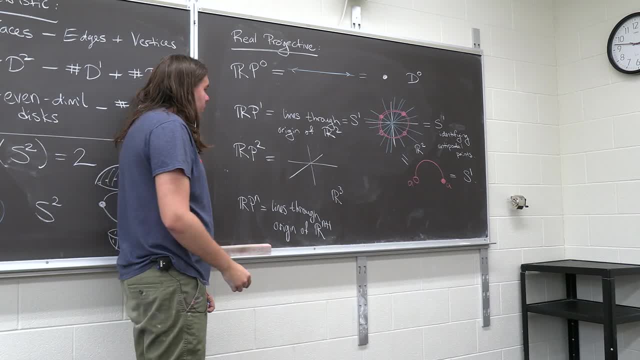 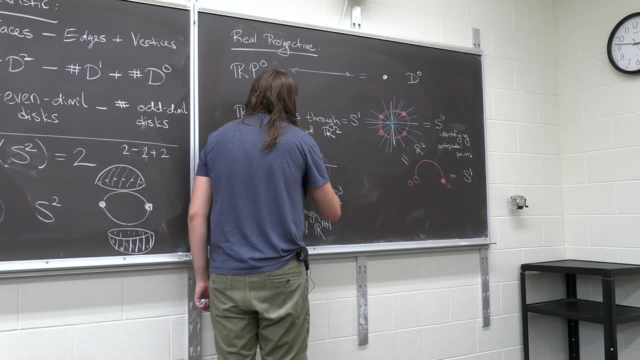 It's just s1.. So we have all these different lines passing through r3.. But instead of thinking about the whole line, we'll just think about where the lines hit the unit sphere, And each line will hit the unit sphere in two locations. 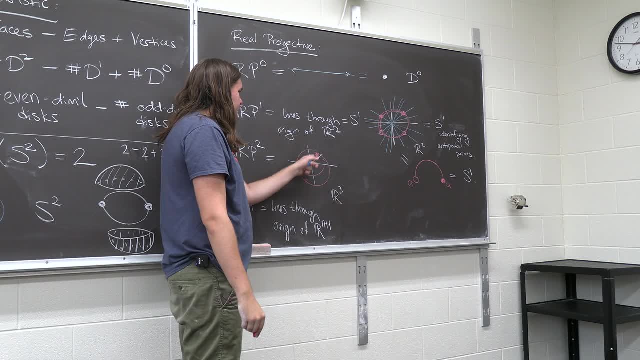 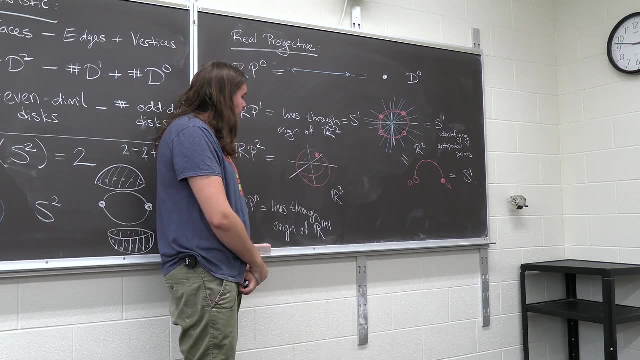 antipodal points. So we need to glue together antipodal points of the unit sphere? right, But if we're gluing together antipodal points of the unit sphere, then we can just think of the bottom sphere as being glued to the top. 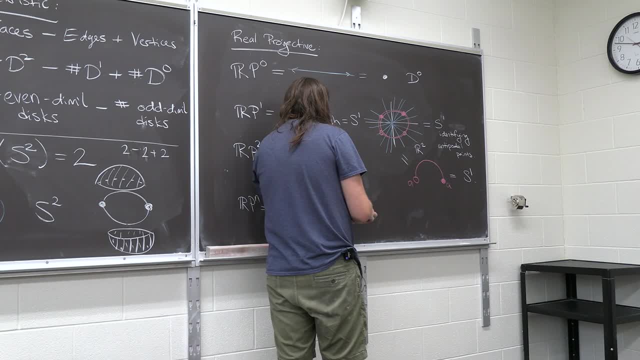 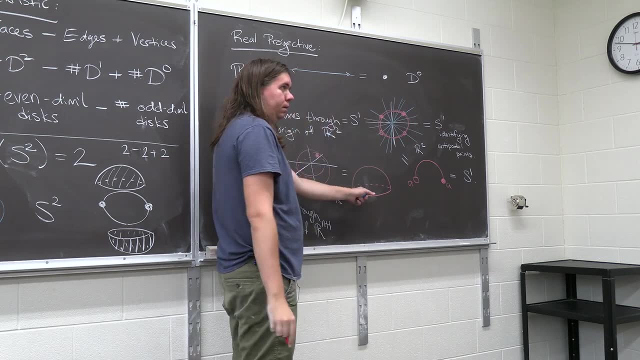 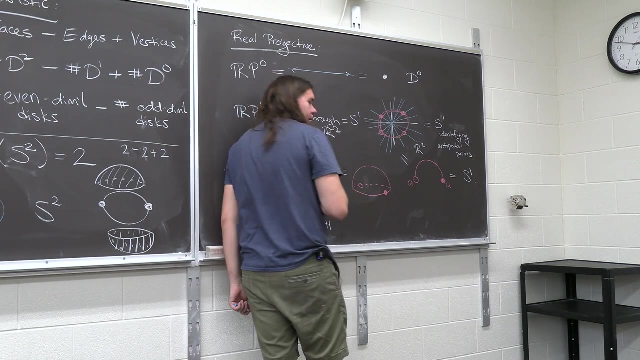 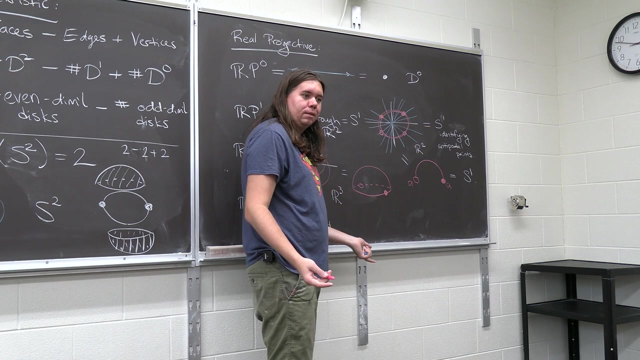 So we really only need to keep track of the top hemisphere. Except along the boundary, you still have antipodal points being identified, right? Ah, so the boundary is a circle with opposite points identified. What is that? Well, we just talked about that. 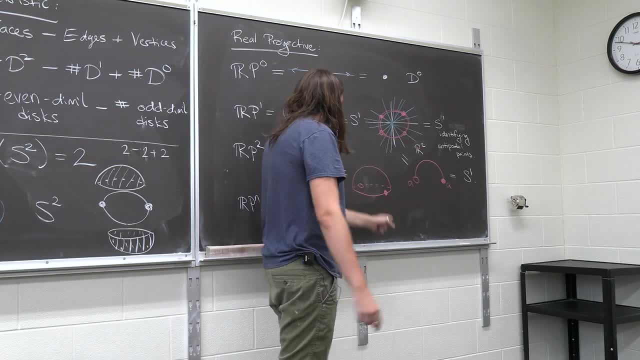 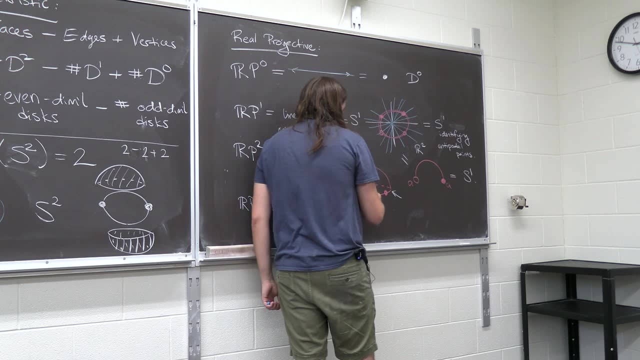 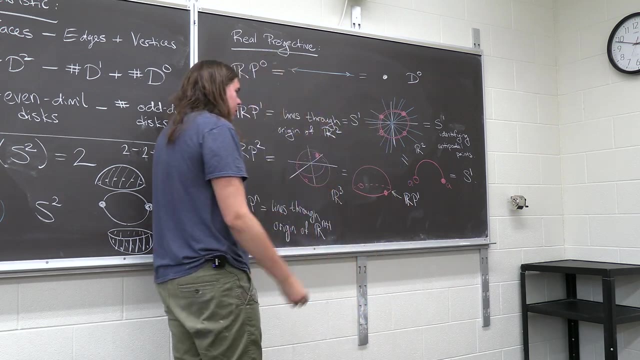 A circle with opposite points identified is s1.. So the boundary itself is s1.. But what I want to point out is that this boundary is s1, but that means it's also rp1.. So let's notice what we had to do. 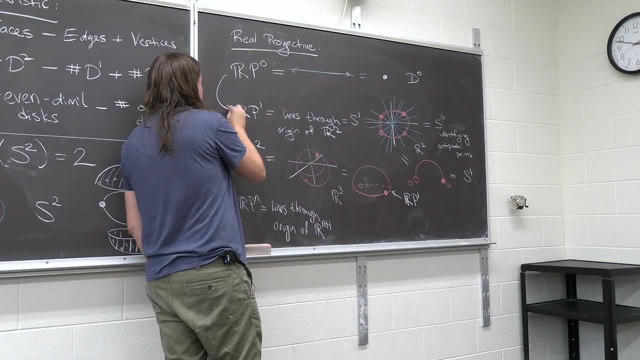 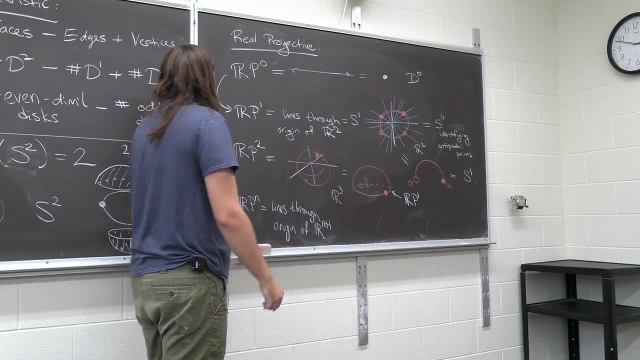 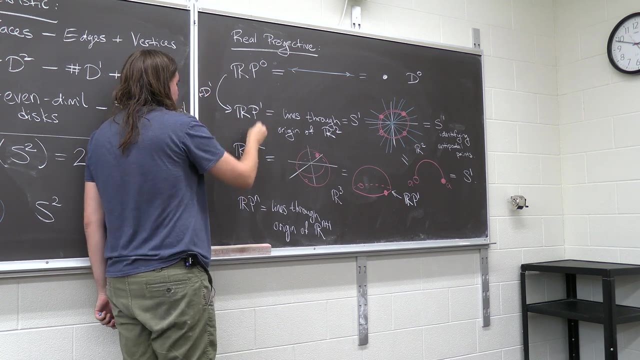 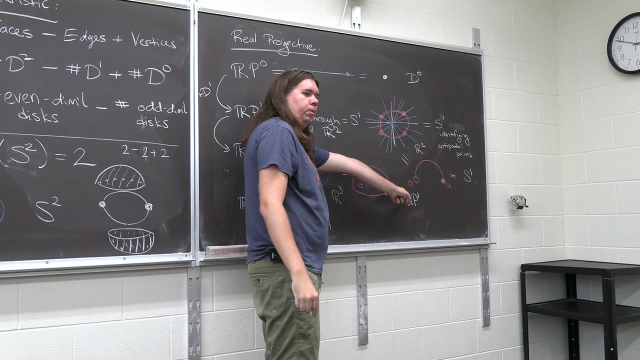 rp0 was just a point, rp1 was a line glued to that point. So to move from rp0 to rp1, we just added a copy of a line, We just added a d1.. To move from rp1 to rp2, we had a disk that was glued to. the boundary of it was rp1.. 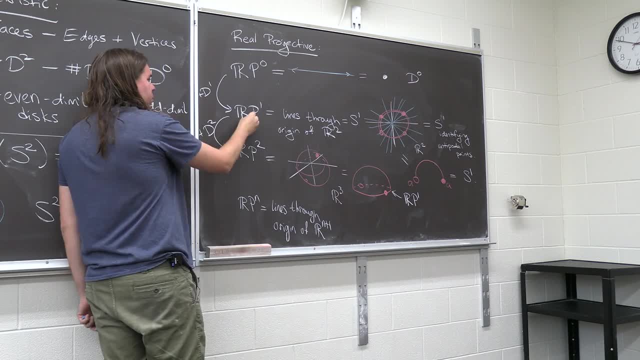 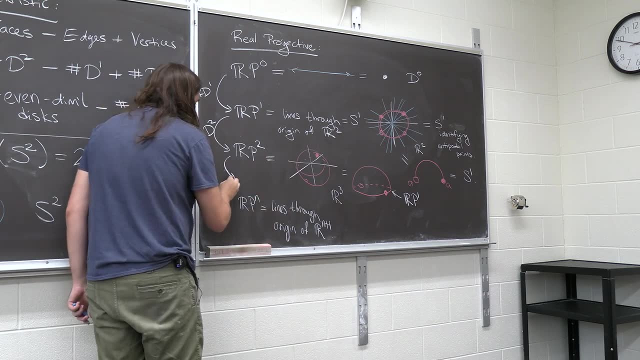 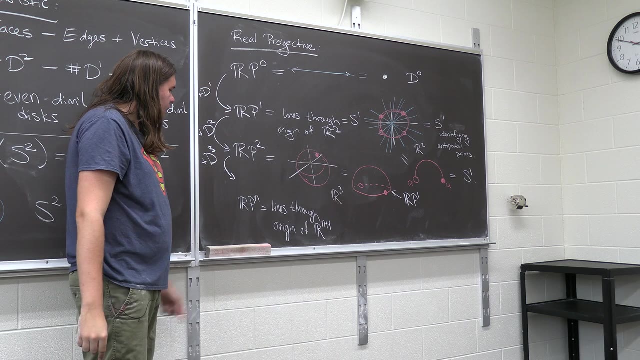 So we just took a disk d2, and glued it onto rp1.. And if you keep thinking about how you build it up each step, I want to argue at each step. you're just adding a copy of a higher dimensional disk to the previous rpn. 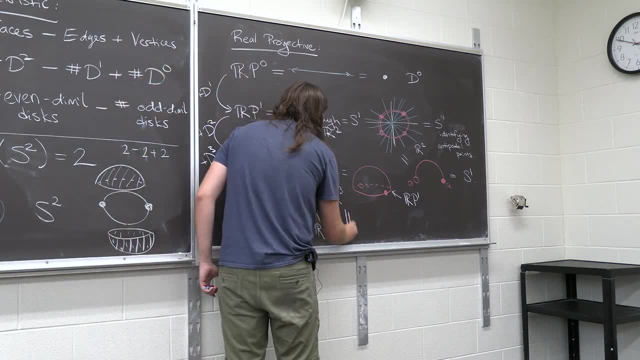 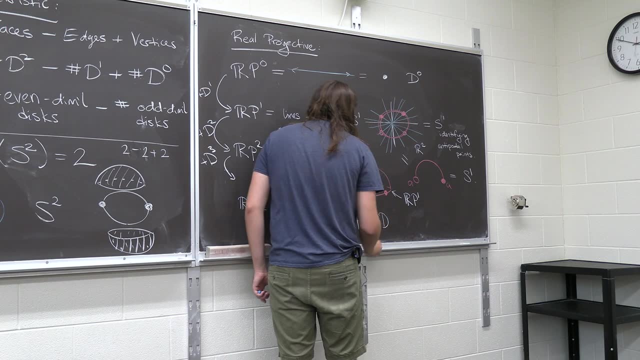 So that in general, rpn is defined recursively as just rp n minus 1, where you glued onto it a disk of dimension. let me make sure I get this right: dn, dn, dn, dn, dn, dn, dn. 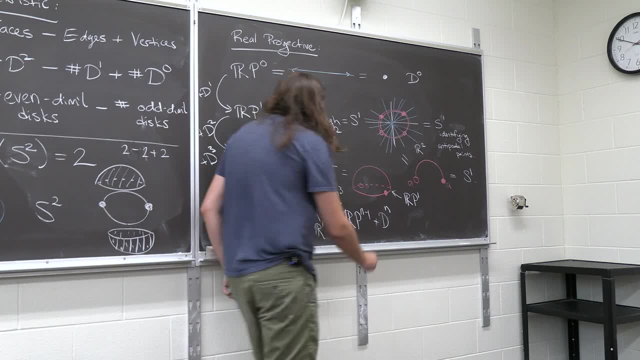 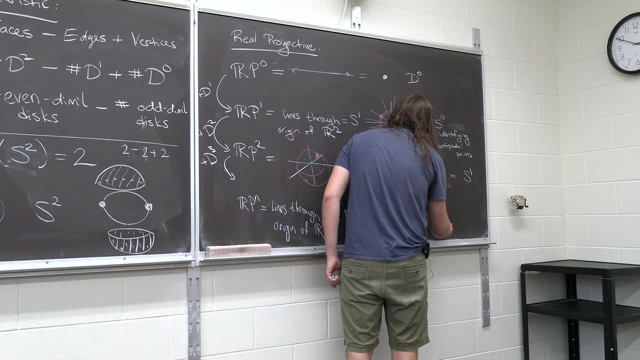 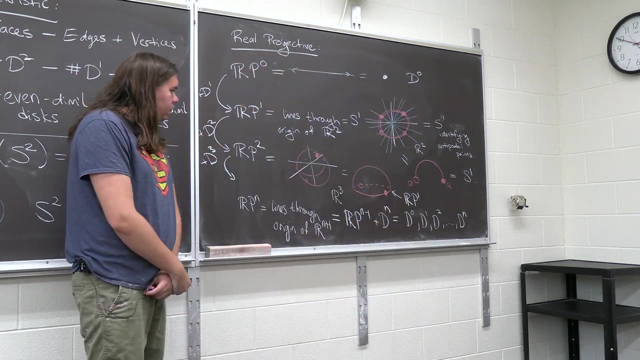 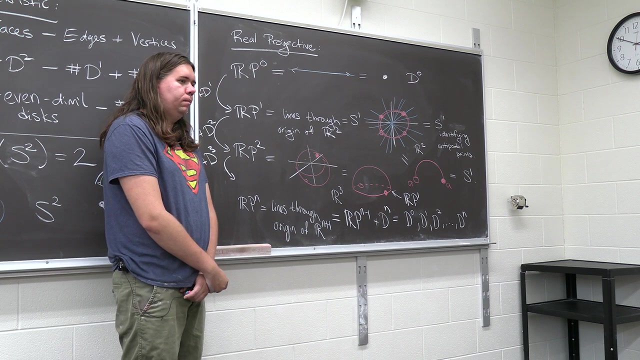 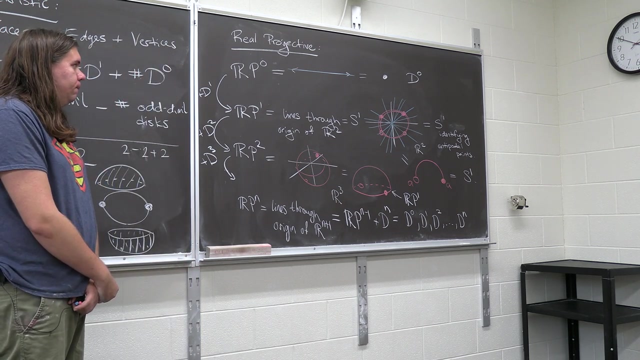 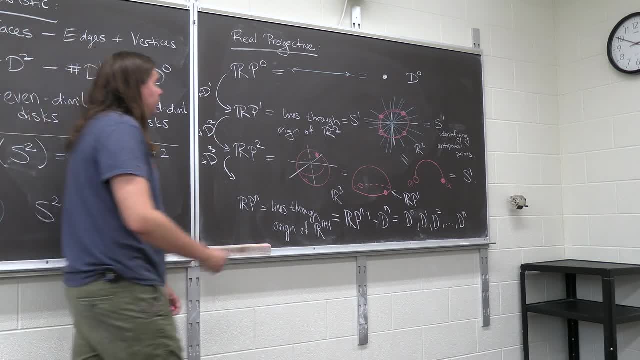 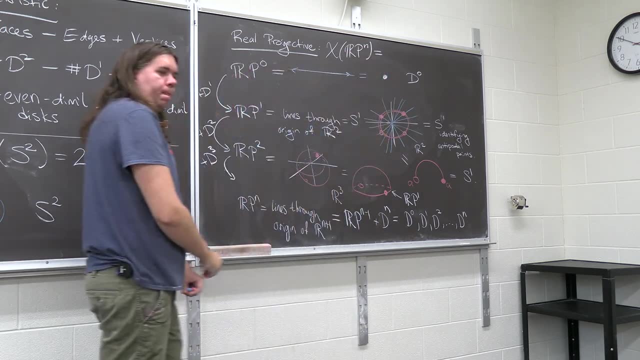 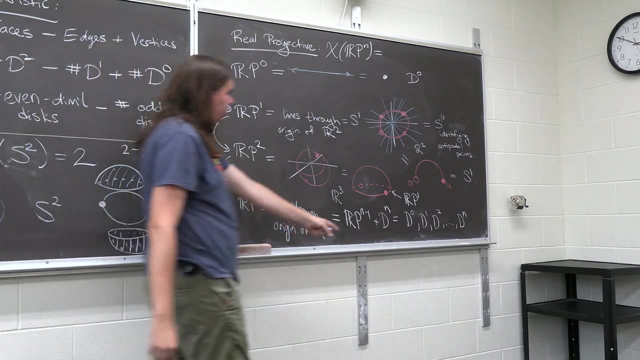 What's the Euler characteristic of rpn? What's the Euler characteristic of rpn? What's the Euler characteristic of rpn? So it depends if it's even or odd. Yeah, it depends if it's even or odd. So in the even cases you think, like you start counting, even is positive. 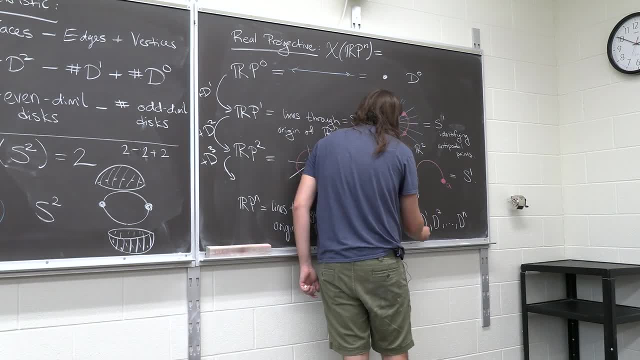 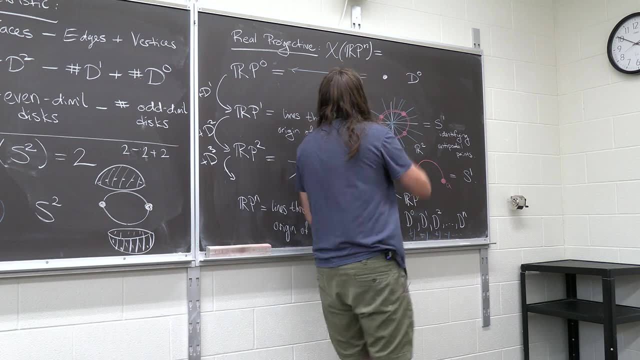 So this gives you a plus 1,, right. And then this guy gives you a minus 1, and then plus 1, and minus 1, and so forth. If n is positive is even so in the case where n. 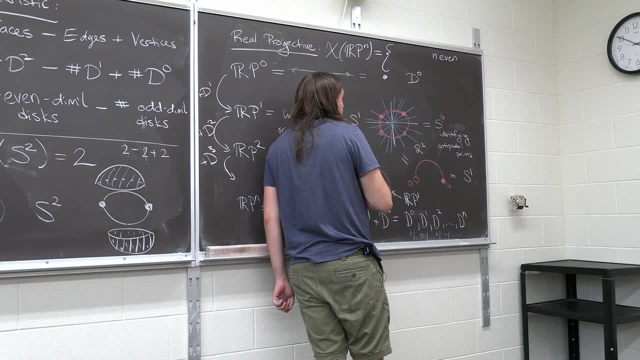 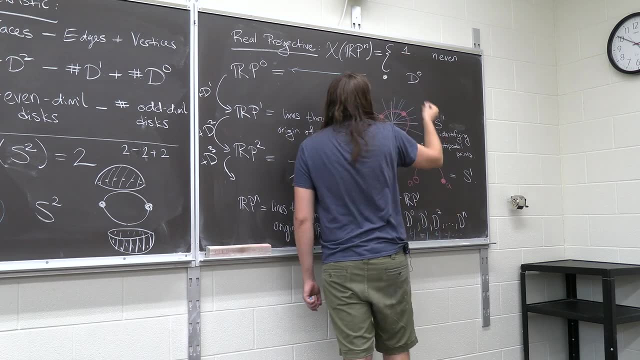 is even it's going to come out to be. if n is even, it'll be positive 1,. that's right, And if n is odd, it'll be 0. It's like that'll be 0,, that'll be 0, and so. 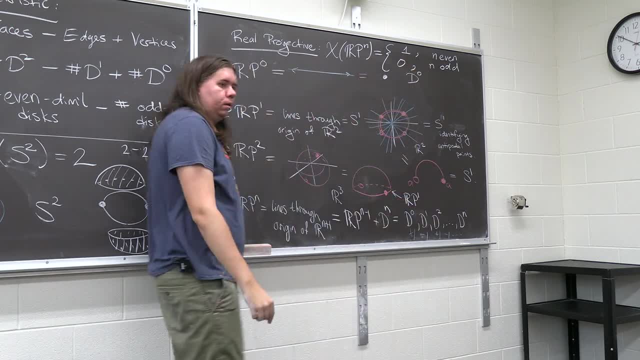 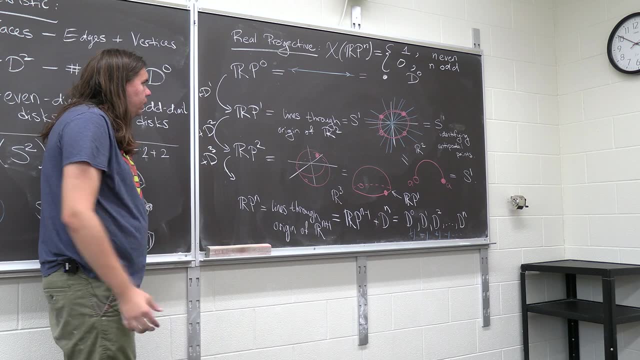 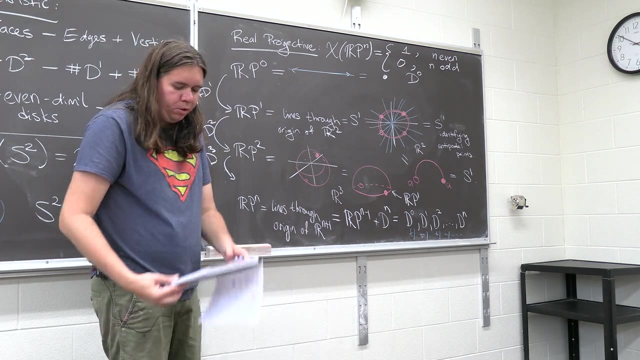 forth. Okay, Cool. So maybe this was not obvious from the definition, but we're getting a powerful technique to begin thinking about spaces, helping us visualize them. Okay, what I want to do for today, the rest of today's class- 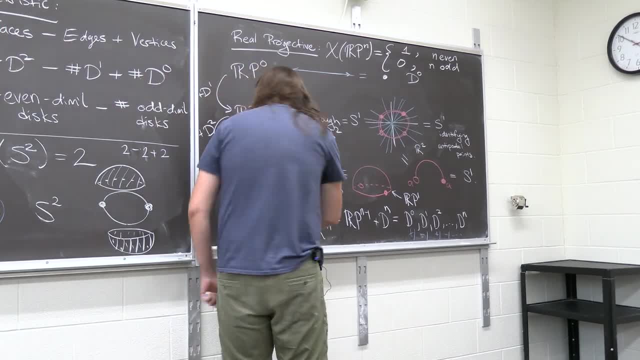 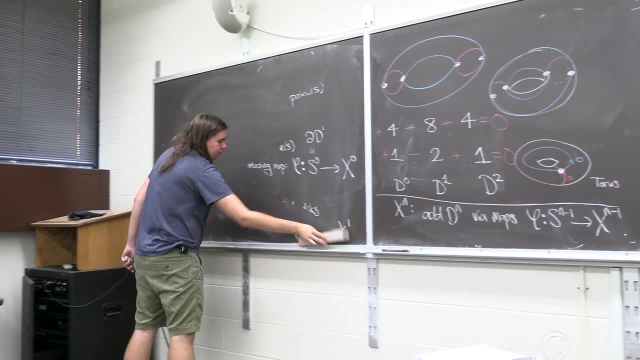 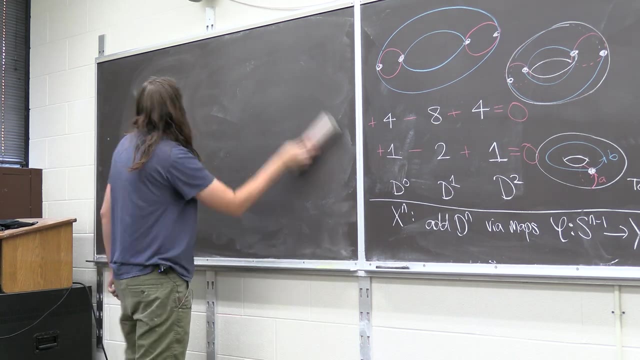 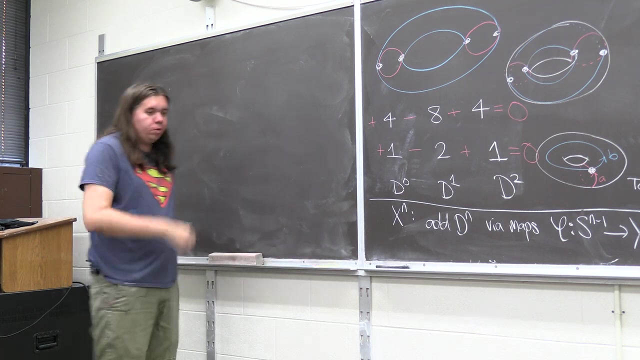 is. I want to talk about how to combine spaces, to get new spaces. Not just build up cell complexes, but operations to combine cell complexes- Cool. So let's talk about some operations on spaces, operations on these cell complexes. I'm going to do several operations. 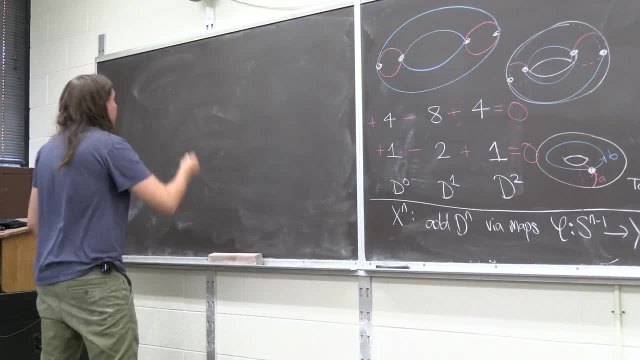 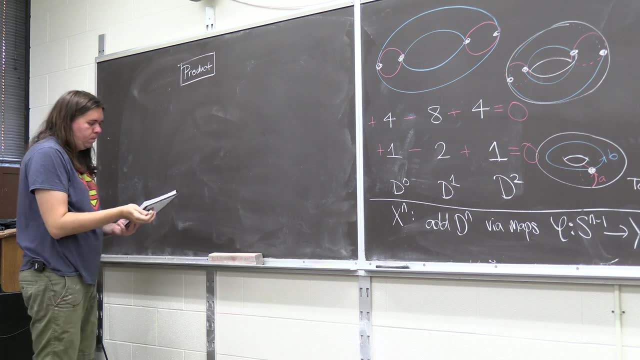 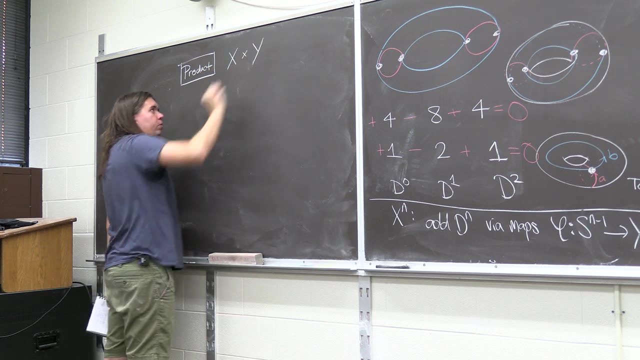 The first one I'll go through is just a product. If you have two spaces, x and y. I want to talk about what I mean by x cross y, And I think the best way to do this is just with a few examples. 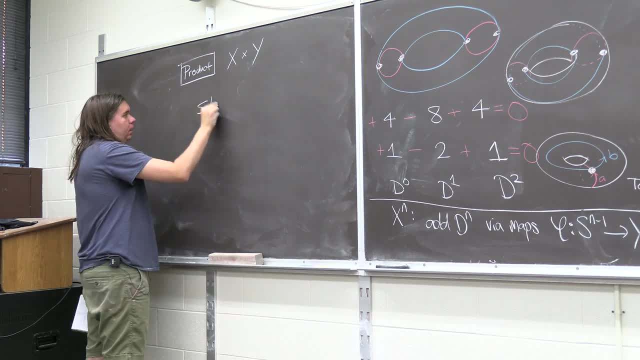 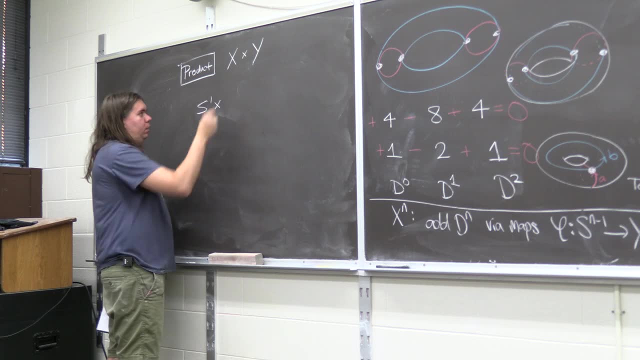 So let's say I have the space S1, and I want to cross it with a D1.. Okay, what I mean by D1,? D1 is just a line, So sometimes for D1, I'll just write it as 0, 1, the line. 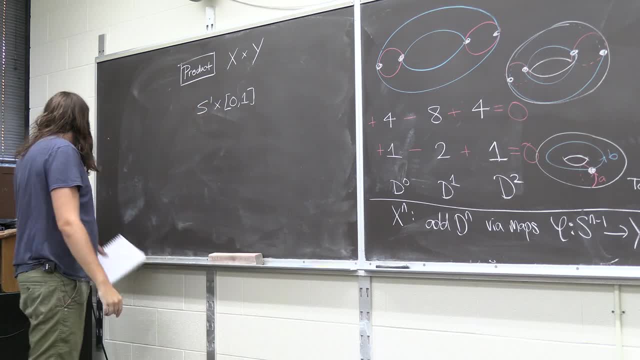 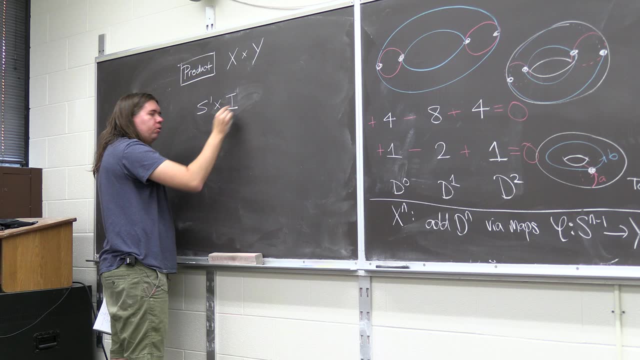 If you prefer negative 1 and 1, that's fine. We often use 0, 1 for convenience. Sometimes I'll write i meaning interval, right, Okay, So so you can instead think of this as S1 cross the interval i. 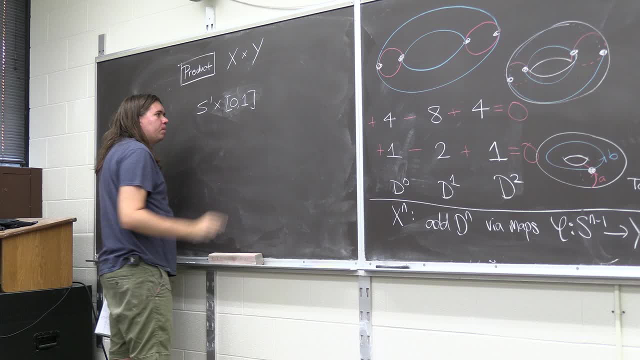 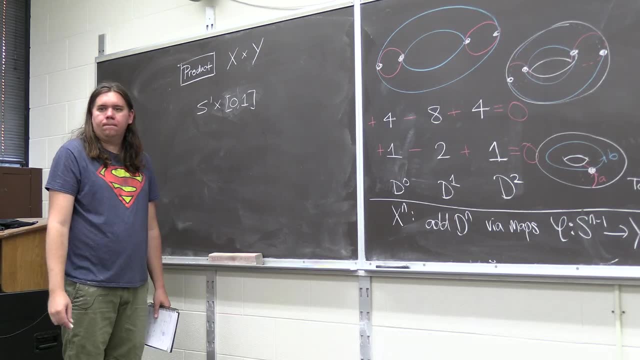 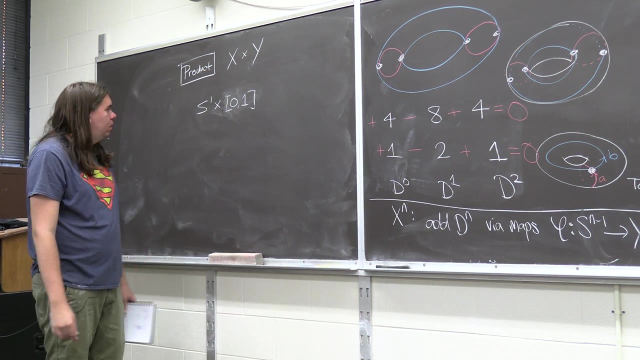 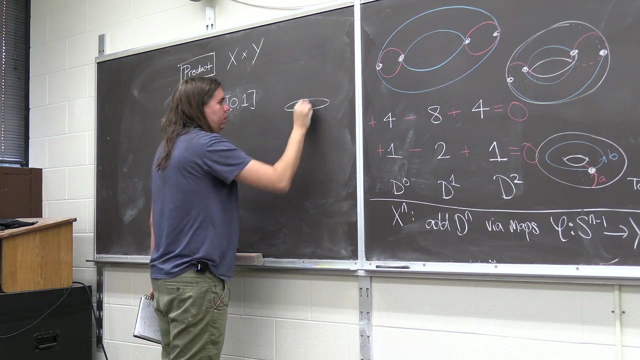 But to be explicit, I'm just going to write 0, 1.. What do you think this means? It's like a good interpretation of this. Well, you can think each point at S1 is going to become an interval. That is, you have S1, each point becomes an interval. 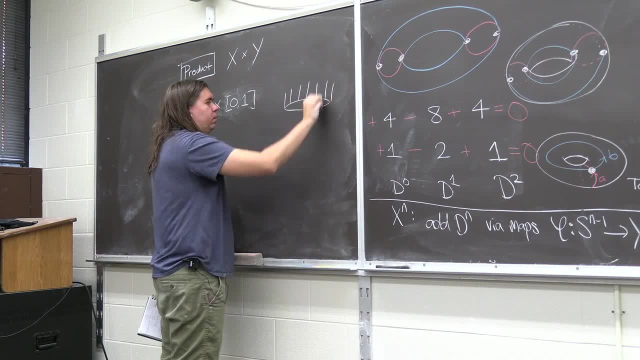 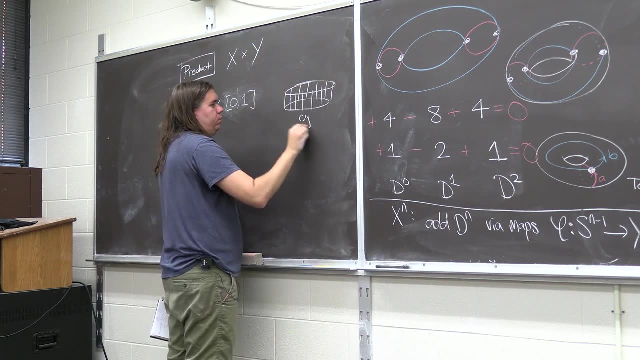 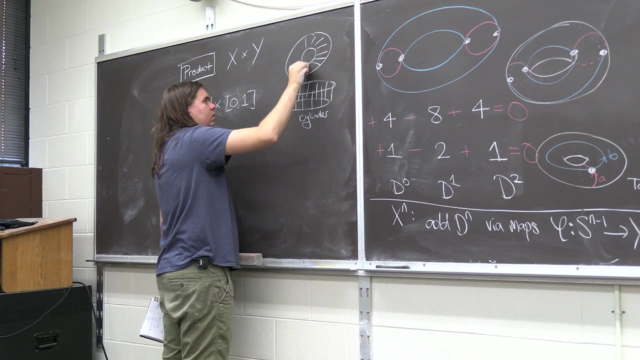 Each point is becoming an interval. Each of these points has become an interval. What is this? that I get? Just a cylinder. So this just gives you the cylinder, Or, if I had instead drawn it like this, an annulus right. 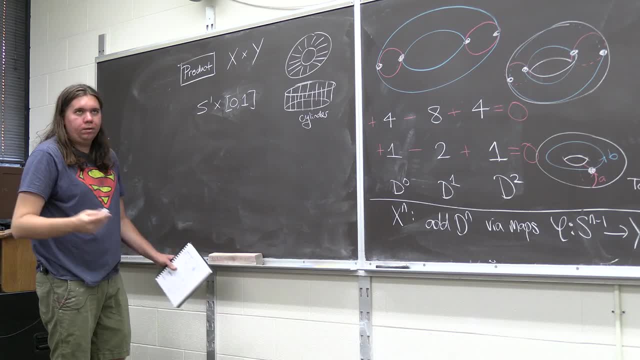 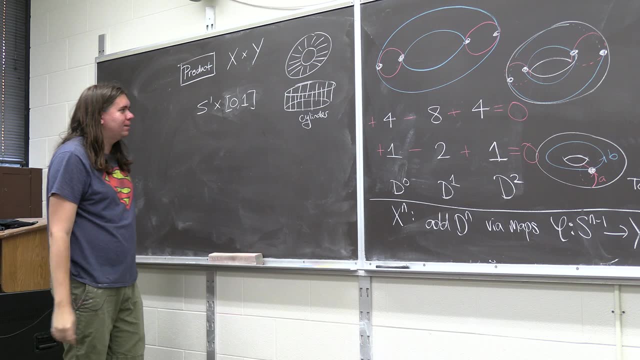 So cylinder or an annulus? Again, there's no metric here. So you know, don't worry that this length is a little bit less than this. You know there's no metric in this class. A little bit too, you know, a little bit too loose. 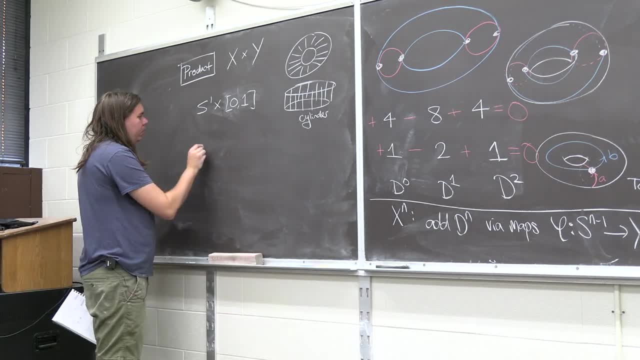 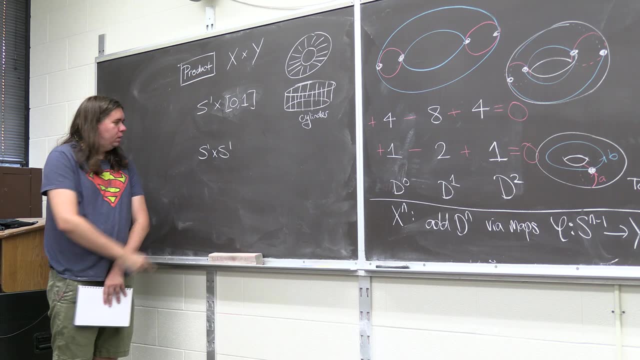 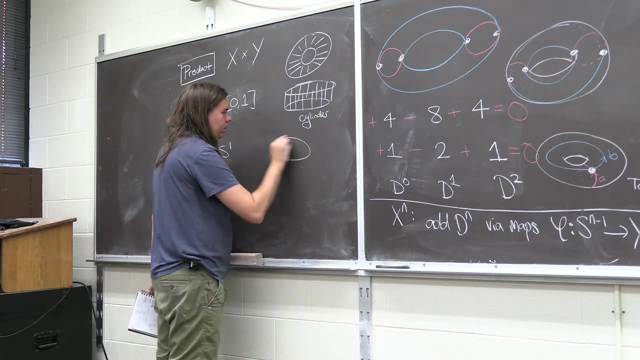 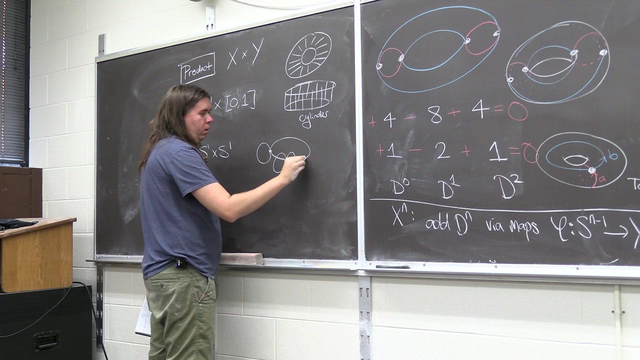 I'm just minded for metrics here. Okay, here's another one: S1 cross, S1.. A circle full of circles. What is that? Yeah, you can think. you take a circle and at each point it becomes a circle. Each point is. I mean, I can't draw for all the points. 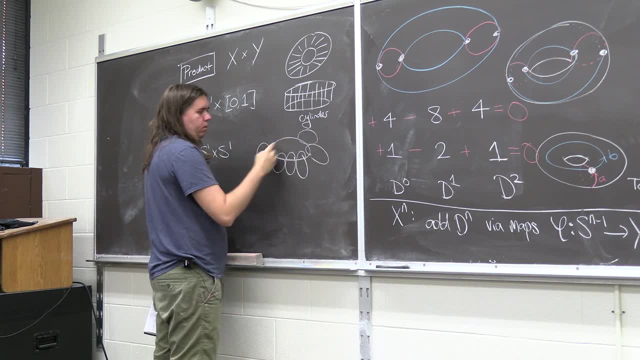 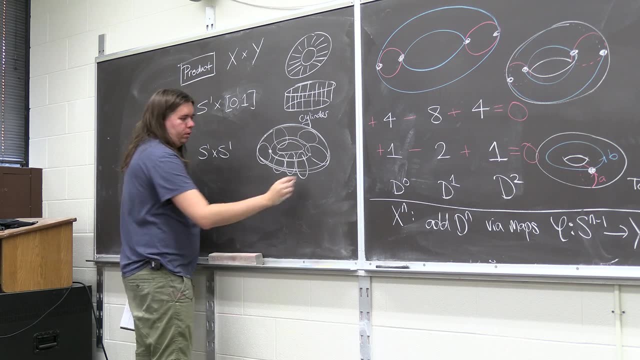 There's infinitely many. I'm trying to draw enough to give you a good, you know, idea what's going on. What is this going to become? This is just a torus. It's just a circle full of circles. It's just a torus. 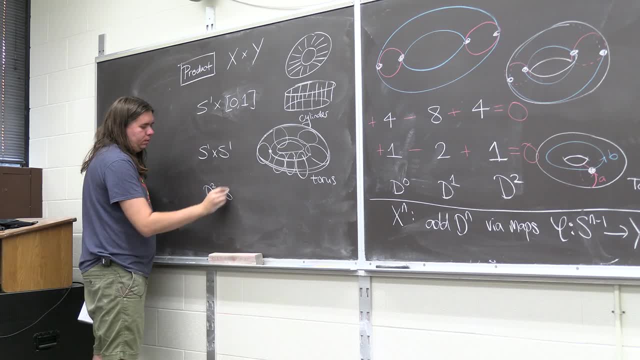 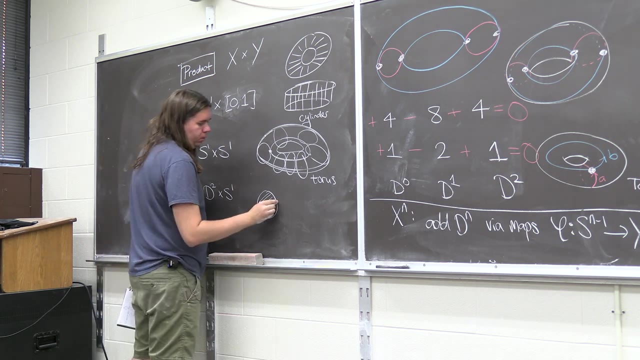 Okay, How about D2 cross S1?? What is D2?? Yeah, it's S1, filled in D2 cross S1.. Each of these points becomes a circle. Each of these points becomes a circle. Each of these points become a circle. 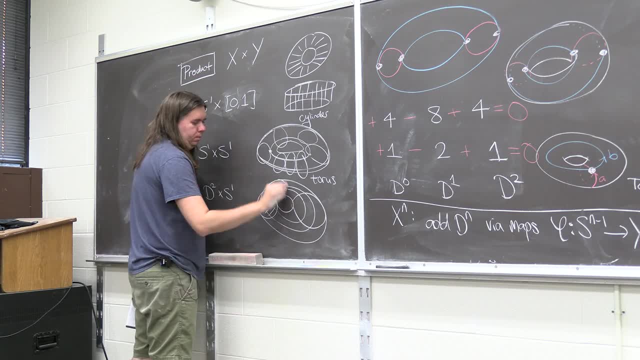 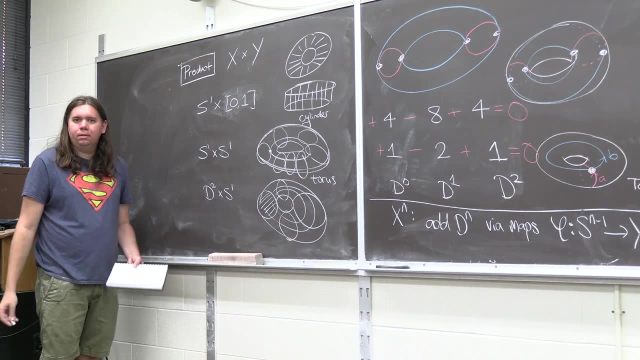 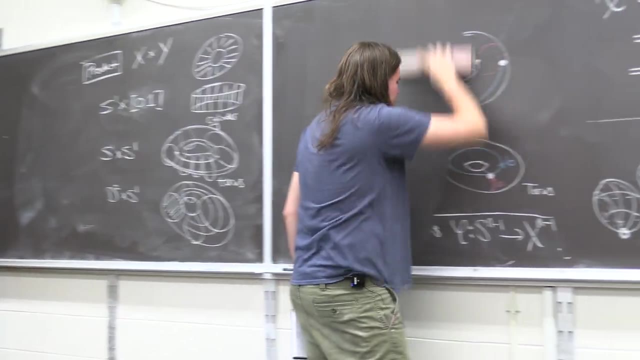 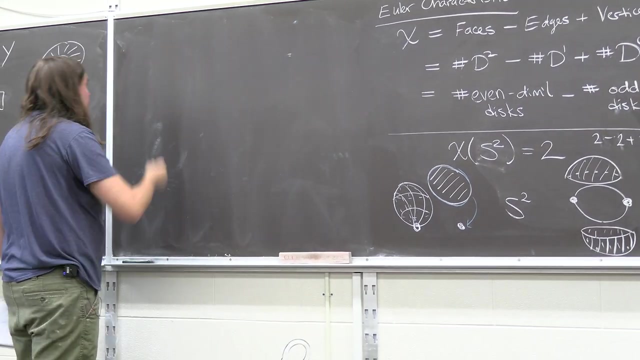 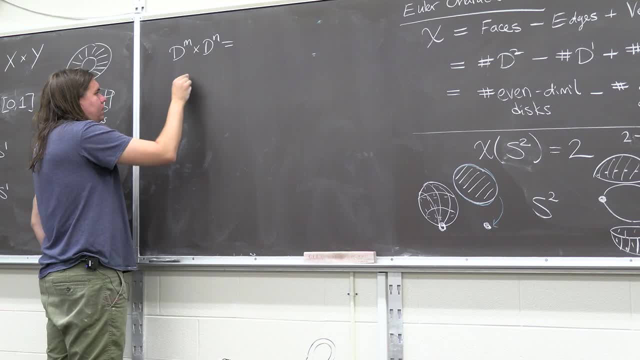 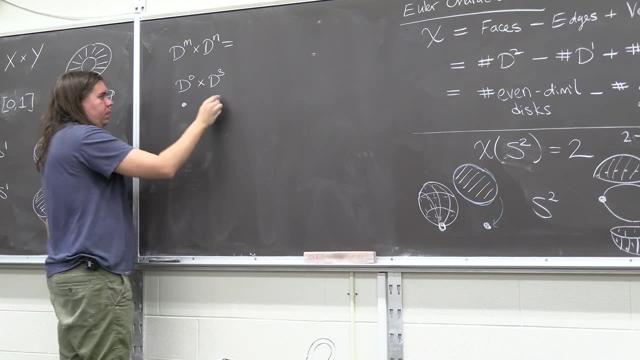 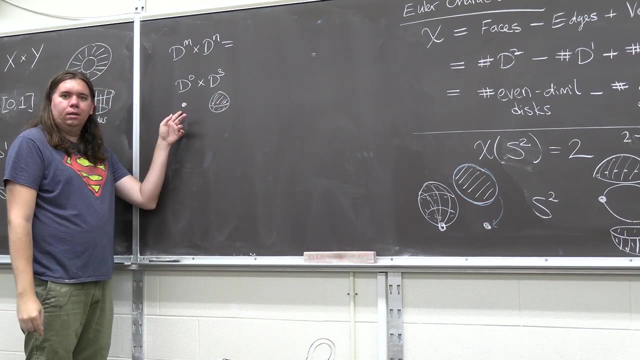 Okay, let's think of some examples. What is D0 cross D3?? Well, D0 is a point and D3 is the solid ball. What happens when you cross something by a point? Well, each point stays a point right. 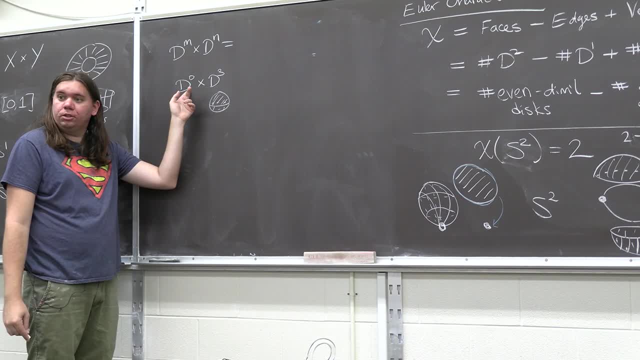 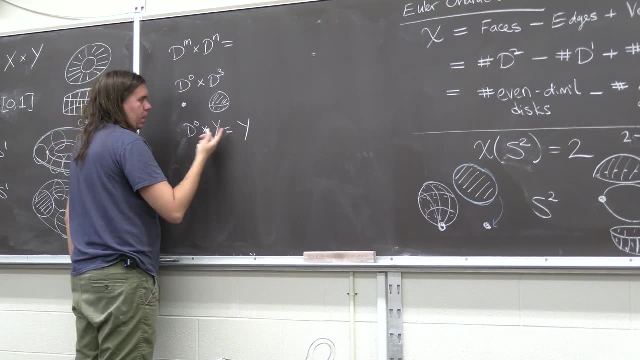 So crossing by D0 doesn't do anything. D0 is like the identity operation. So in general D0 is a point. So in general we could say: D0, cross any space, just leaves of that space. You're just crossing by a point. 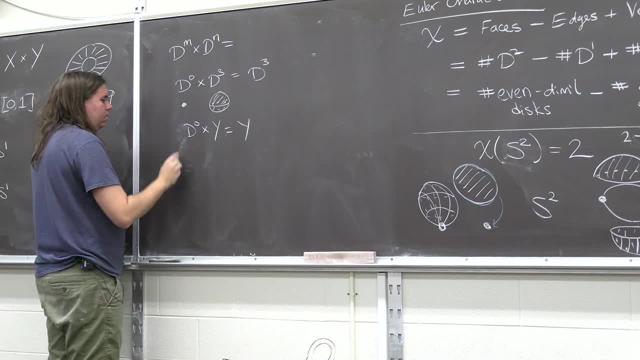 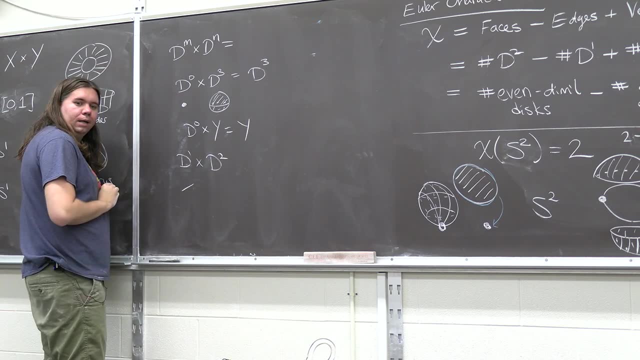 So that's just D3.. Okay, what if I want to do something like D1 cross D2?? D1 is interval line segment, D2 is the disk. What do I get when I cross those together? D3.. 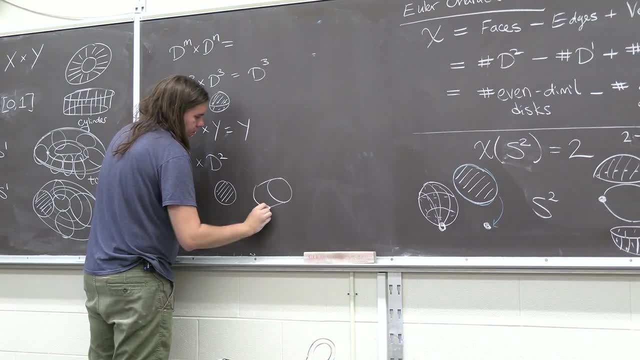 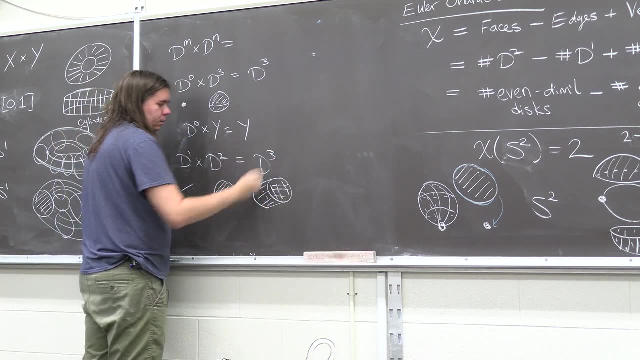 They're like: oh, some kind of like Thickened wedge thing, right, But it's filled in, it's solid. What is that? That's just a D3. Okay, typically you draw D3s like this, But it's a D3 that got smashed a little bit right. 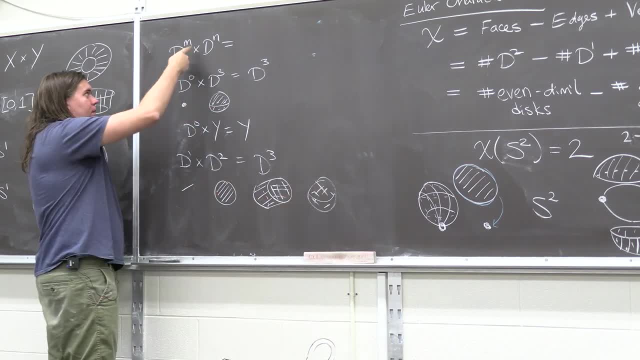 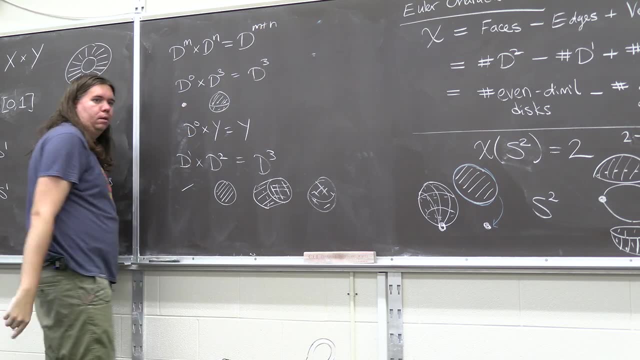 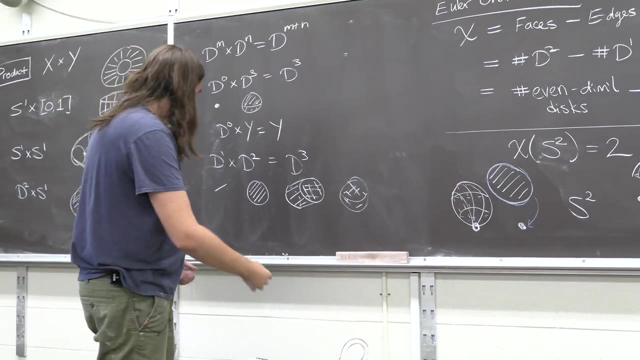 That's D3.. Anyone want to make a conjecture about Dm cross? Dn is Dm plus n. That's right. I'm just adding the dimensions. How about? here's one more interesting one. What if we include a couple of crosses? 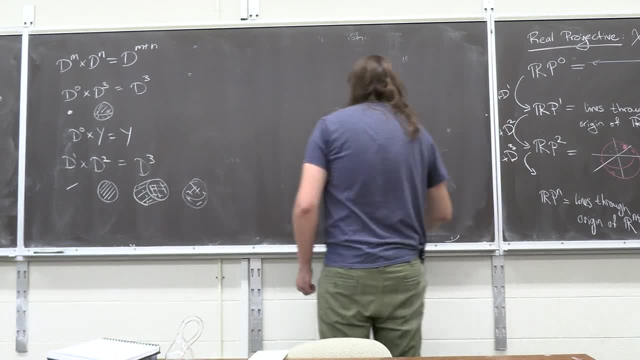 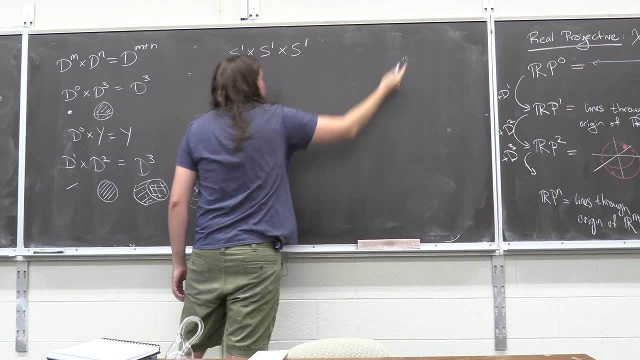 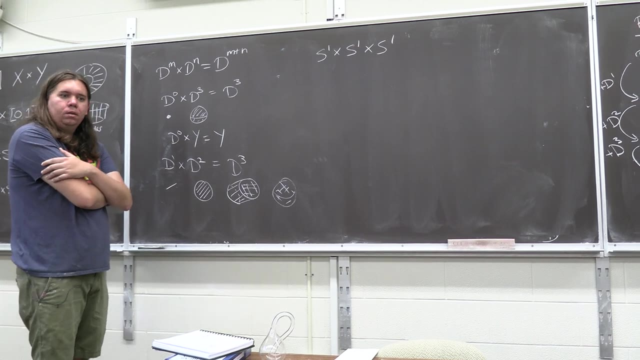 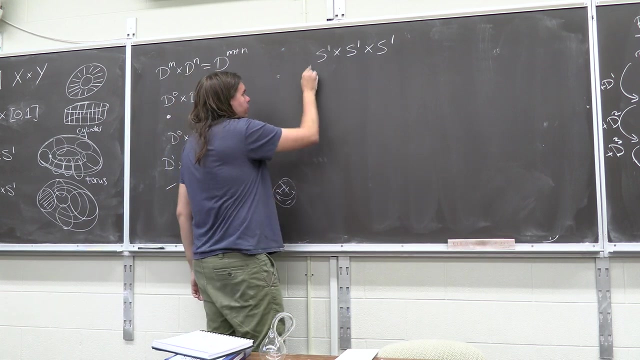 What if we do a product of, say, this one's a little bit tricky- S1 cross S1 cross S1. The product of S1 with S1 with S1. This might be a little bit hard to think about. Well, we know these first two give us a torus. 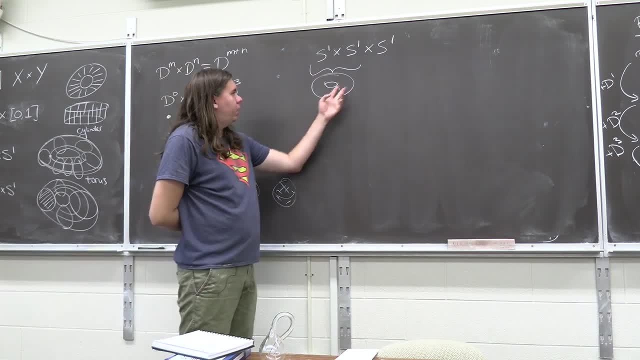 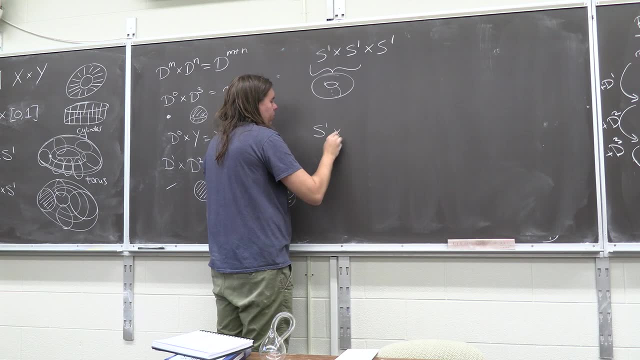 Not a solid torus, just the surface. And now we want to cross that torus with S1.. Now this might be hard to think about, So it may help if you first think about what is S1 cross. S1 cross with just an interval, say 0, 1.. 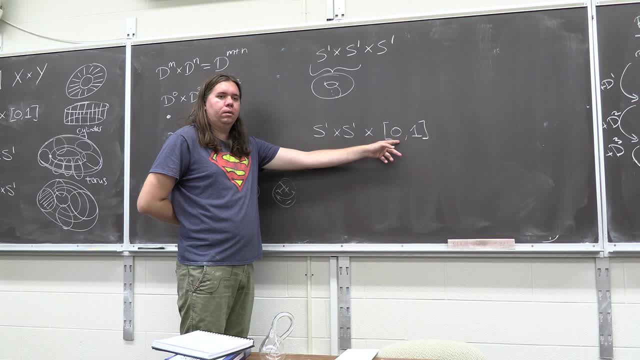 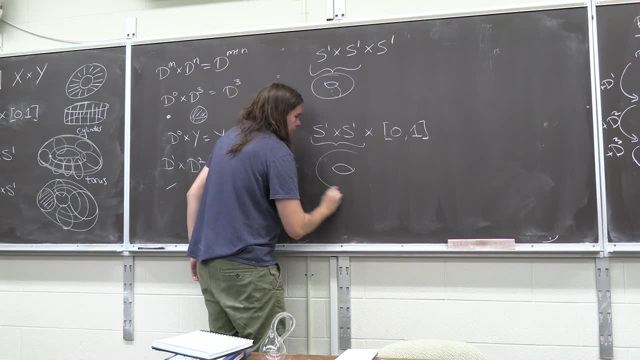 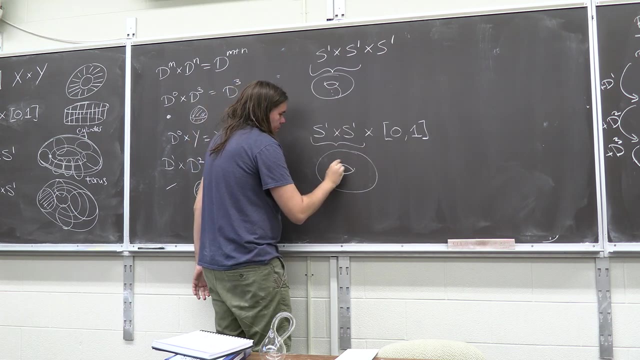 Right, What would that cross 0, 1 do? What was that word? Yeah, it would thicken it up. You have your shell and this cross 0, 1 thickens the whole thing, Right? So you might think it ends up being like a torus with like a drilled out center. 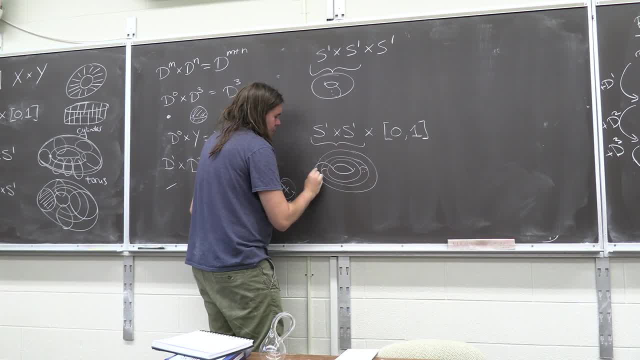 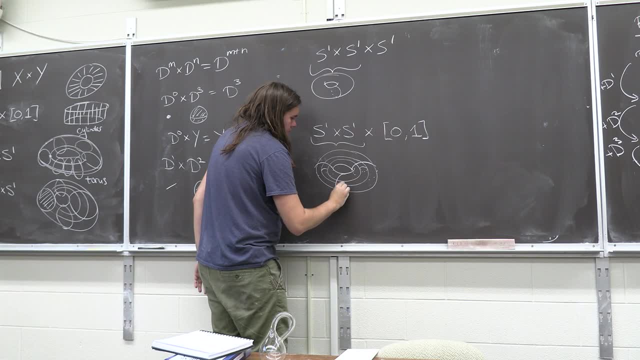 Right, It's like it has this drilled out center. You have the overall torus, But this center is like a torus. This center has been drilled out inside of it. Hopefully we can see what's going on here, Okay. 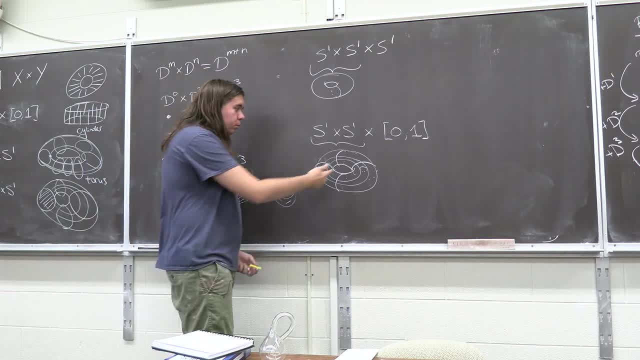 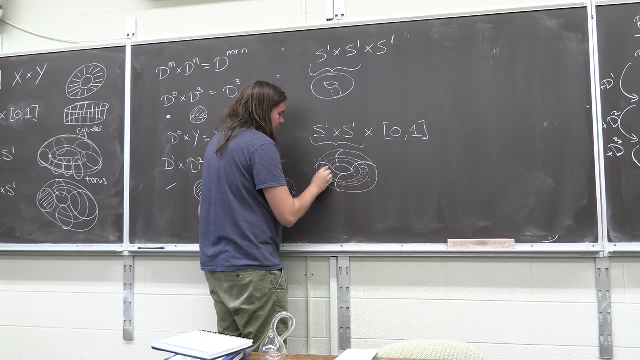 So it's like someone came in. It's like a jelly donut where someone ate all the jelly Right. It's a jelly-less donut. All this jelly has been eaten out. It's hollow inside. There's no jelly in there. 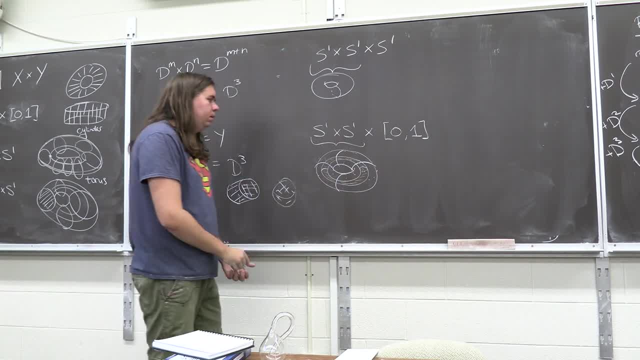 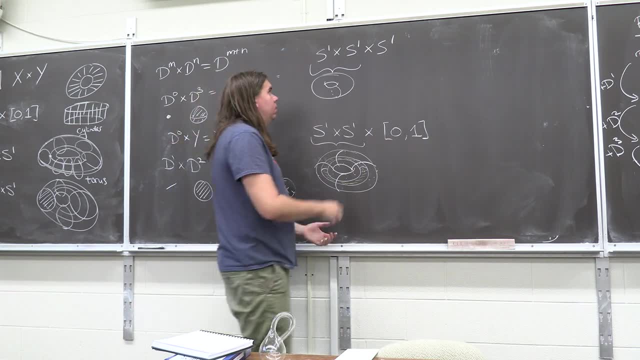 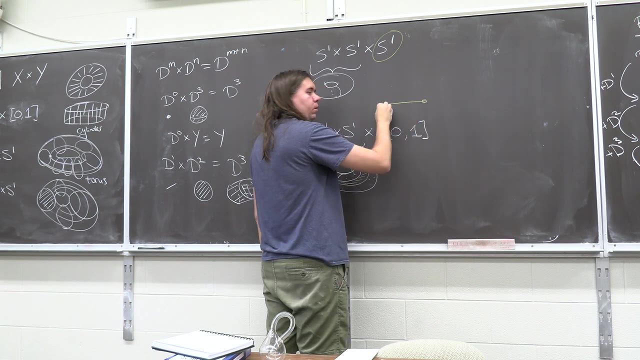 No, jelly, What a sad world we live in. Right, Okay, But now that you have that picture in your mind, what is S1? S1.. This S1 is exactly 0, 1, identifying together the 0 and the 1.. 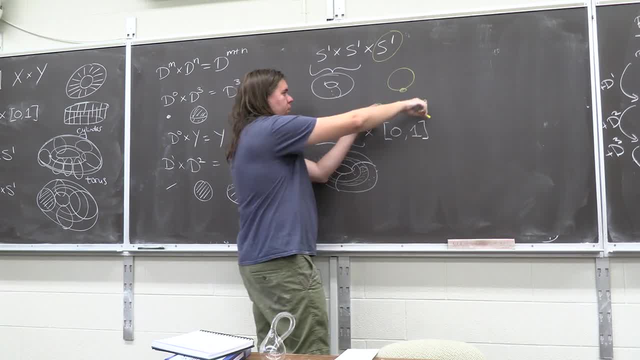 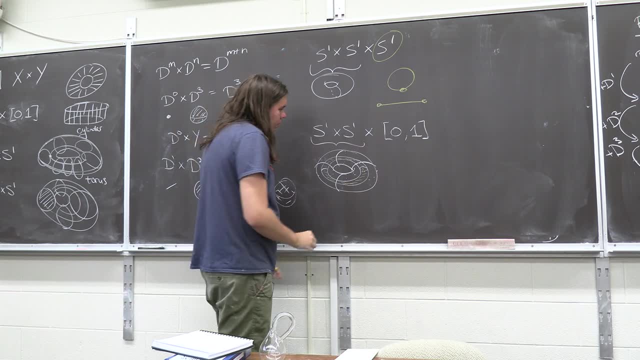 Gluing together the 0 and 1.. Right, If you just glue together the 0 and the 1, you get S1.. So the way you think about this is: you're in this jelly-less donut, but as you travel through and you get to this edge right here, 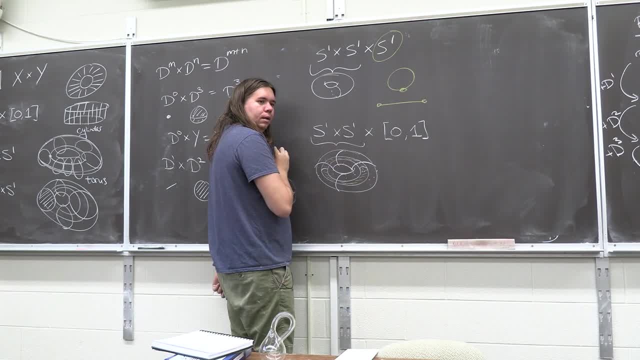 it's identified with that point. on the inside, Each of these lines is like this line, where one end gets identified with the other. You're like in this jelly-less donut, but when you get to this point you're back at this point. 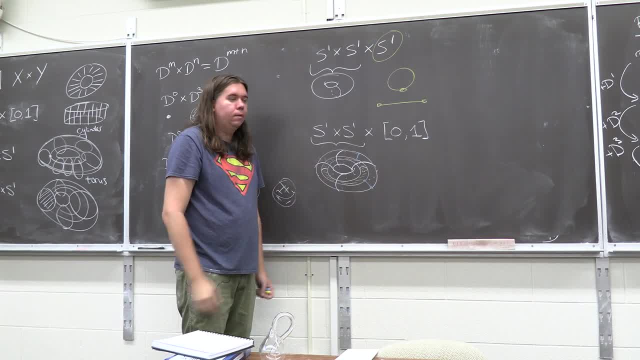 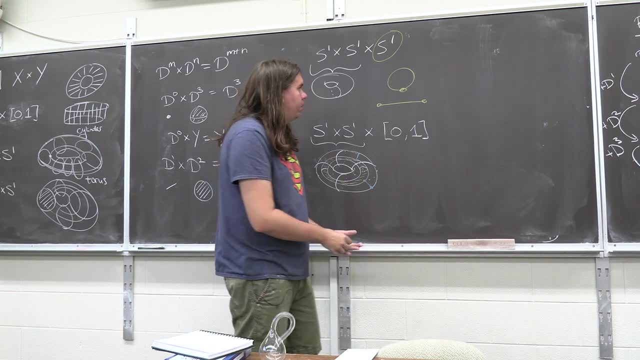 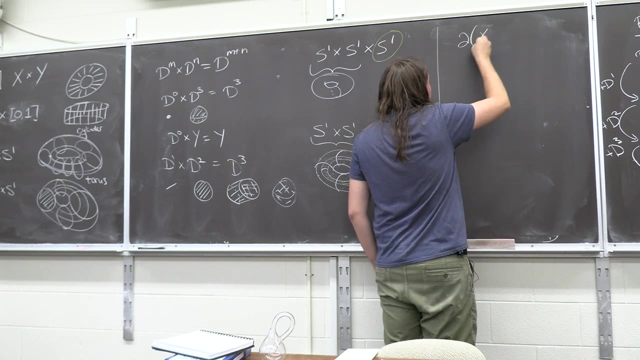 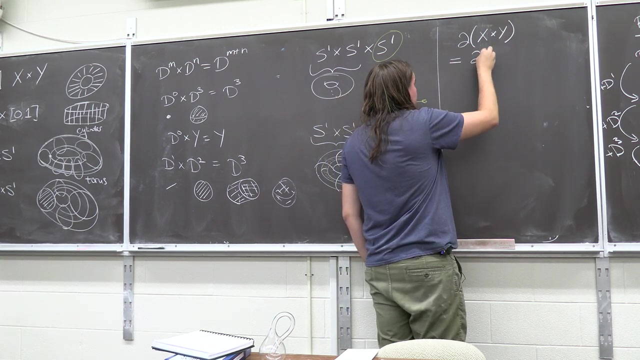 So there's no boundary to this shape, Whereas here there is boundary. I should take a second and talk about boundary. If I want to calculate the boundary, I should take the origin of a product. This is my notation for boundary. The way we do it is, it comes out to be simply the boundary of x, cross, y. 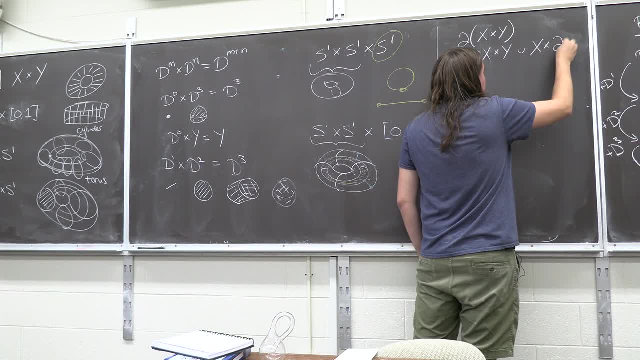 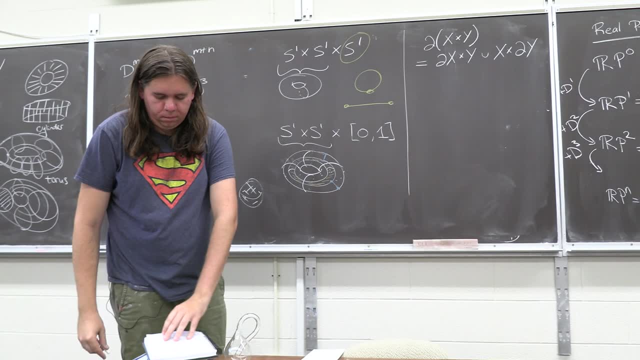 union x cross the boundary of y. So let me give some examples of that. You're going to be able to see this: Let'sлись wich Theяни c, The g S2.. So this is a hanno. we give some examples of that. 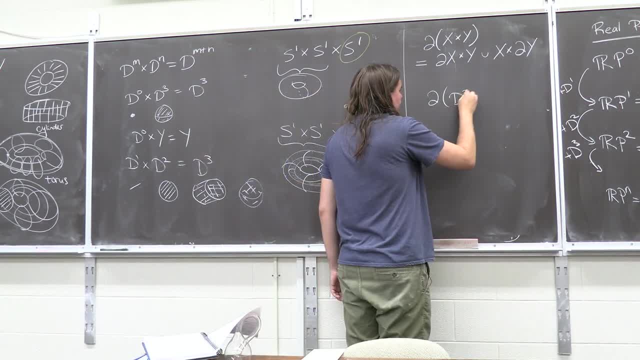 Let me do one more answer on this. You are going to take a second and this is already. this is in this rectangle. It's not actually done it. We've needed down the conversations of the wearing. What's the boundary of d2, cross the interval. 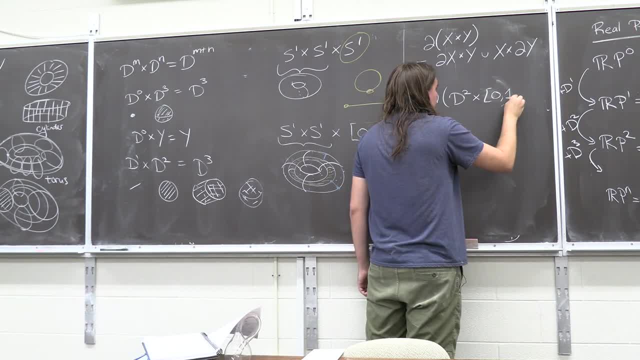 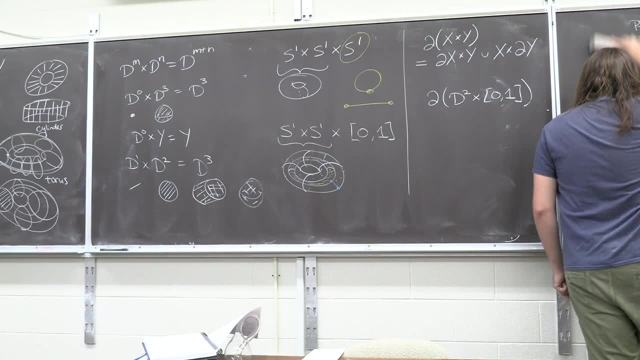 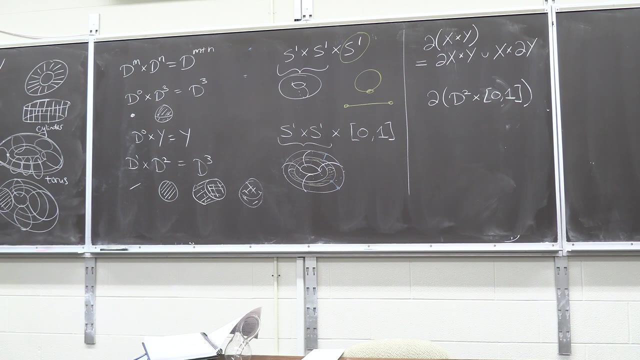 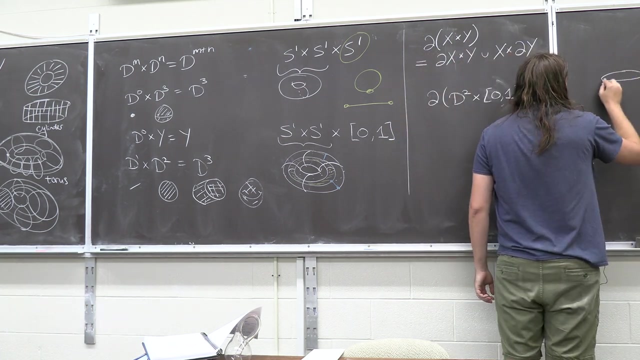 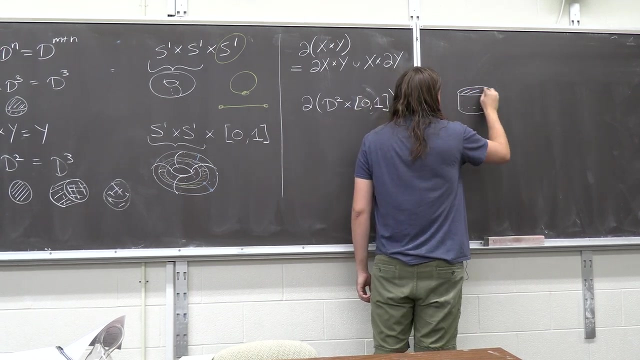 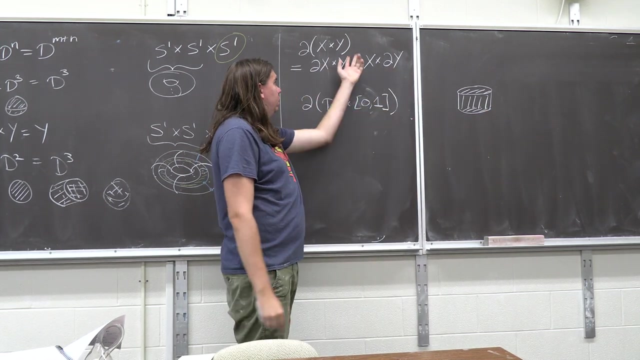 So this is d2 cross 0, 1.. So we can visualize d2 cross 0, 1.. d2 cross 0, 1 is just the solid cylinder, right? So what's the boundary of that? Well, let's use the formula. 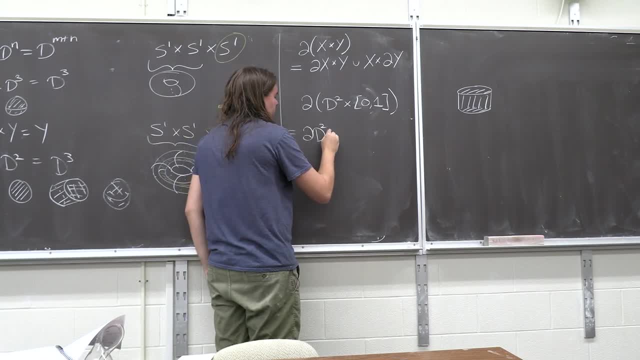 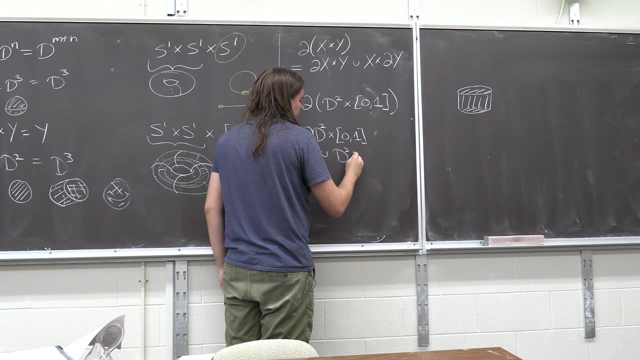 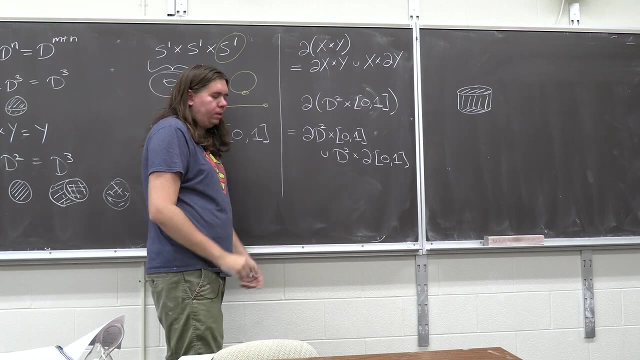 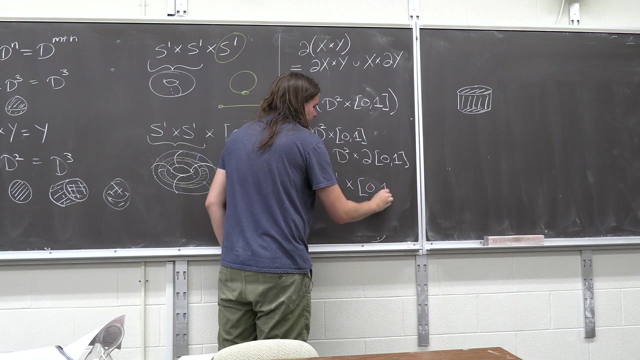 It's the boundary of d2 cross 0, 1. union. d2 cross the boundary of 0, 1.. Talk about this first piece. What is the boundary of d2?? S1.. S1 cross. S1 cross 0, 1.. 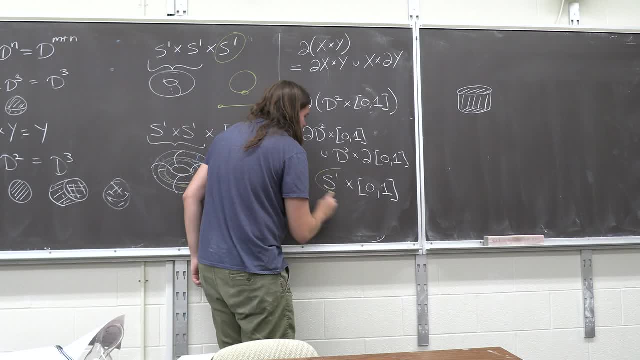 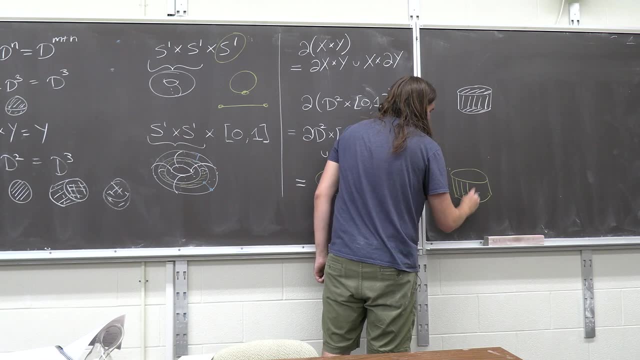 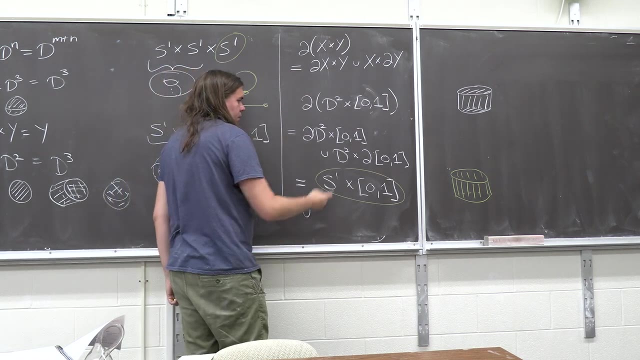 That's this first piece right here: S1 cross 0, 1.. That's just going to look like S1 cross 0, 1.. That's just a cylinder Union. What's the boundary of the interval? 0, 1?? 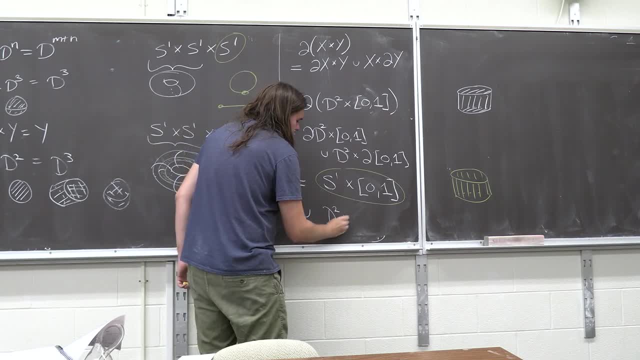 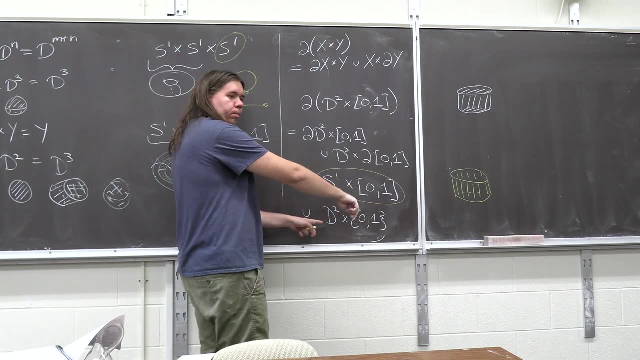 Two points. right, It's d2 cross two points: The point 0.. And the point 1.. Which just means two copies of d2.. Each point of d2 becomes two points, becomes two copies. So this guy down here is saying two copies of d2.. 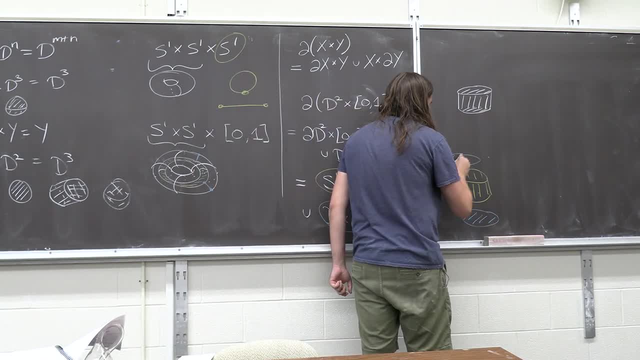 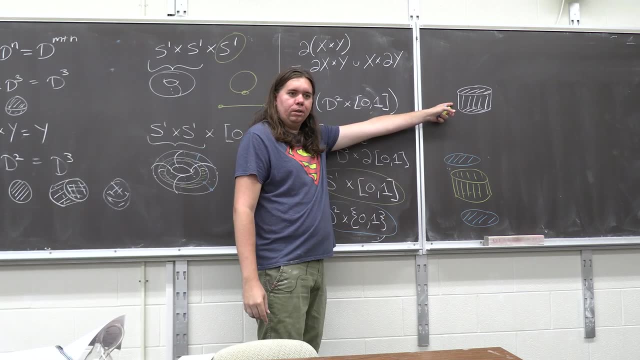 A copy of d2.. And a copy of d2.. And when you glue those together, what does it give you? Well, just the boundary of the cylinder, right? Okay, I also need to keep track of how they're glued together. 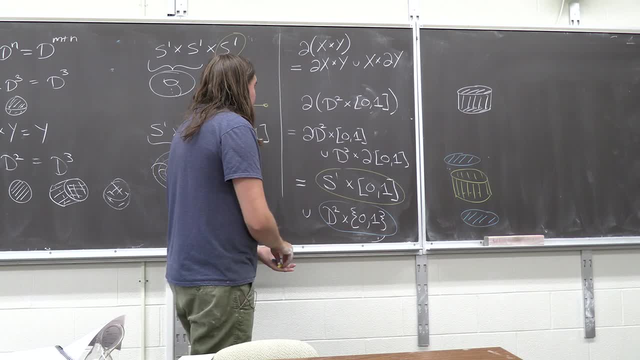 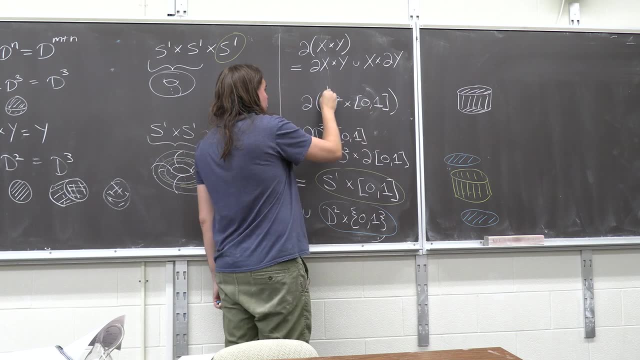 I won't worry about that too much. But here's another way to think about this. This is just d1.. What is d2 cross d1?? This is just d3.. I'm just asking you, what is the boundary of d3?? 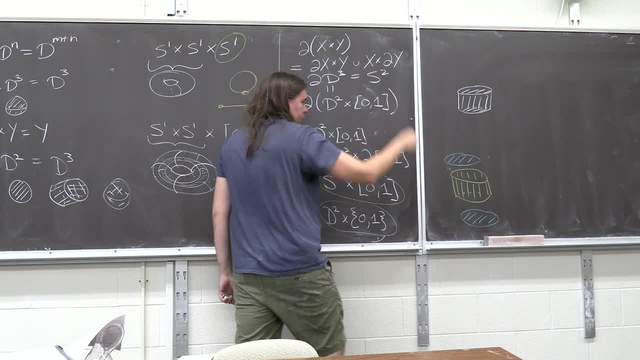 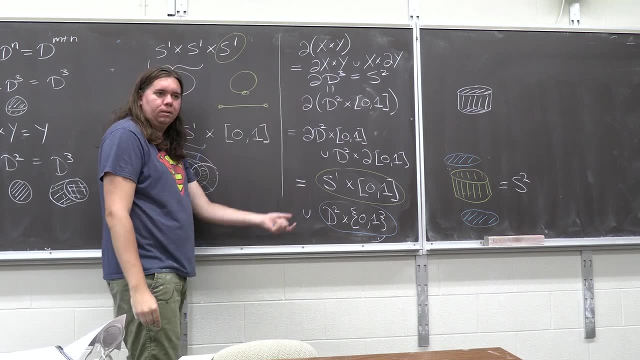 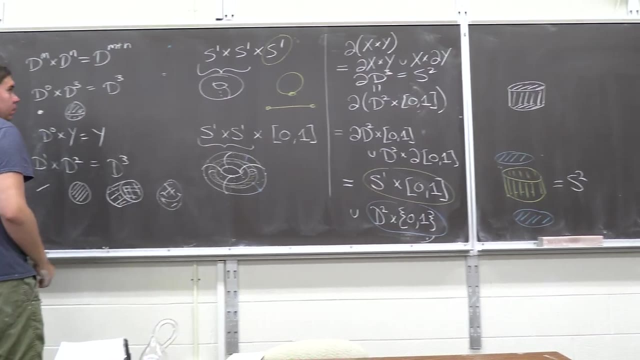 What is the boundary of d3?? It's just S2.. And, sure enough, when you glue this together, it's just S2.. Right, So it all agrees. Coming back to this example, Well, what is the boundary of S1?? 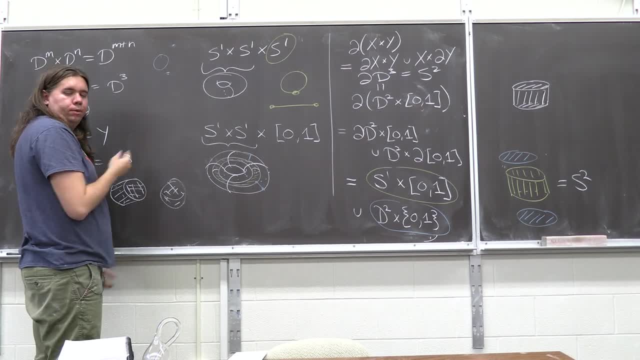 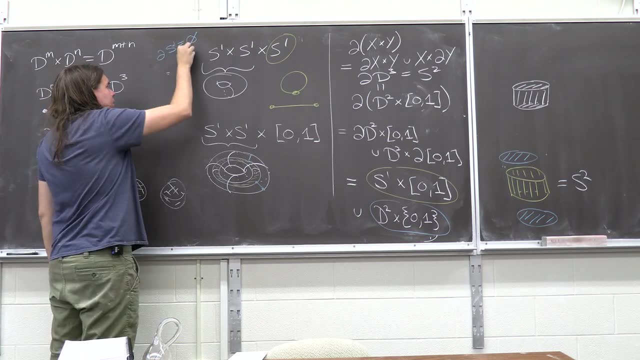 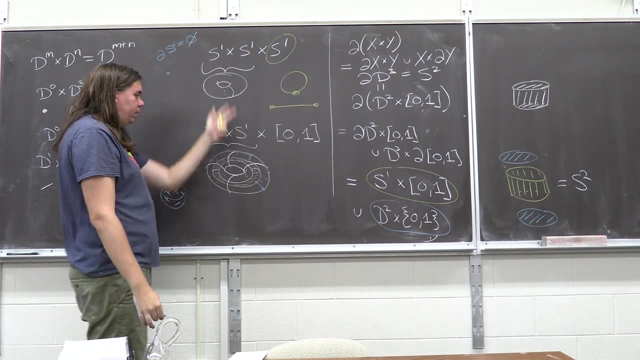 What's the boundary of a circle? There is no boundary. It's empty. The boundary of S1 is empty. So when I take the boundary of this whole thing and start taking the boundary of each piece, it all becomes empty. So this has no boundary. 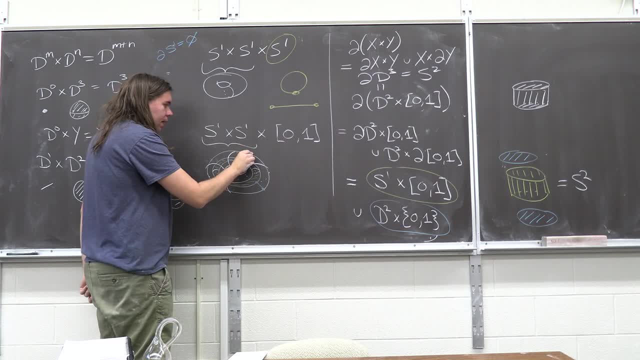 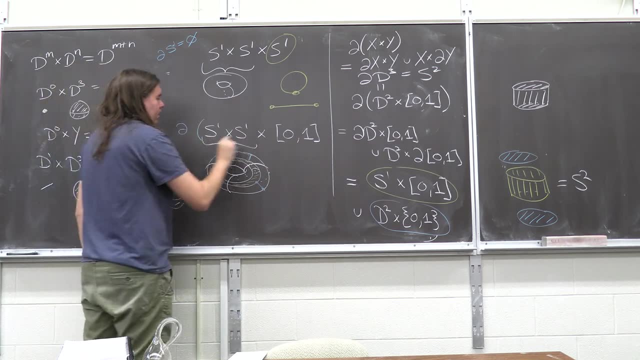 This has no boundary, Because when you're inside, you're going to have a circle. You never get to the boundary. You travel to the end, you're back inside, Whereas this guy does have a boundary. The boundary of this guy is: 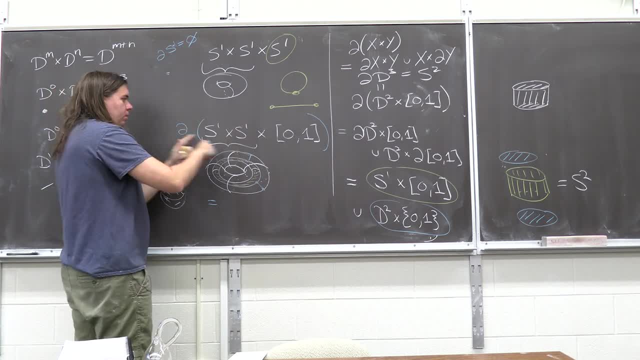 well, when you do the boundary of S1, it becomes empty, so that piece is nothing. When you do the boundary of S1, it becomes empty, so that piece is nothing. But when you do the boundary of the interval, you get two points. 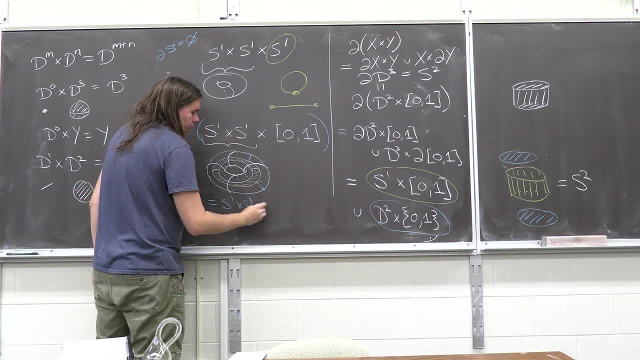 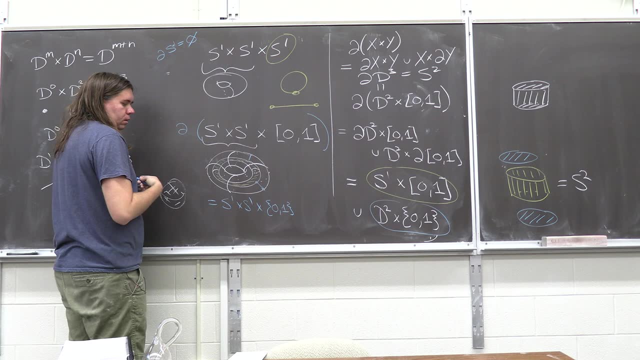 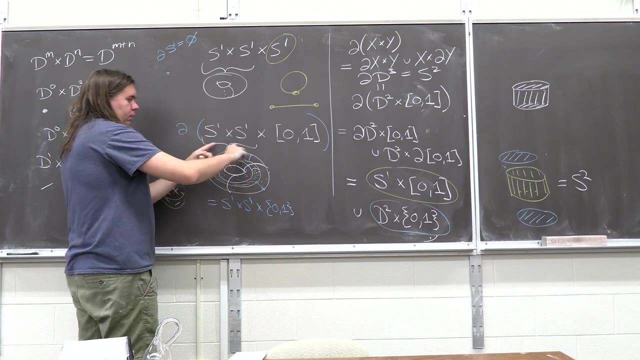 So it's S1 cross. S1 cross the points 0, 1.. What is this saying? What is the boundary of this guy? It's just two copies of the torus, The inside torus and the outside torus. So here you have an inside torus and an outside torus. 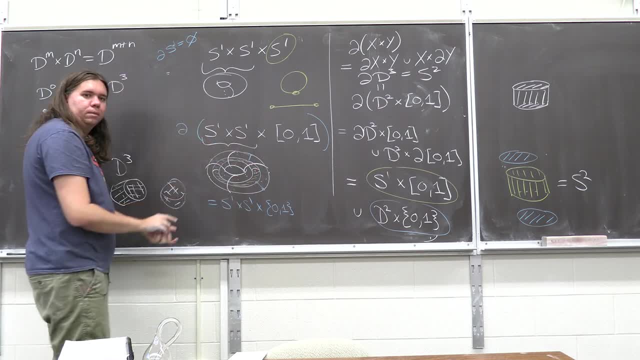 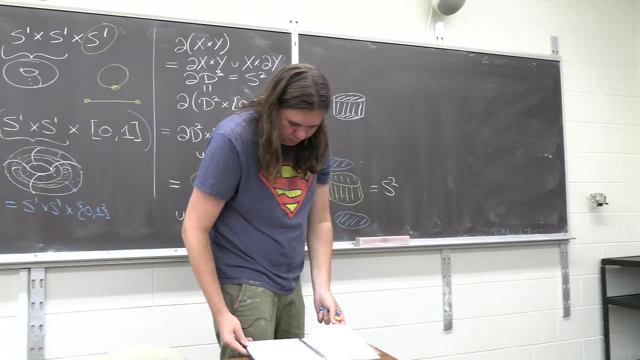 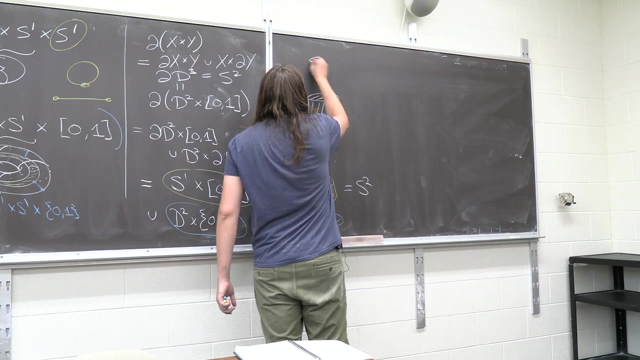 But when it becomes S1, those get glued together And now there is no boundary. Okay, let me show you one more thing you can see with boundary. This is pretty neat. What is the? what is S3?? How can we think about S3?? So this might seem kind of weird. like what do I mean? 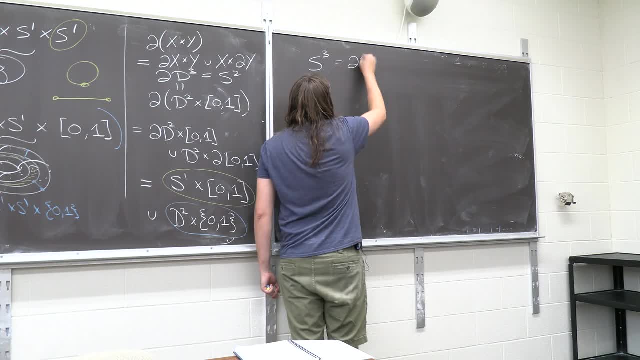 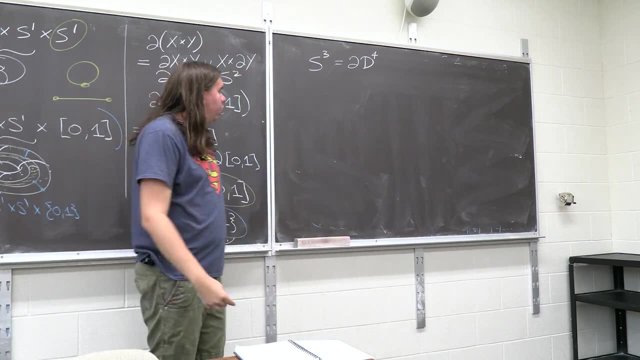 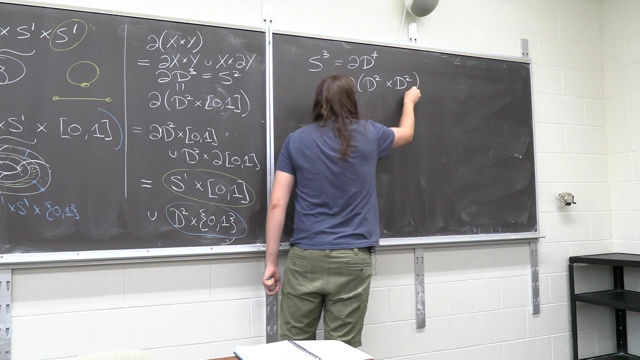 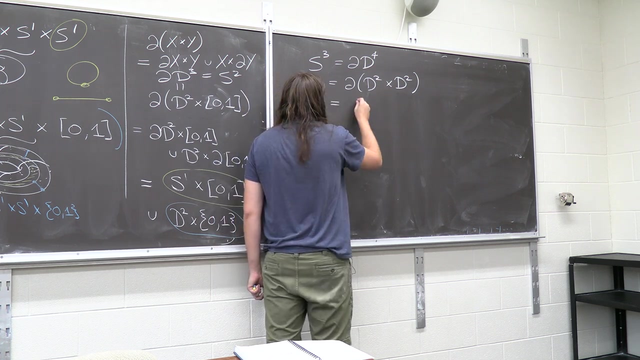 by S3?? Well, it's the boundary of the four-dimensional ball. We're not used to thinking about four-dimensional balls, but you can. The four-dimensional ball is just the product of a two-dimensional ball and a two-dimensional ball Which is just using our boundary formula, the boundary of D2, cross D2, union D2. 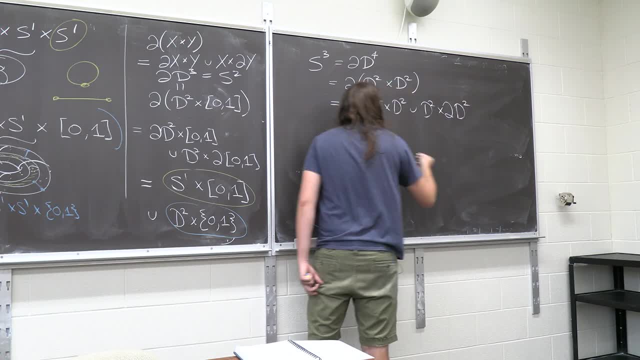 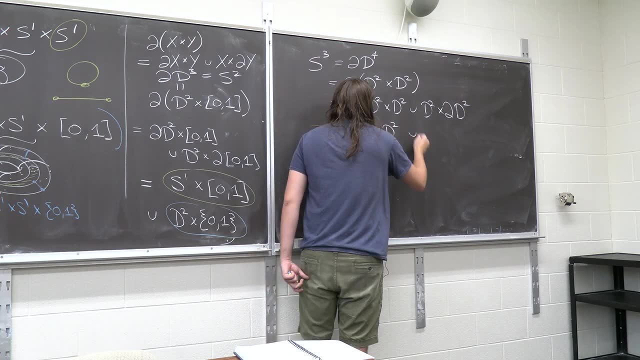 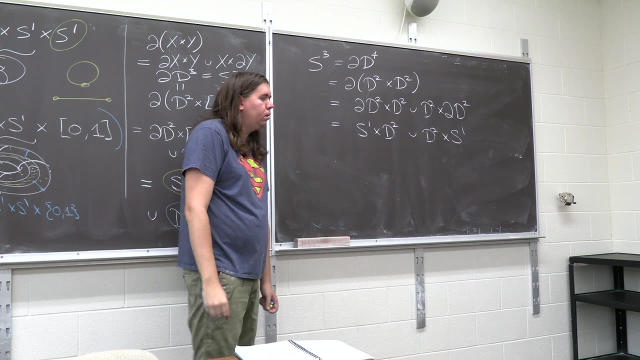 cross the boundary of D2.. The boundary of D2 is S1.. So this is S1 cross D2, union D2 cross S1.. What is S1 cross D2?? Yeah, S1 cross D2 is Okay, let's see. 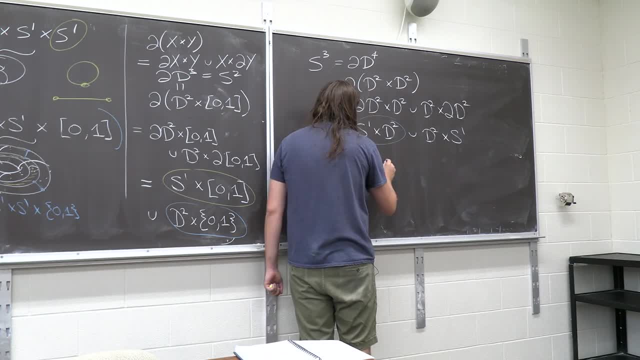 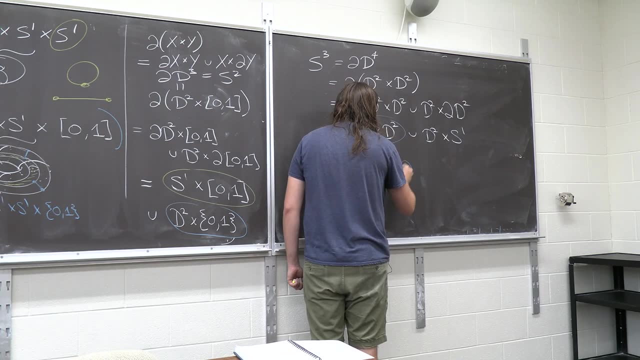 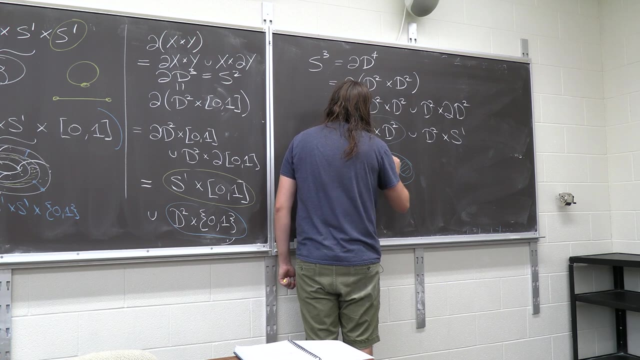 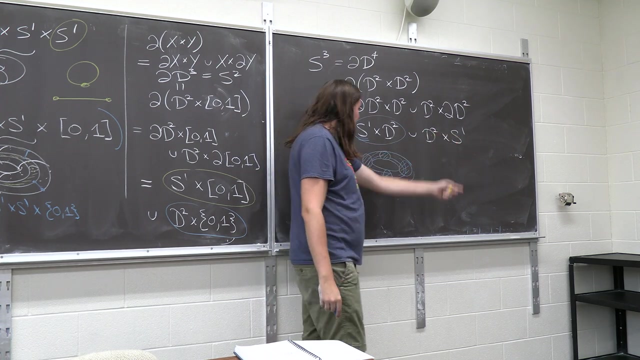 Let's see, try and draw this in a consistent way. i'll draw my s1 going around this direction, so that means my d2 is coming around here. it's the solid torus, solid torus. so here we have my solid, trying to draw here a solid torus, solid torus. this is also solid torus, but this being opposite. 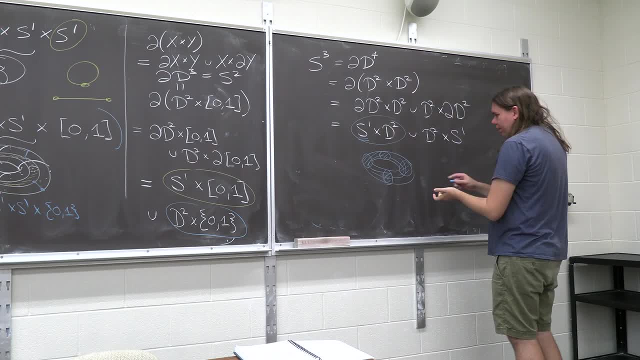 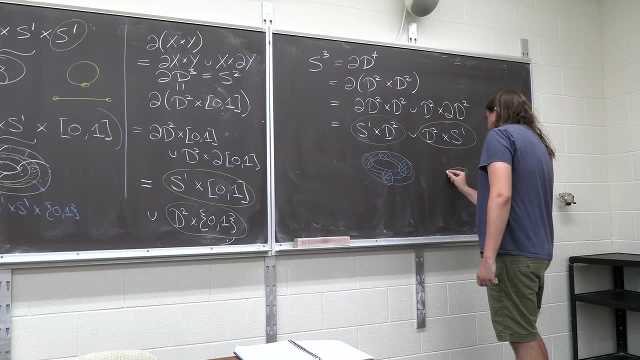 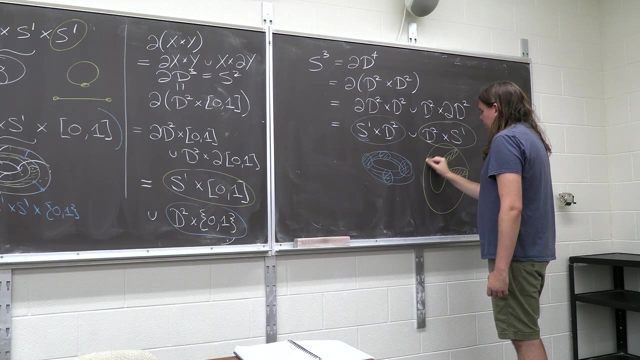 suggests the way you should think about this. s1 is moving the circle, moving the other direction, so you should think about this guy more like: here's my d2 and my s1 moves around like this, so it's also a solid torus, another solid torus. 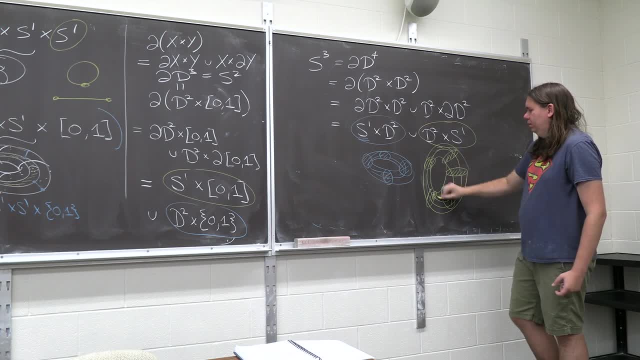 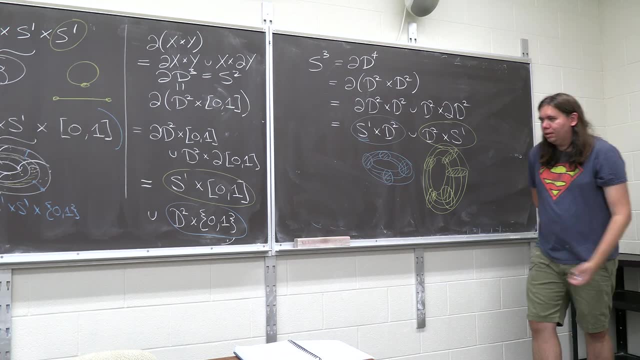 this is saying: if you glue together two solid tori, glue together two solid tori, you get s3. this is really counterintuitive, and so i encourage you to take a look at this and see if you can figure out how to draw a solid torus in this direction. 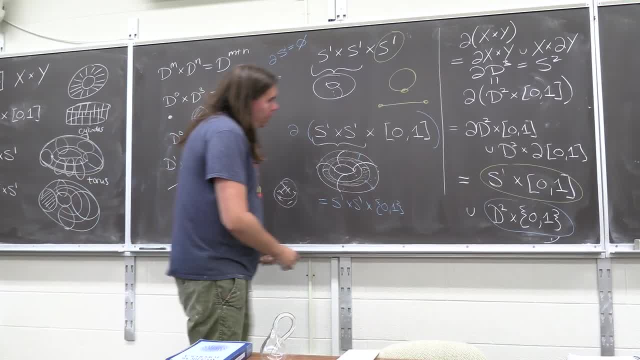 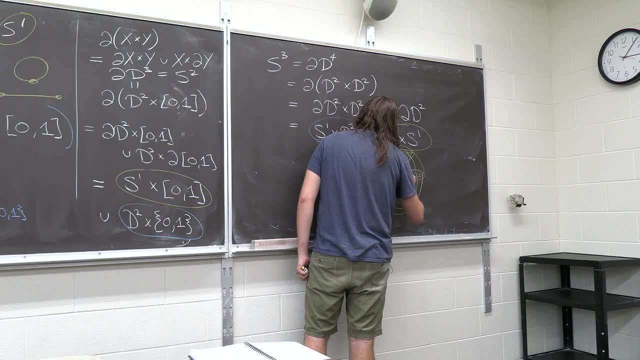 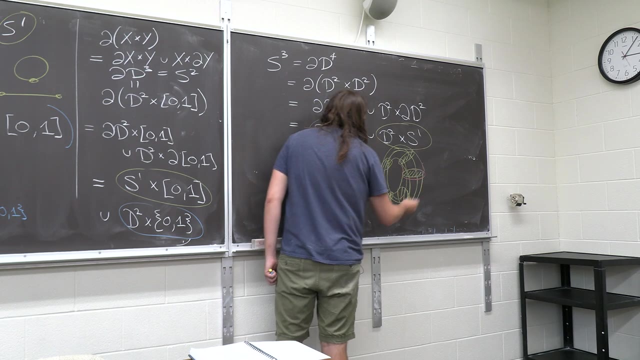 some time to think about this. but the way to begin thinking about it is is take the center of this, like this, this circle right there, and and glue this bit in, so like stick that in the middle right and then, as you start coming up here, that's like gluing along all this bit. 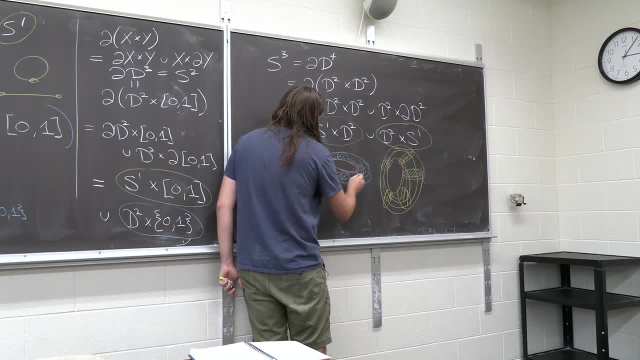 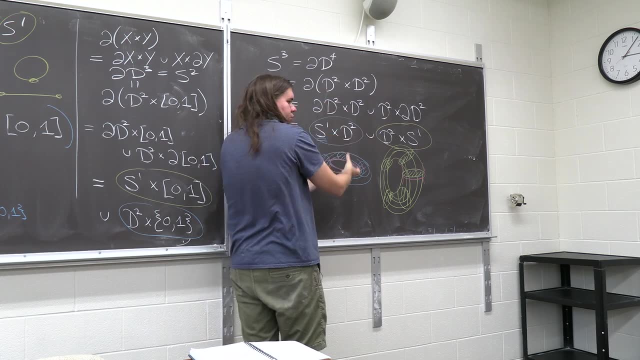 and as you're coming down, all this down here is getting glued to the bottom part. but what's going to happen is like it's not just if there's a cylinder, you can kind of glue it and kind of try and stretch it right, but what happens is like this: 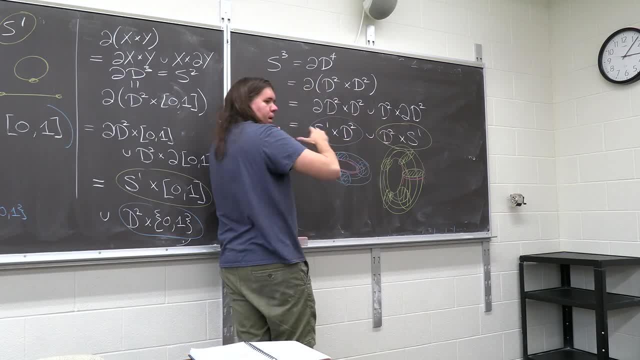 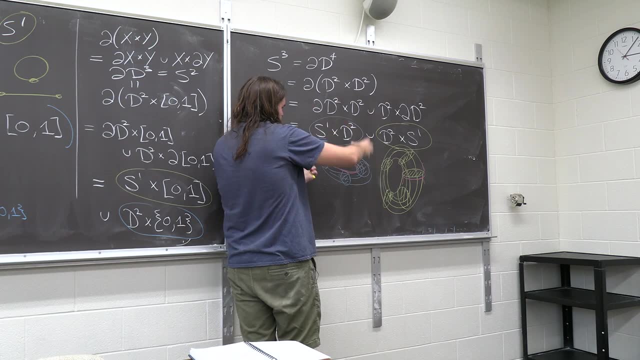 this bit here gets stretched and it fills in all the space outside because it's like it has to connect back upon itself. so maybe first you break it open, you try to glue it, but then you have to glue this on himself and it's filling all the space and it becomes what we call a. 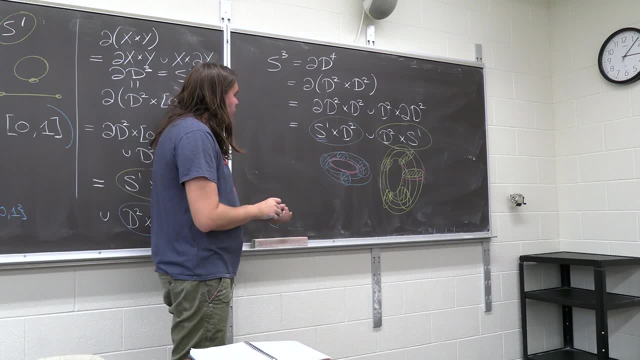 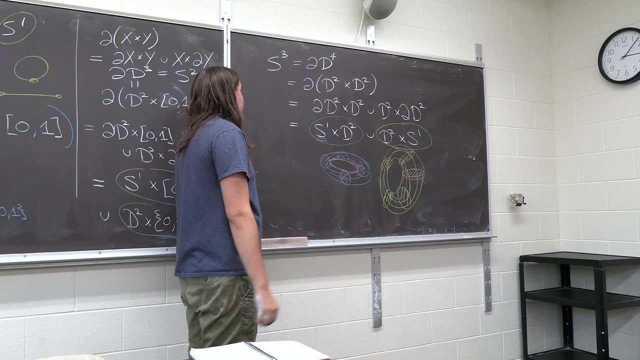 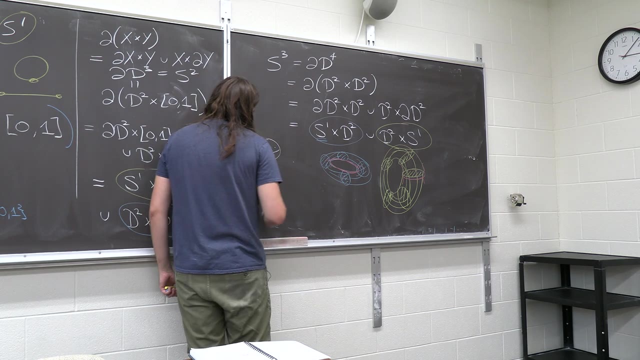 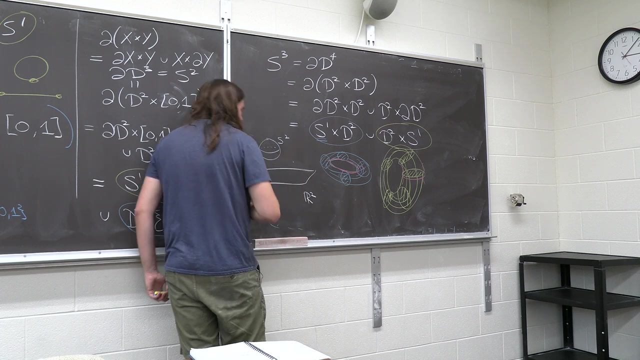 one-point compactification of r4. so essentially, what's going on here is just like how you can um think about a disc as being um, just like how you can think of, like a sphere s2 as corresponding to r2, through like this classic projection you've probably seen before. 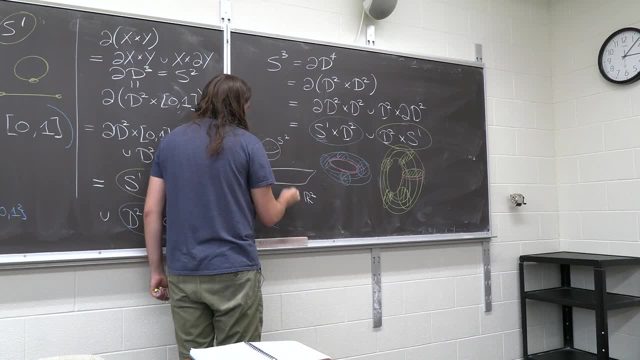 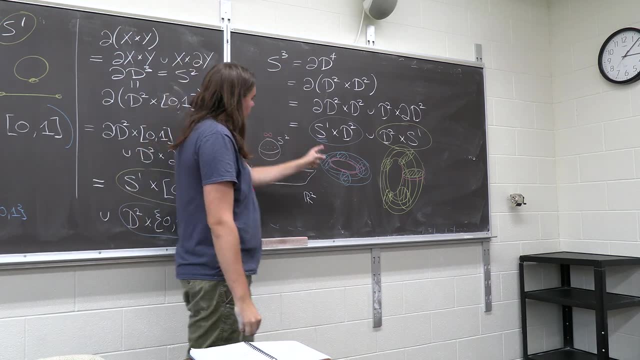 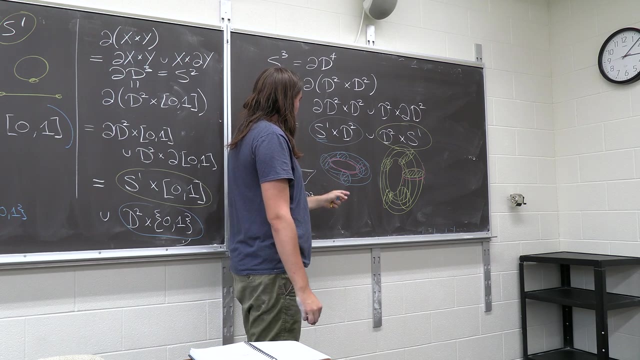 where points down here correspond to points on here, but then on the very top there's a point at infinity. the same thing is going on in s3 is you have each point being filled up in s3, but then there's a point over here that corresponds to a point at infinity. when you try and stretch this over, it hits all the. 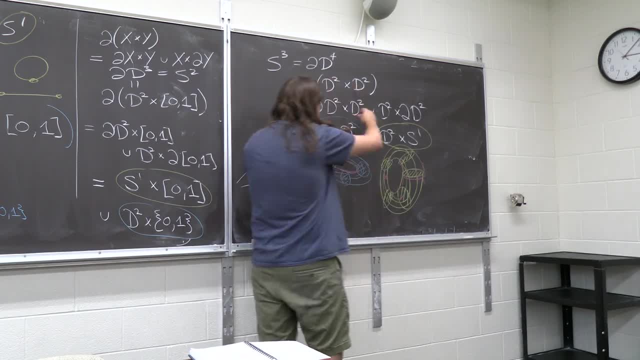 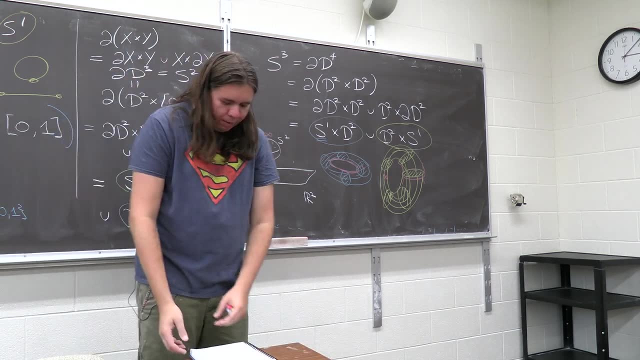 points off at infinity and so when you're trying to glue this bit on at the end you're going off to infinity. so this is kind of mind-boggling, but you can think about that. okay, i've only told you about products, and there's a whole lot more operations i want to tell you about. 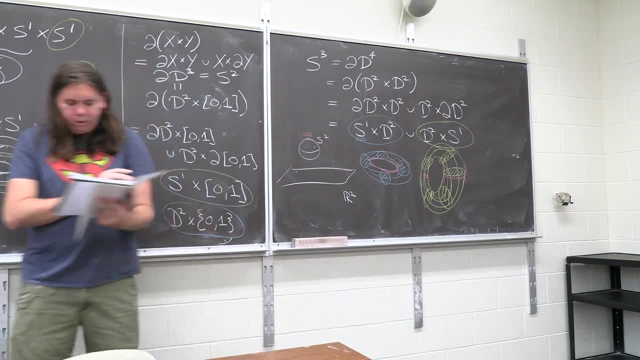 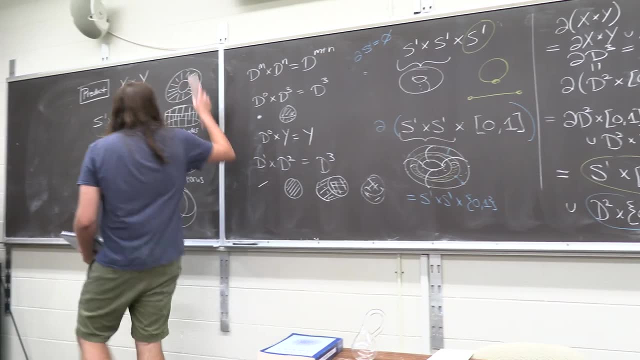 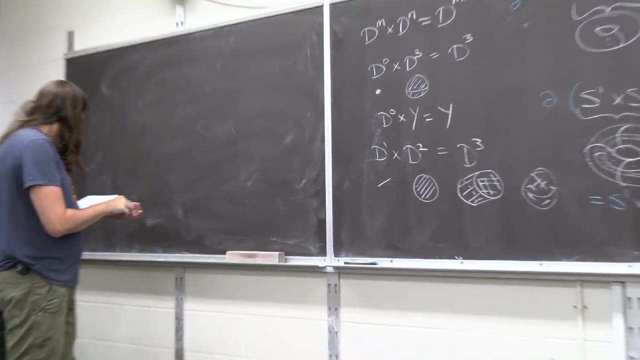 i don't know if we have much time, let me let me just mention one or two of them, and and then we'll pick up with more as we need them. maybe the only other one i'll tell you for now, just because it's so significant, is quotients. so we know how to do products. how do we do quotients? 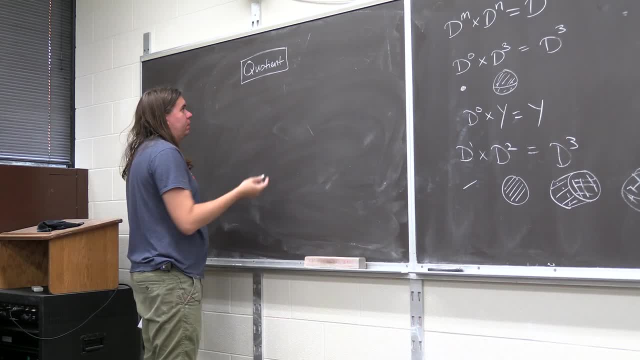 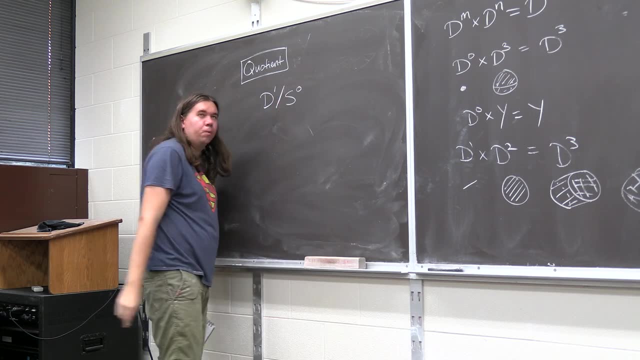 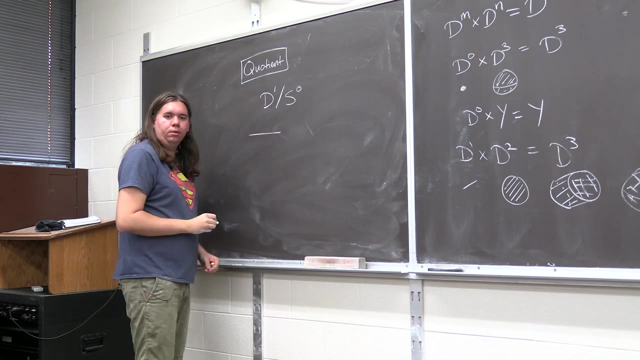 okay, so a quotient. what is what i mean by division? what do i mean by something like d1 divided by s0? well, d1 is just the line, and what is s0? two points. so here i'm thinking: what is the s0 that naturally lives inside of d1? 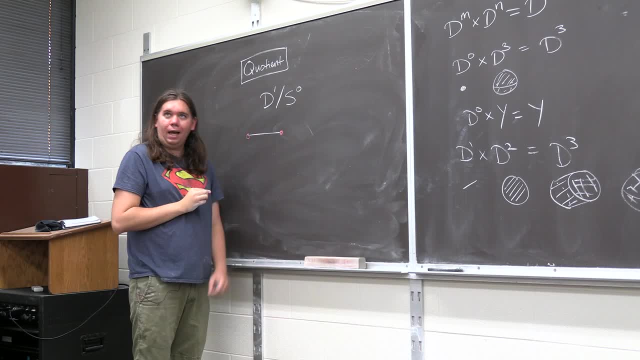 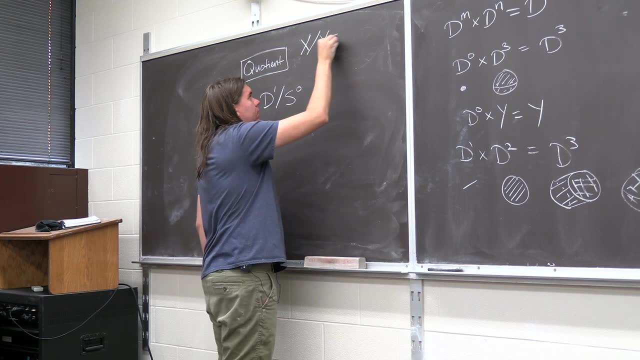 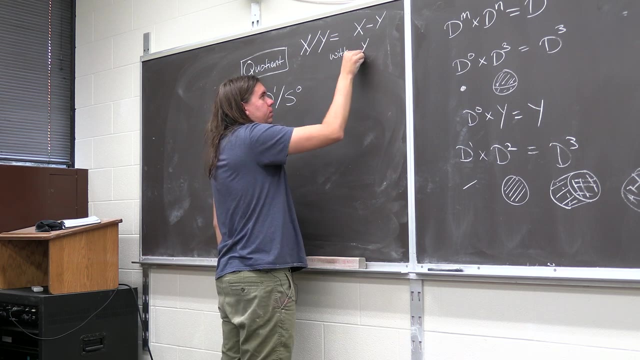 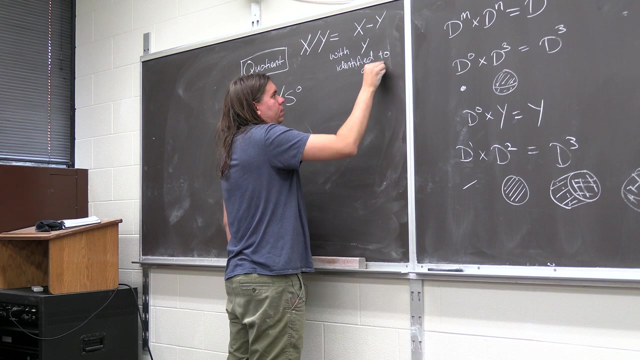 well, it's these opposite points, and so when you quotient out, what you're left with, in general, x quotiented by y is going to be the space x minus y, with the space y identified to a point, identified to a point. so these two points i'm going to identify to a single point. 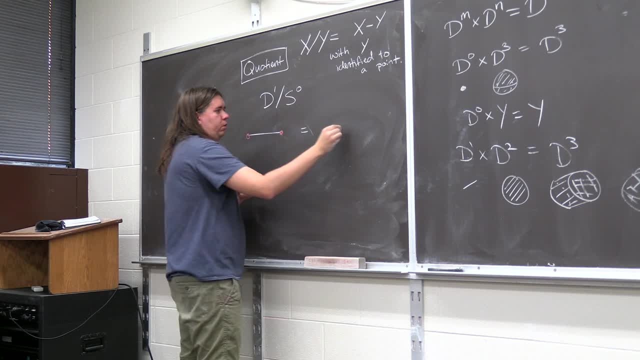 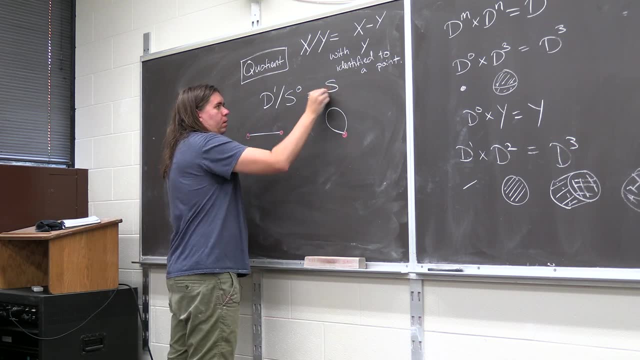 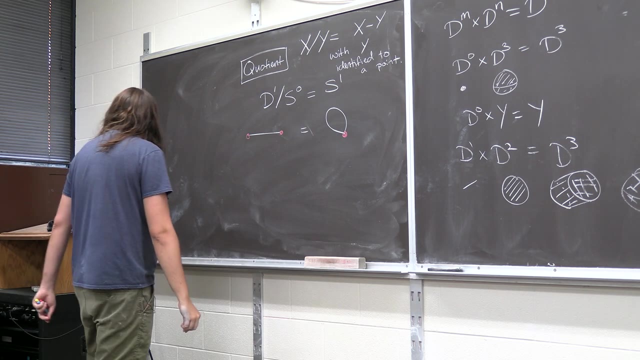 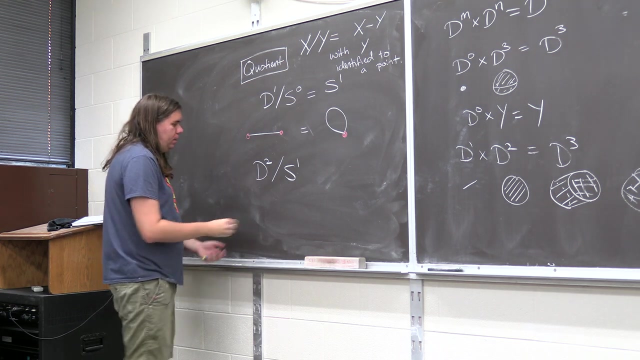 and what i end up with? those two points glued together to a single point. this is just a copy of s1, right? okay, more examples. if i want to do something like sure, if i want to do something like d2- quotient out by s1, my d2 is this disc. this s1 lives on the. 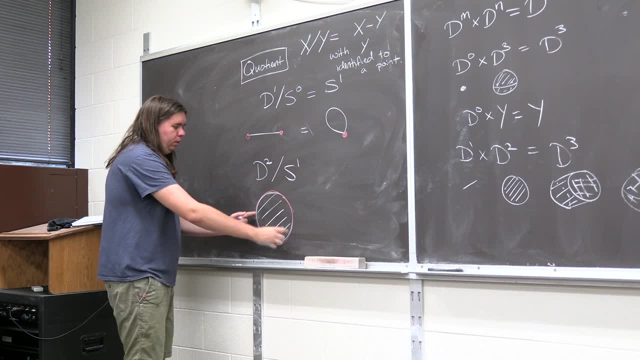 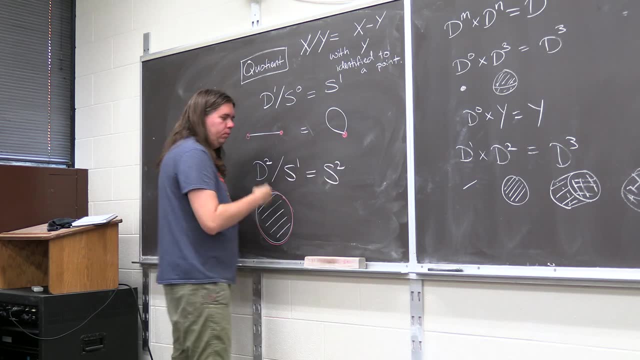 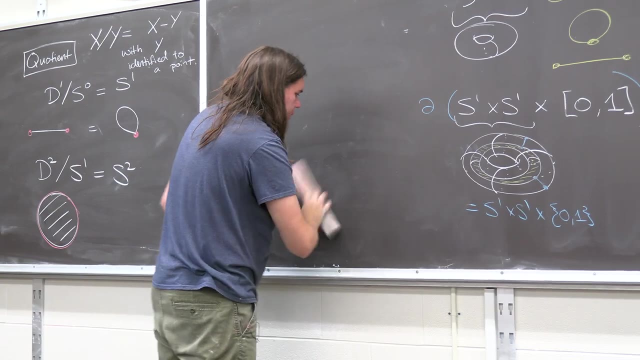 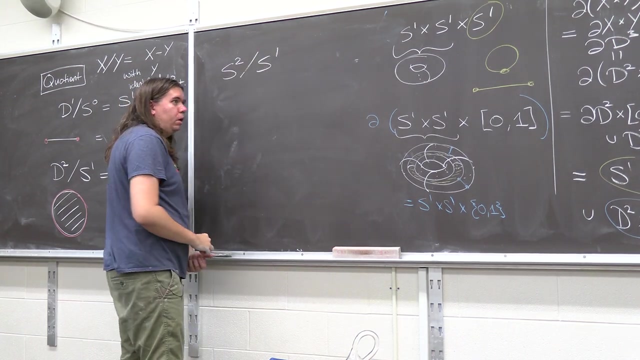 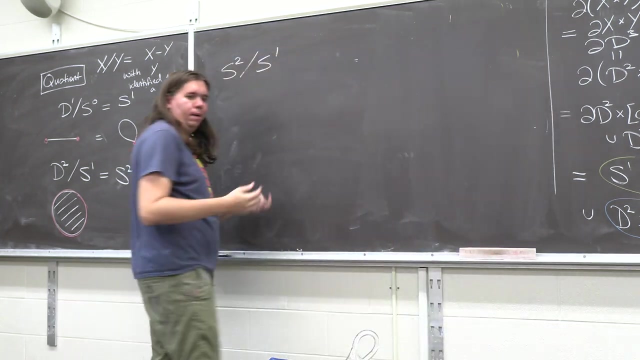 boundary. if i take all those points on the boundary and glue them together to a single point, what do i get? s2- we're getting the hang of this. what if i want to do something like s2 quotient out by s1? well, you know, you always have to ask which s1 you're talking about in s2, but a lot of times 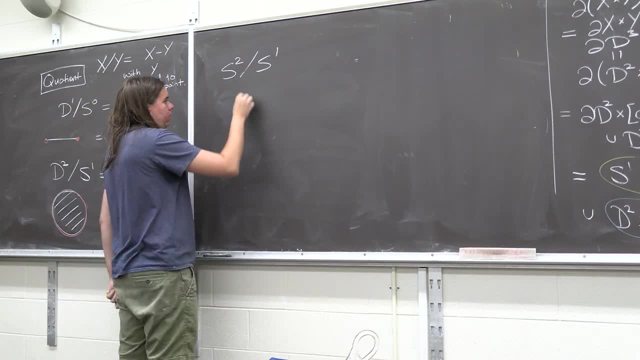 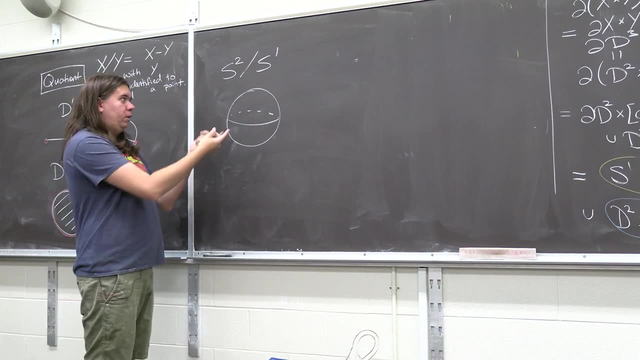 you know, it's pretty obvious what's in mind, and here doesn't really matter which one you pick, it ends up looking the same. here's my s2 quotient, out by s1, two right, and even in drawing s2 to make a three-dimensional, i'm forced to draw that s1. 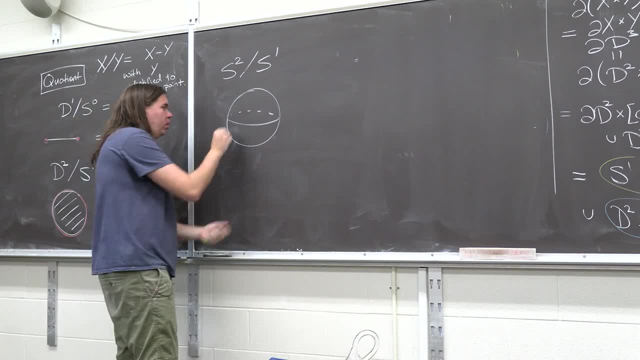 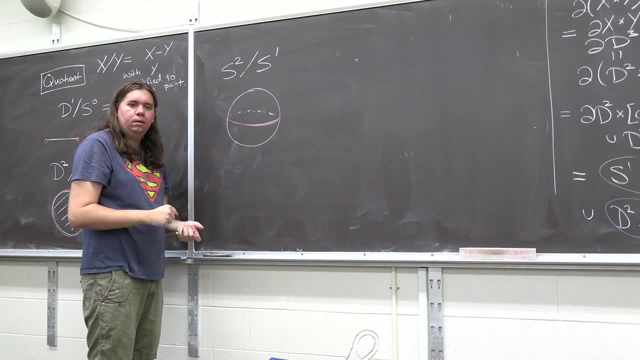 aren't i? so there's my s1 inside of s2, here's my s1. what happens if you grab that s1? you shrink it all to a single point. what do you end up with? what is it? yeah, it's two s2s, but they're like. 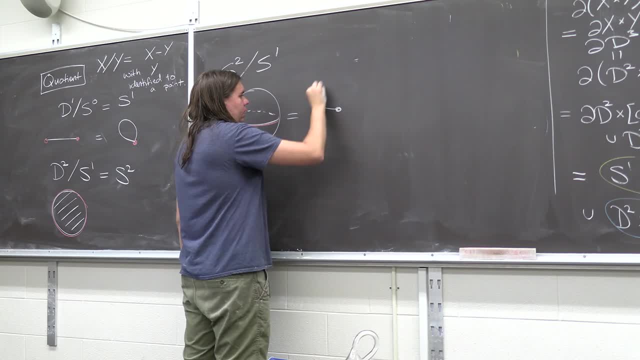 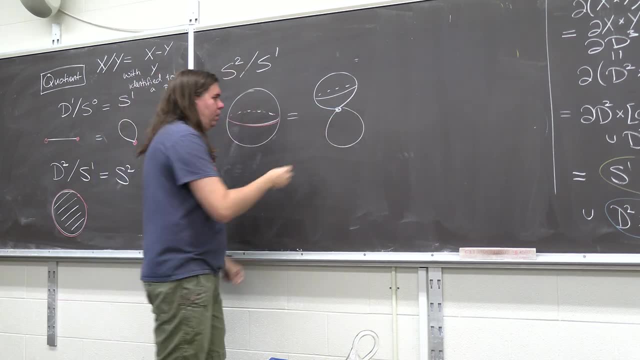 stuck together at a point. right, it's like you have this point here and you have an s2 on top. it's like you put a belt and you made it really tight until it gets shrunk down to a single point. okay, we have a name for this. when you have two spaces stuck together at a point. 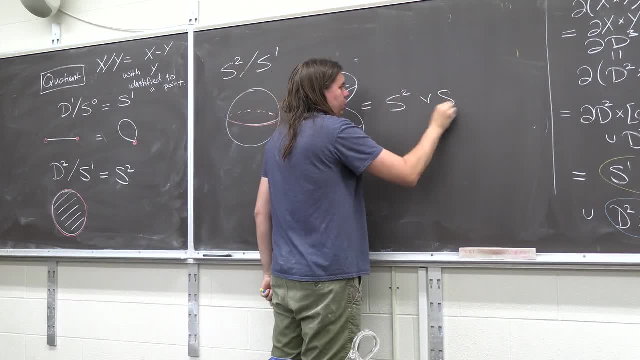 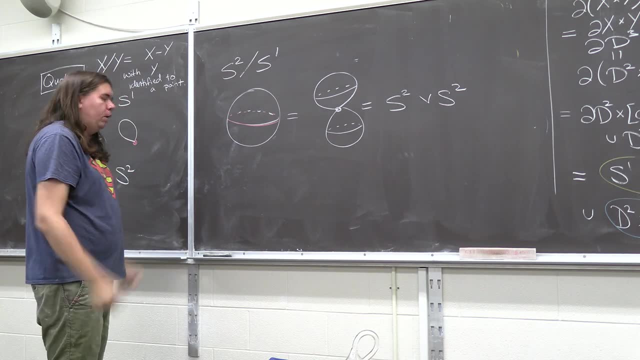 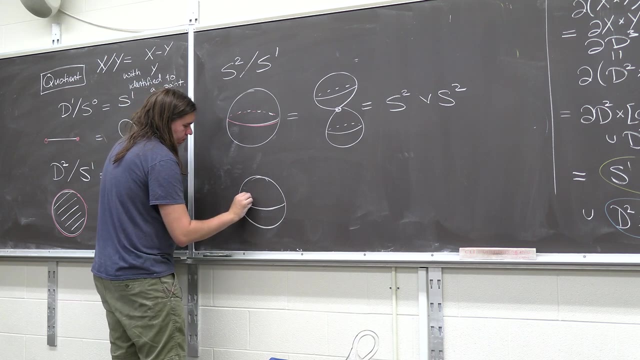 we just call that the wedge. this is s2 wedge, s2, where wedge is just sticking them together at a single point. okay, i'll do one last example. what i want to do is i want to take a sphere and i'm going to attach a line joining the point on top to the point on bottom. 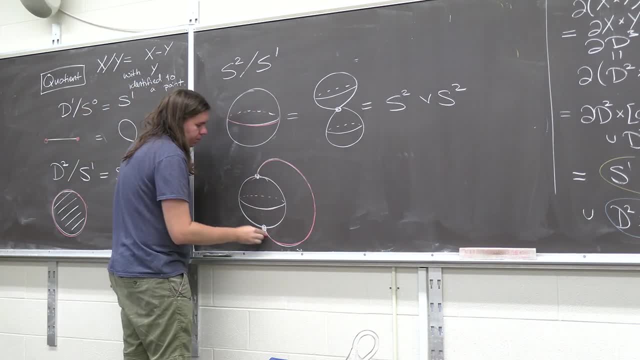 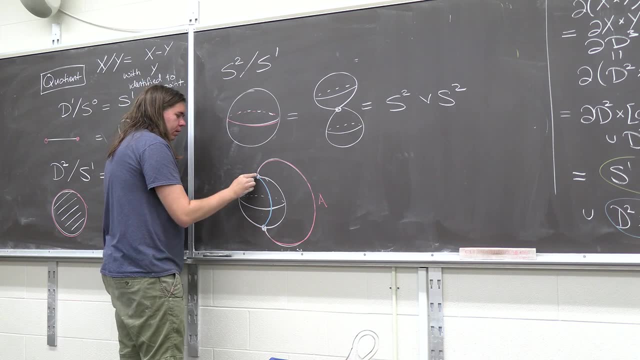 let's call this arc attaching the point on top to the point on bottom. let's call that arc a and let's call this arc attaching the point on top to the point on bottom. let's call that arc b and i'll call the overall space x. 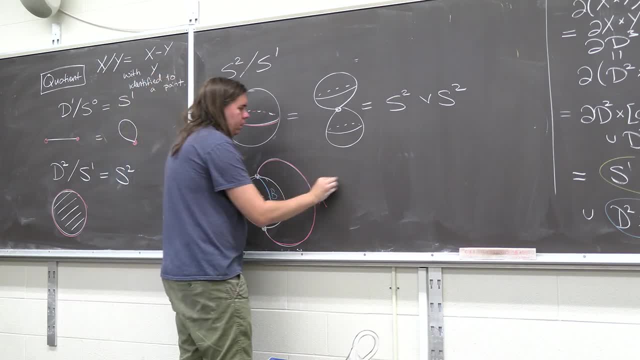 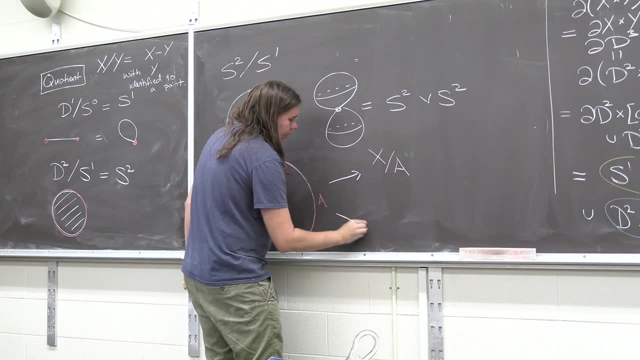 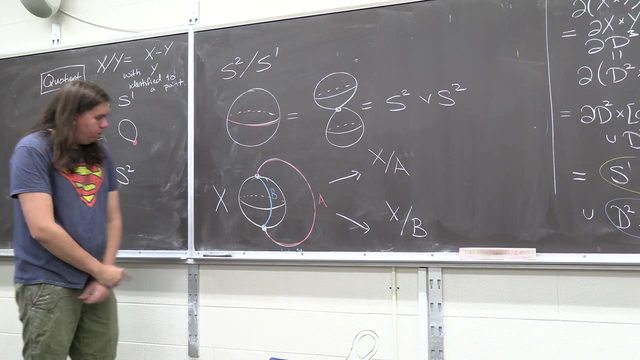 let's think about two things. first of all, can you tell me what is x quotient by a, and then can you tell me what is x quotient by b? so we're just practicing building up our intuition here. okay, what's going to happen if i quotient by a? that means i'm shrinking a to a single point. so what?